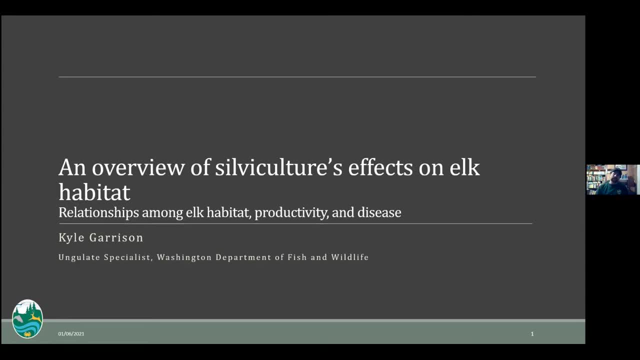 concepts, together with a bit of a case study on hoof disease and some of the things that we've learned from research we've done at the department on elk In Mount St Helens and how- I guess you know- habitat and nutrition tie into management. 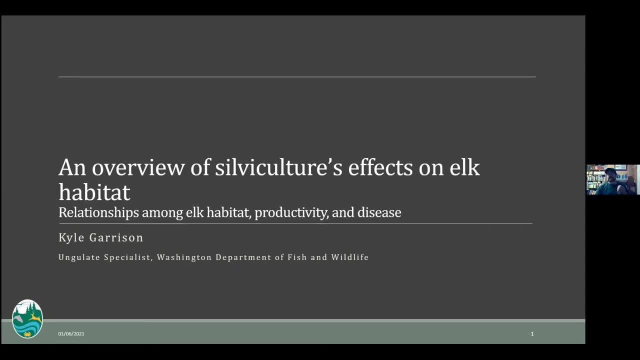 of elk and in this case may tie into the management of treponema-associated hoof disease, which I'll just refer to basically as hoof disease during this talk. So to go ahead and jump in here. it looks like my computer's maybe going a little slow. 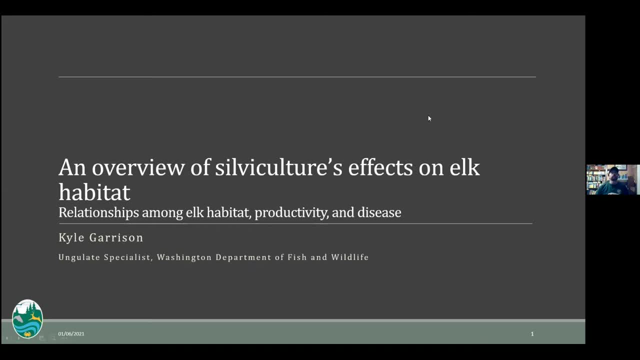 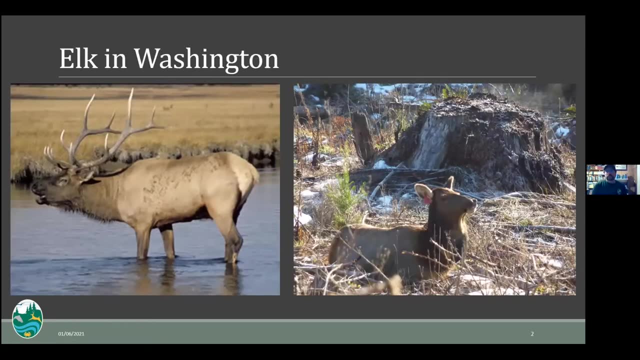 All right, there it is. There we go. So I think probably all of us are pretty well aware of what elk are and how they look, and in Washington we're really quite blessed to have two subspecies of elk in this state. 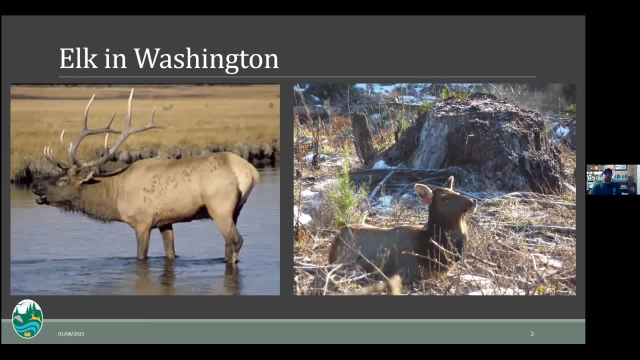 We have Roosevelt elk in southwestern Washington and the Olympic Peninsula and in other areas, herd areas of the state. we predominantly have Rocky Mountain elk and with some intermixing of those two subspecies where they meet, Elk Elk. That's something that we've done in our history. 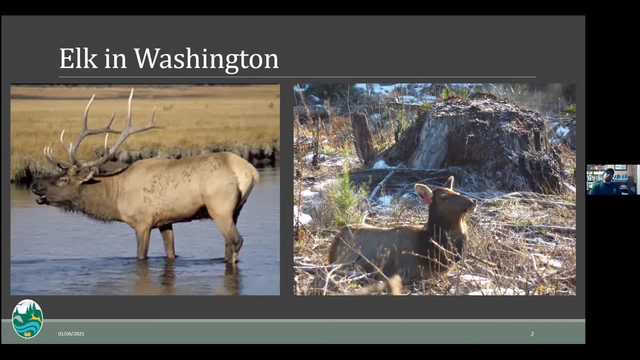 We're largely extirpated from all but the most rugged areas, essentially the Olympic Peninsula, But now we're sitting on a population of anywhere from maybe 45,, 55, to 60,000 animals statewide, depending on you know kind of what's going on that year that you know. 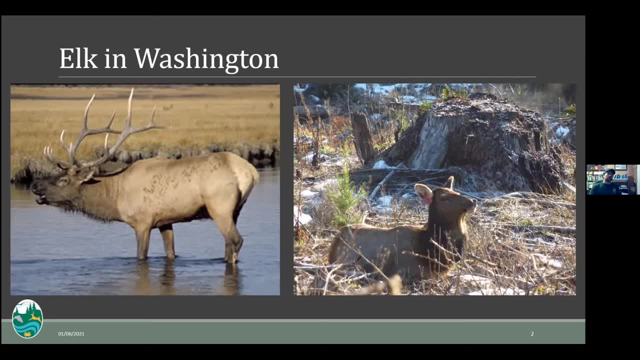 few years that we are able to do surveys. And of course you know, elk are really highly valued species for Washingtonians, Washingtonians and people across the West for their cultural, aesthetic and recreational value and also importantly, their economic value to the state. 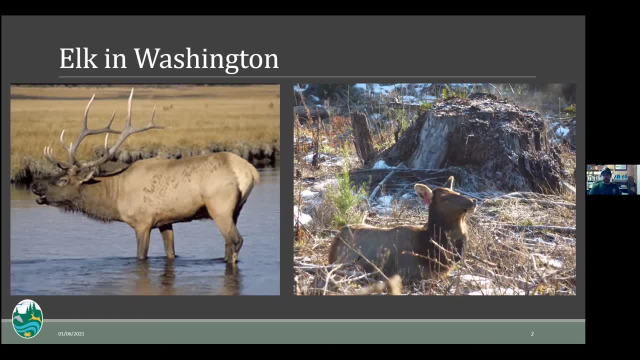 So understanding things about what limits elk or what might produce more elk and in general how to manage elk is fundamentally sort of an important task for us in the state as the Department of Fish and Wildlife. And of course you can't have elk without elk habitat, and habitat can be defined in. 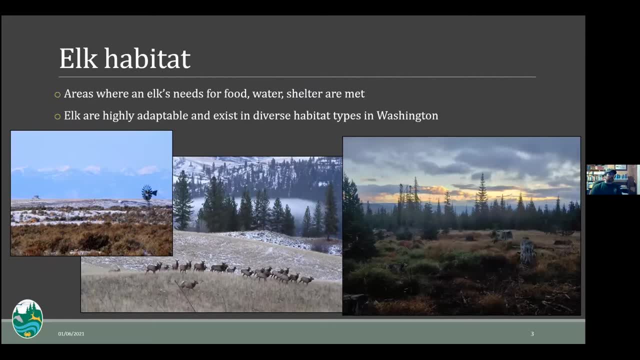 a lot of ways and can be looked at in very sophisticated ways, but essentially this is pretty common sense. It's an area where the needs for an elk are met through its nutritional needs. its food is there, it has water, obviously, and it has shelter, not unlike any other animal or 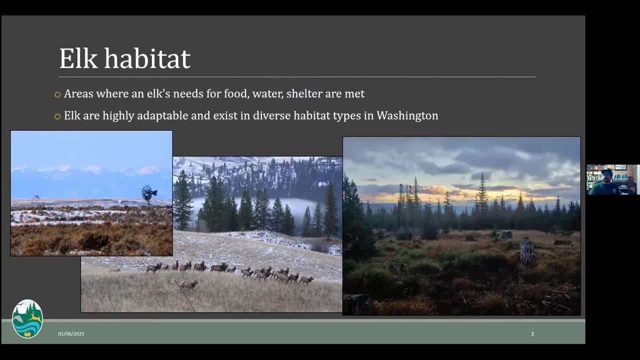 us really, And elk are really highly adaptable. Elk are an adaptable species that can exist in very diverse habitat types, not only in Washington, of course, but you can think of elk existing in arid areas and desert areas of the Southwest and all the way to the Olympic Peninsula, where we have record levels of 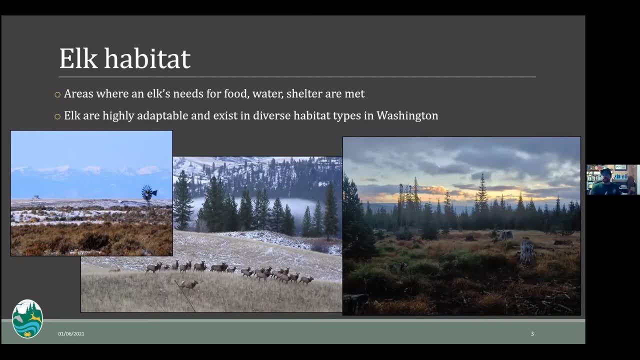 rainfall In Washington. you can see photos here of sort of some of the areas where we might even find elk that are very diverse. so you have sort of this sagebrush, steppe scab land almost in eastern Washington. There is a central and north-central Washington. 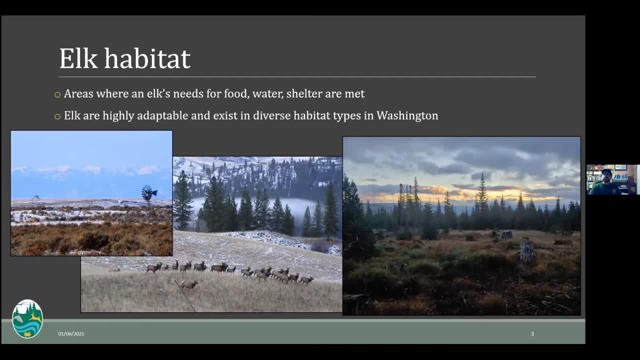 As a kid from Montana, when I think elk habitat, I think what we see in this sort of center photo of these grasslands: a bit of prairie with intermixed conifer stands, a drier landscape of what we might see in central Washington. 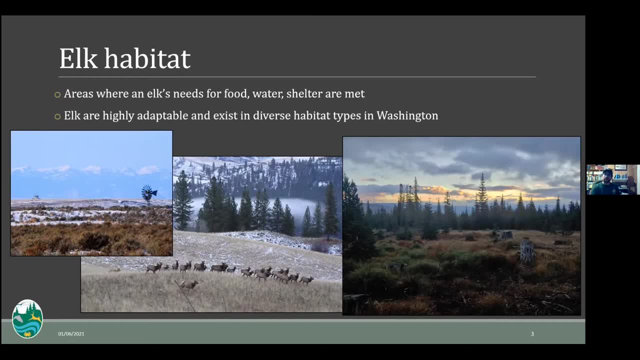 And then, of course, for those of us in western Washington I forgot to mention, I'm based out of Olympia, where we might think of elk habitat. out here We might think of elk. in Pierce County we might think of this sort of wet dug fir. 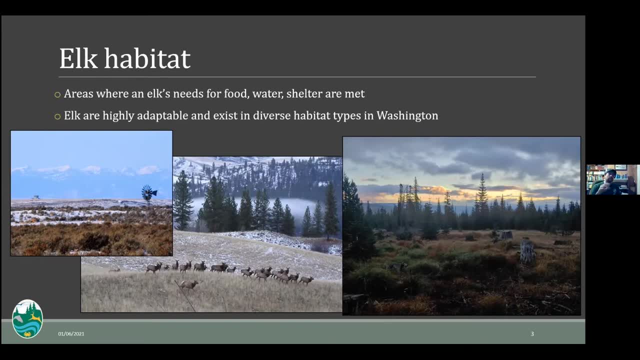 western hemlock stand with intermixed sort of meadows And today's talk again will mostly focus in on some of what we know about elk habitat in these sort of western West Slope Cascades habitats from research that's really been done over the last 20 or more years. 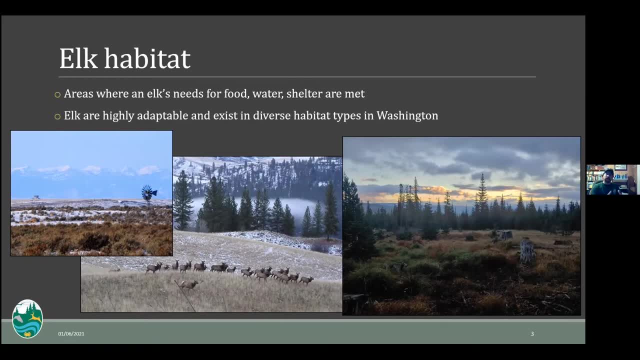 It's just a really great body of literature that I can only barely scan, I can barely skin the surface of, and of course also because of this tie-in with hoof disease and what we know about hoof disease and how habitat may be playing a role in the 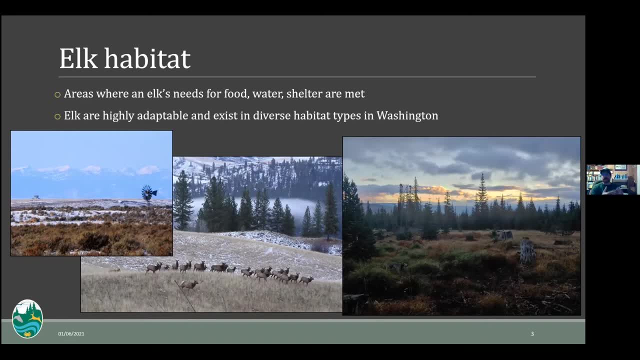 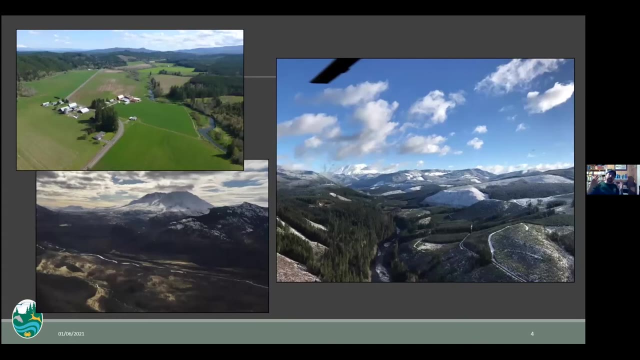 dynamics of that disease. So in western Washington. of course elk can exist in a large variety of habitats here as well, just in this sort of more narrow scale. In this upper left photo we have a very standard agriculturally-dominated lowland. 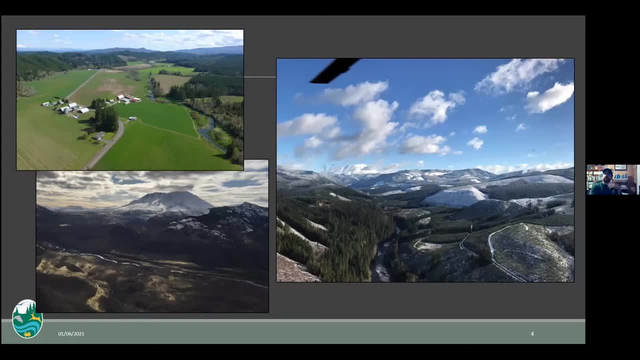 valley that's bookended by private industrial timberland or even public timberland. as you see, there We've got large tracts of federal or state land that's managed at varying levels of intensity. You see, maybe a representative example here on the bottom left of Mount St Helens and 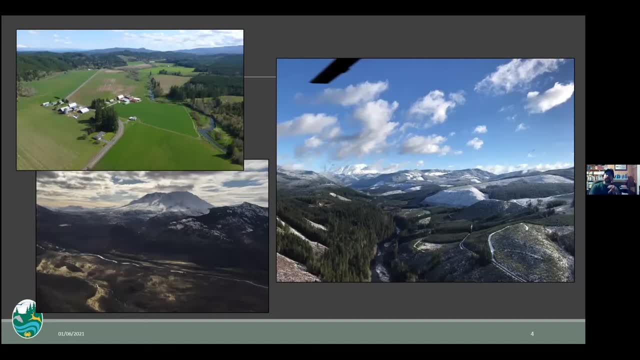 the National Monument, That tool room, That's where we've got a lot more river drainage. And then, of course, on the right here, where sort of what I often think of when I think of elk habitat in southwest Washington is this industrial timberland where you have 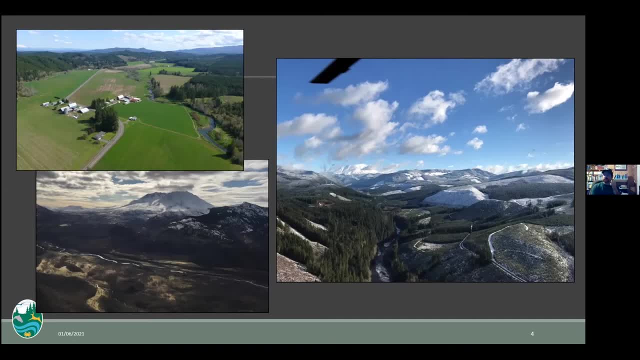 this mosaic of very intensively managed forest land and tracts of forest land, As you can kind of see in these photos when we think about elk habitat, well geez, I see a lot of green out there. I see a lot of green out there. 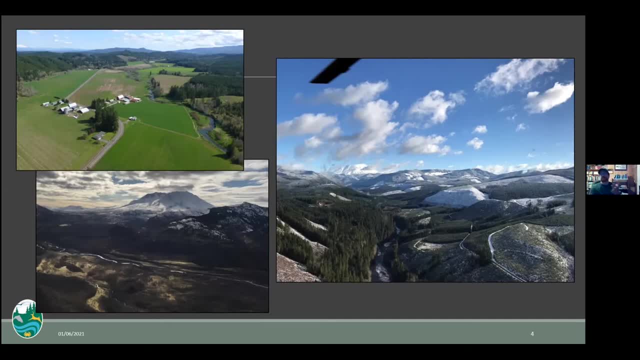 And green means plants and plants means food, because elk are herbivores And outside of that top left photo where there is quite a bit of green, that would be really, really great for elk and cause a lot of damage and consternation to those landowners. 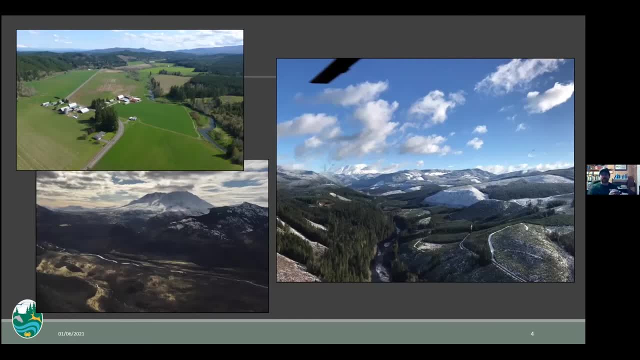 those producers, a lot of the other areas where we find, maybe, potential elk habitat. the vegetation that exists is really not all that great for elk. You know. Well, we have unlimited green. You know, I remember once I went to Alaska and I was like, oh geez, there's green everywhere. 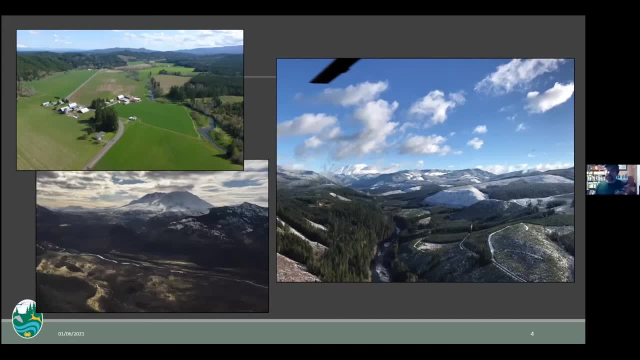 Why aren't there animals just absolutely everywhere And when I was at high school? the reason why is that not all plants, not all forage items are created equal in their palatability and their nutritional value for elk, And I apologize if a lot of this may come across as common sense to folks, but I want 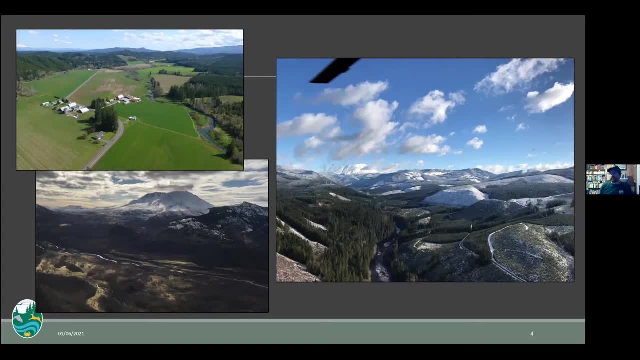 to make sure we're kind of all on the same page here. So plants, So plants that are really common in a lot of these areas: Western Washington things like you know, of course, conifers and ferns and Oregon grape, you know, these are pretty. 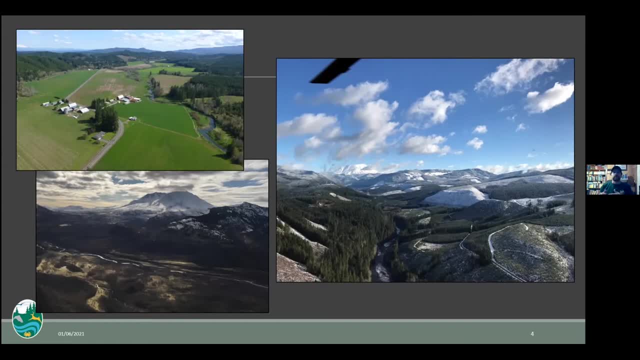 low value for elk And rather elk would much rather prefer to consume, you know, nice green grasses- post-winter green up, and the forbs that come along soon thereafter and the shrubs that are available seasonally. Those are really highly nutritious, easily digestible plants. 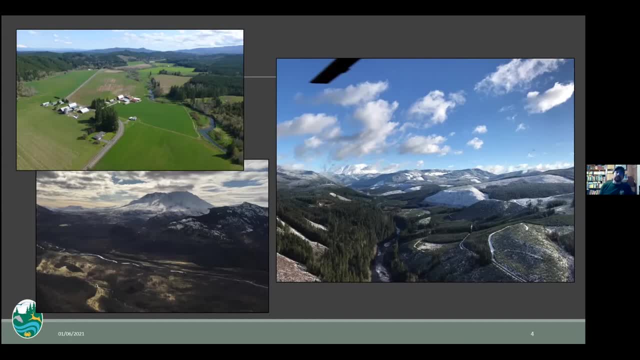 Yeah, And I think that's a good point, And I think that's a good point, And I think that's a really good point. I think that's a good point. I think that's a good point. You know, these are broad brushstrokes. every species is a little bit different. 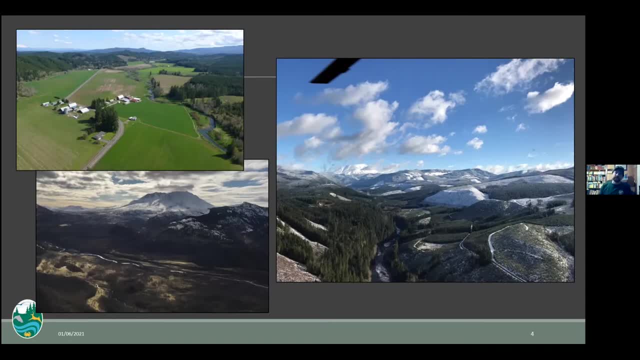 We don't have the time to maybe get down into those weeds. but that's just to say that there's sort of considerable plasticity in the diet of elk and in what they might prefer, and that isn't always represented in some of these areas in Washington. 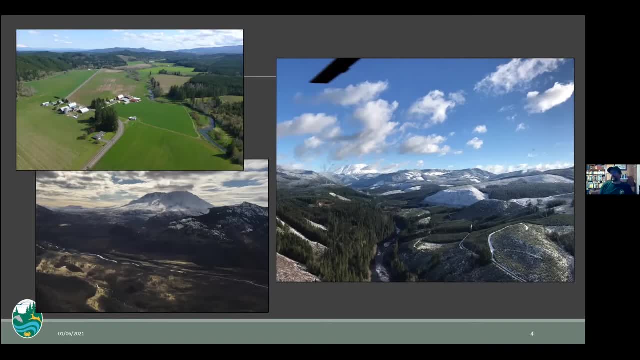 And that kind of explains some of those broader meta-scale dynamics of you know why elk are doing well in one area and they're not doing well in the other areas, So where we find these highly valuable forage items? you know that the grasses and the 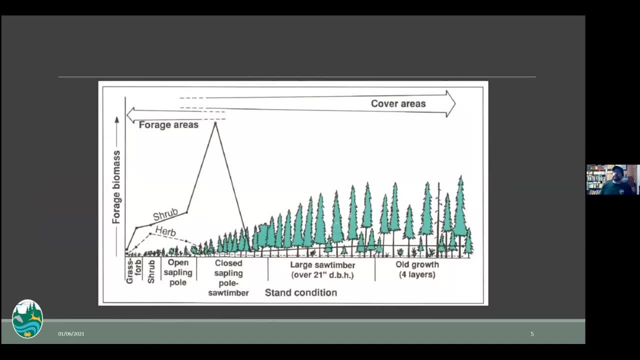 shrubs and the forbs. are these what are called early cereal stages? And of course I'm talking to a group of foresters. I always- I kind of hope I don't sound super foolish- to speak forestry to actual foresters. I'll just pretend to be a forester at this. 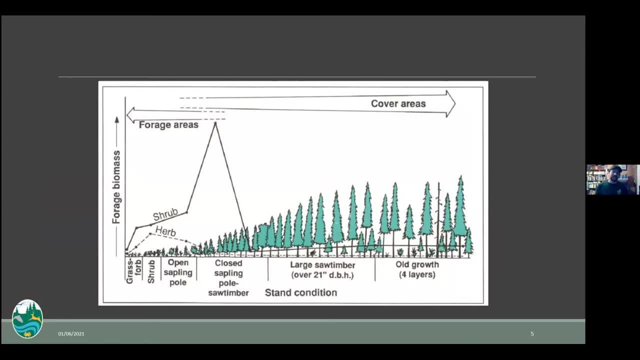 moment. But this figure I really like. Yeah, It kind of shows us what we're dealing with where in the early period of a cereal, very early cereal periods of a timber stand really those first 10 to 15 years post-disturbance. 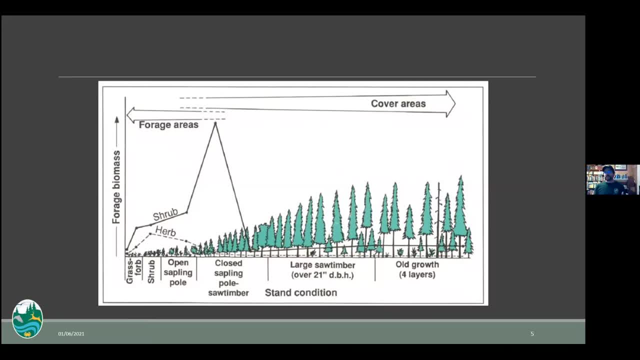 where we see a lot of sun, solar radiation, a lot of sunlight hitting the ground, It allows for those palatable species to grow and become more abundant. Those are really good areas for elk For their foraging, But of course it's not the only thing. 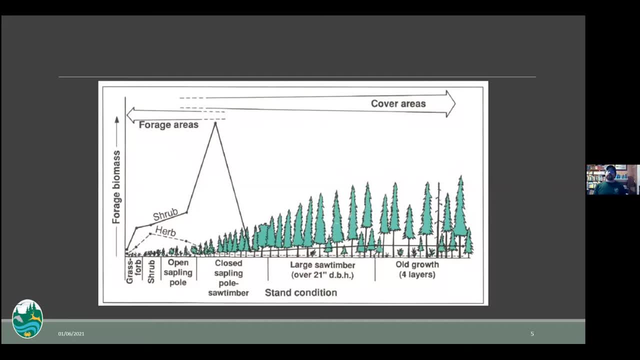 And this figure kind of shows you is there's there's foraging areas and then there's cover areas, And I think that's an important concept where it's not just about food, of course, although you know, the idea of cover might sometimes be a little bit exaggerated and it kind of 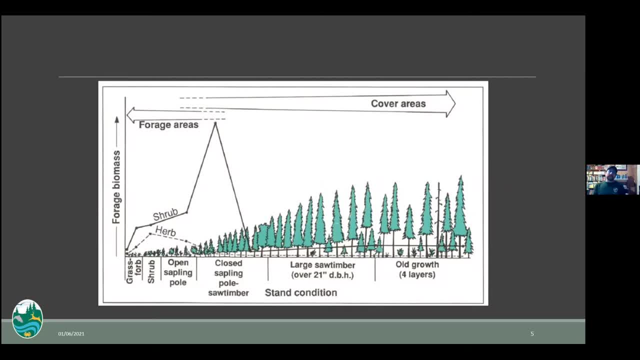 it's sort of context dependent. you know, elk don't necessarily need it for thermal cover as much as I might need it for security cover to evade hunters or predators of some kind. So these early successional stands are really great for forage and as the stand grows older, 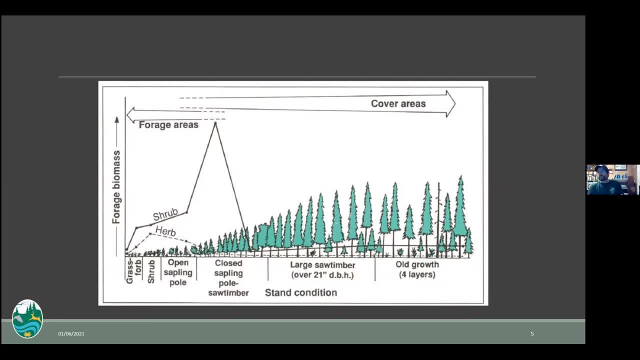 after that 15 year period or so begins to close and there's just less forage available in there. And those early cereal stands, of course, historically created by things like natural disturbance. you know these are massive windstorms or fires that happened more intermittently. 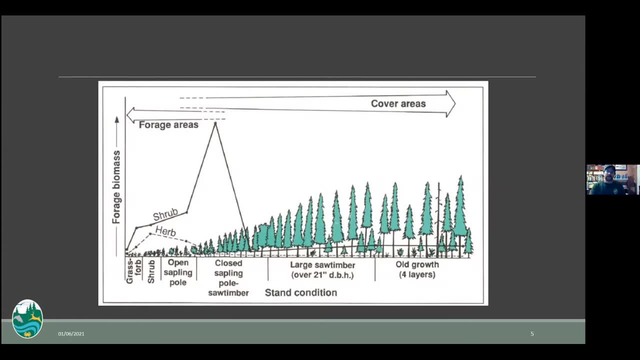 than we see them now, Or and perhaps I think you know kind of the most dramatic fashion and I can think of naturally occurring, is a volcanic eruption like we saw at Mount St Helens that really created a tremendous amount of early cereal, early cereal stands. 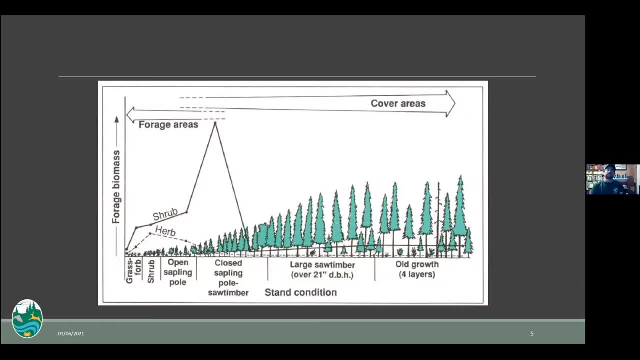 Today, of course, and for quite some time, timber harvest and its associated management and practices, silvicultural practices are what have been creating the majority of these early cereal stands And, of course, consequently, the forest practices, and forest management has really important. 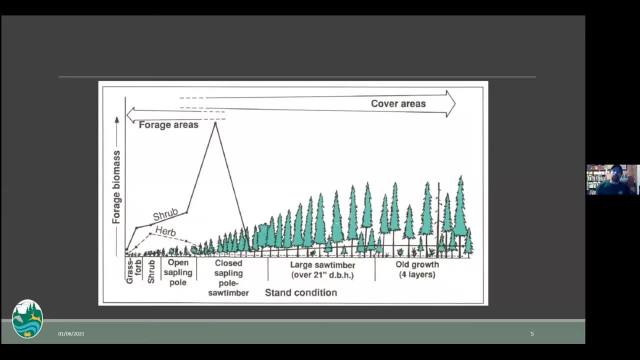 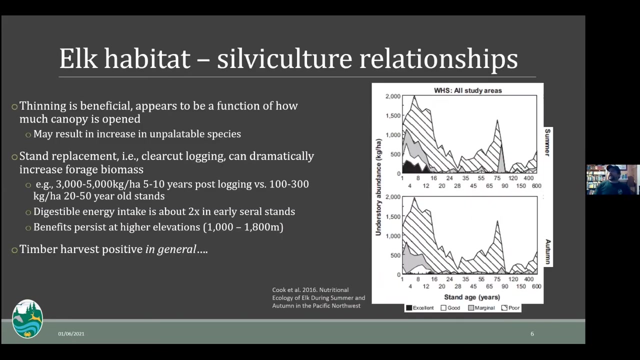 and not necessarily altogether straightforward- influences on elk habitat and ultimately that habitat is determining kind of the population dynamics of the elk population. So you know, kind of highlighting a little bit of what these relations are, What these relationships might look like here, and I've got to move this all your pretty. 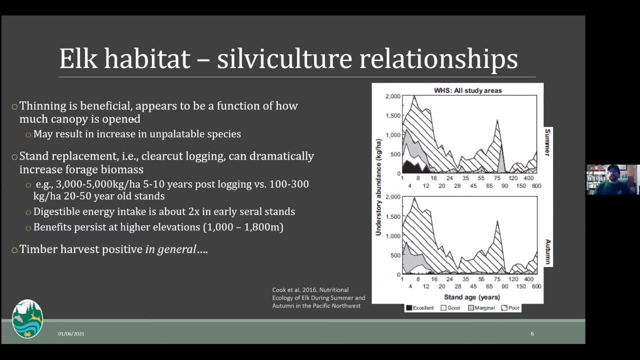 faces over out of the way. so I can kind of explain this figure, because it takes a little bit of doing So. first sort of try to ignore this busy page for a little bit. and I'll just say you know that finning- not to dismiss finning as an important silvicultural practice, and it's 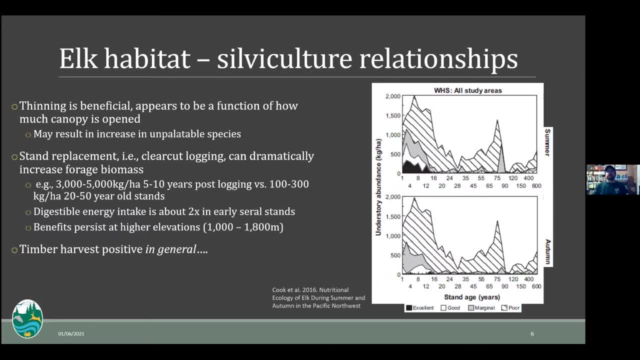 got value for creating those conditions. It's got value for creating those conditions where solar radiation reaches the ground and it grows grass, forbs et cetera. that it is good and it is valuable. I know less about it sort of direct impacts. there's a little bit less, it's not quite. 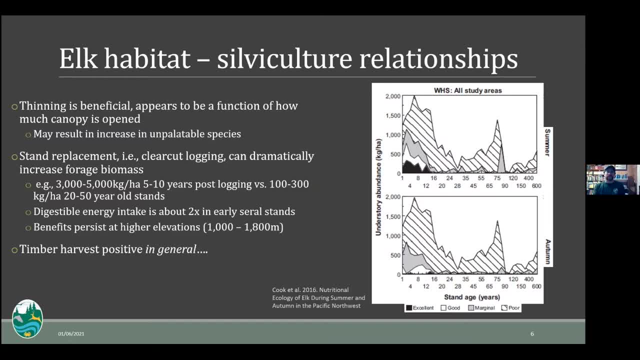 as you know- pardon the sort of pun, clear cut- and it's really kind of just this function of how much do you open in the canopy. And one of the interesting things there is that if you, if you're not opening the canopy a lot and you're not creating a lot of ground level disturbance, you may actually inadvertently 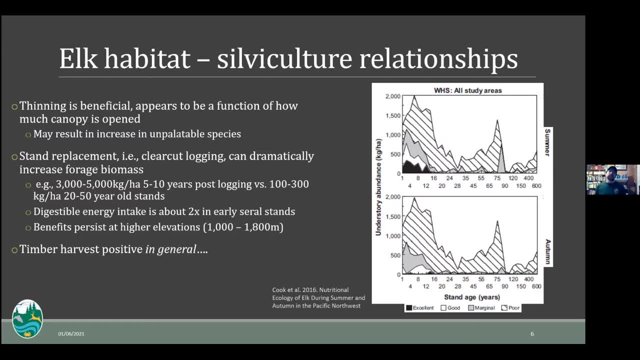 inadvertently encourage the growth of those unpalatable species that they're shade tolerant they do all right in the understory. when there's canopy cover and then you open it up and you give them more solar radiation, they might actually kind of go gangbusters in there and 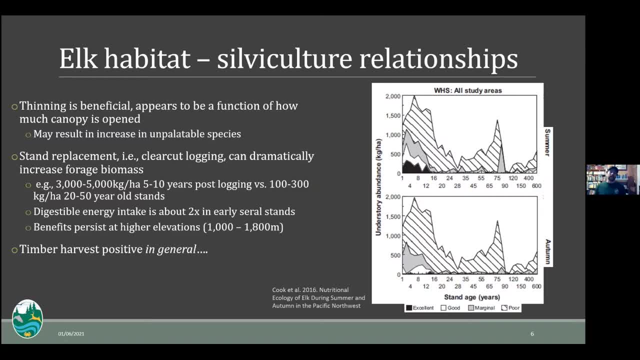 out compete some of those more palatable species for elk, As opposed to say stand replacement or clear cut logging, which really dramatically increases forage biomass. you know, and again I'm painting broad brushstrokes Here, but that's a pretty, you know, pretty solid rule. 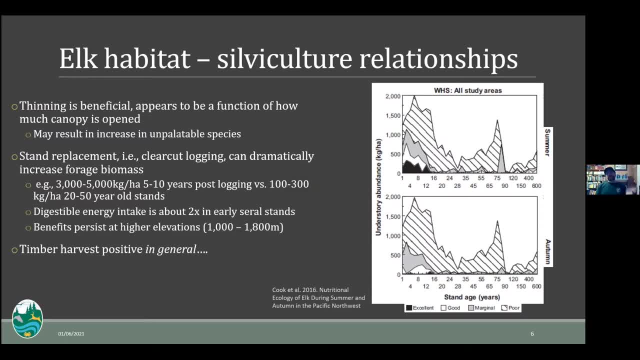 You say you cut down, you know a 20 acre stand of timber. you open it up to sunlight. A lot, of, a lot of good plant species are going to regenerate in that early stage and that's going to. those are going to be of high value for elk. 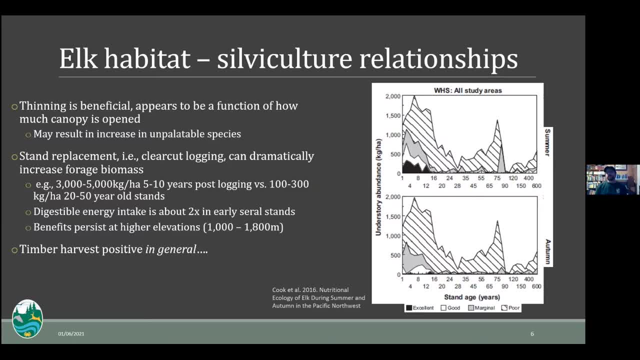 That's a pretty low risk thing for me to say, And one of the ways to sort of illustrate this is: now we can kind of look at this figure on the right and I'll give this sort of example here from some of the work that John or Rachel. 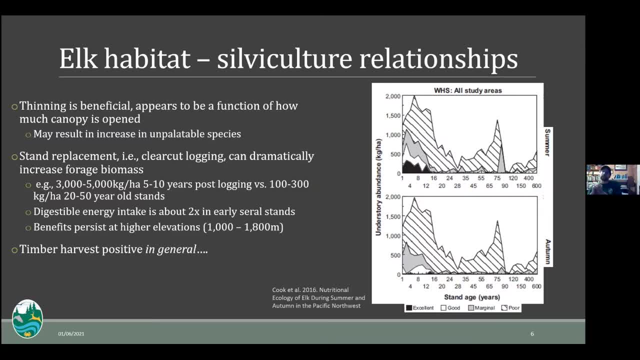 and others have done. These are: these are folks that are kind of paragons of elk nutrition and understanding elk nutrition and how it ties into these population level effects. They showed in this paper that in these early stands, these five to 10 years post logging 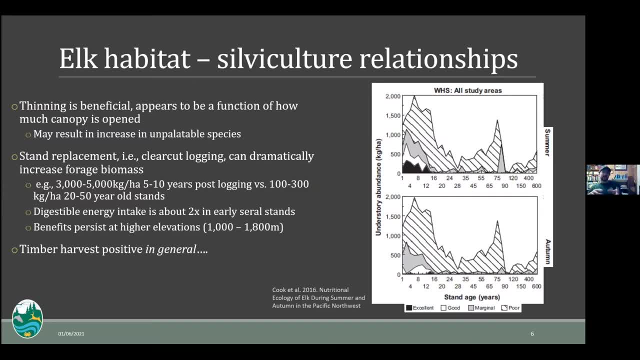 three to 5000 kilograms a hectare of biomass, versus 100 to 300 kilograms in 20 to 50 year old stands, And that's just kind of showing and really driving home this idea that a stand grows older and the canopy closes. 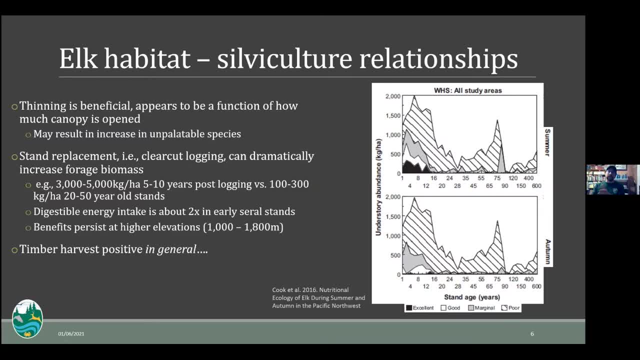 That's a window where the forage value is really diminishing. for elk It's not invaluable. It can be very important that security covers not to be dismissed, but it doesn't. it won't have a lot of forage value. And so what this figure here on the right is showing us? 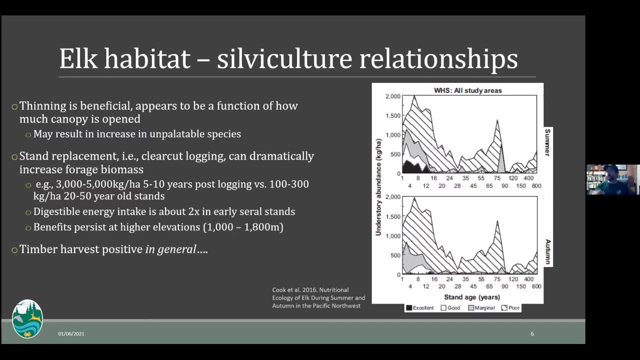 So the top is summer biomass in the understory and the bottom is autumn fall biomass And the understory of forage plants for elk And the x axis. here is time in years going across. It's got kind of the staggered way of looking at it. 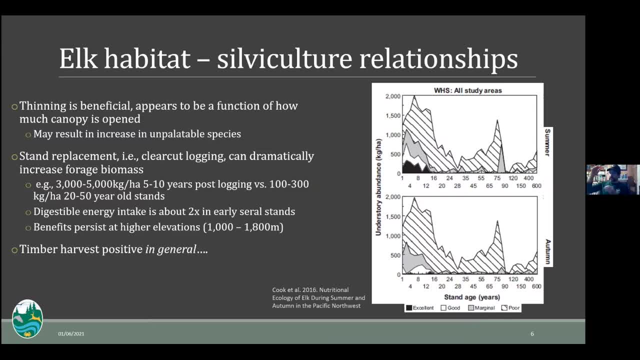 So you know, just you know it's sort of 15 years is kind of 25%, maybe maybe 20 years, about 25% of that x axis. And you can see, there we have black, white, gray and sort of dashed and those represent 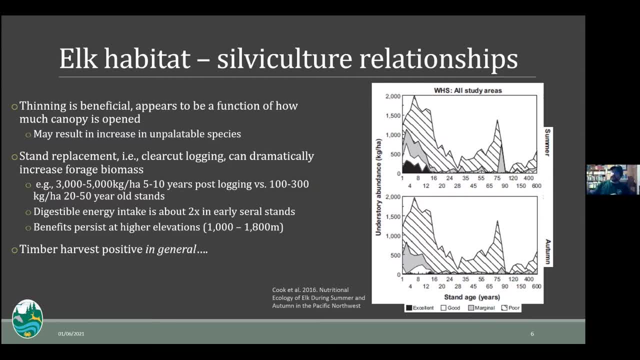 excellent, good, marginal and poor Sort of density plots of biomass there. So what you can see is in for summer nutrition or summer forage availability on this top panel, the first you know one. there's this massive dip in that data set, but you know. 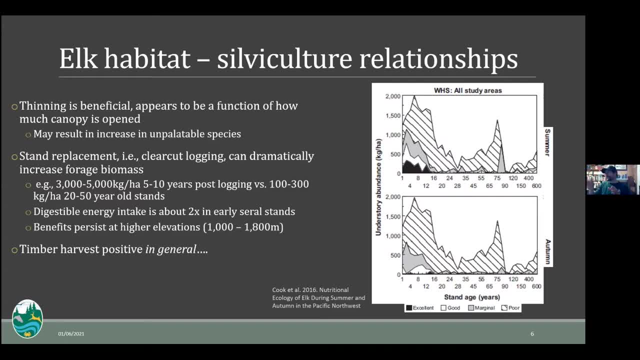 one to 15 years or so. that's where we see the excellent forage biomass. When we look at the, at the good, you know same general pattern, marginal, same general pattern. and the poor, you know we've got a lot of forage. 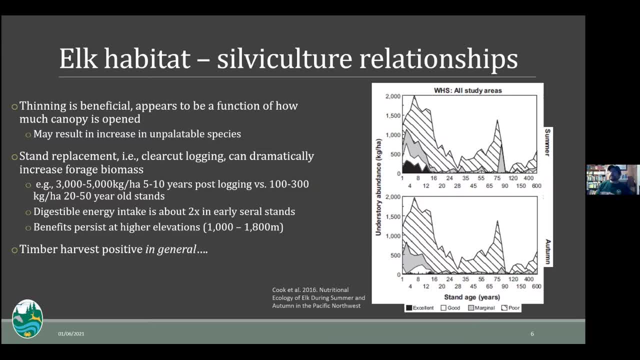 Yeah, Poor biomass and poor meaning unpalatable or a poor nutritional value to elk. you know that that just exists out there and sort of superfluously. then you see, in autumn, you know, our, our forage is starting to senesce. we're getting into, you know, out of the 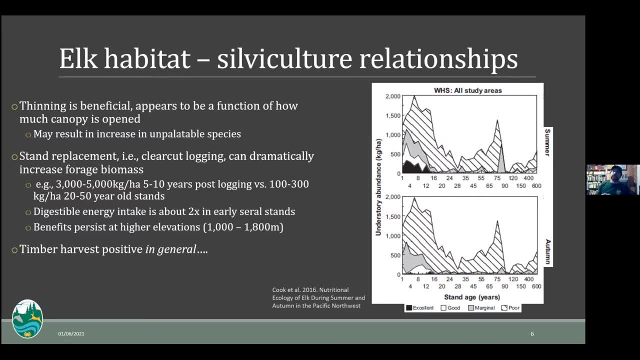 the really productive seasons. So a lot less of that excellent biomass. got some good biomass and and and you know, getting pretty pretty standard with that, With the marginal, And then a lot of them. you know, the poor biomass is just sort of out there and just 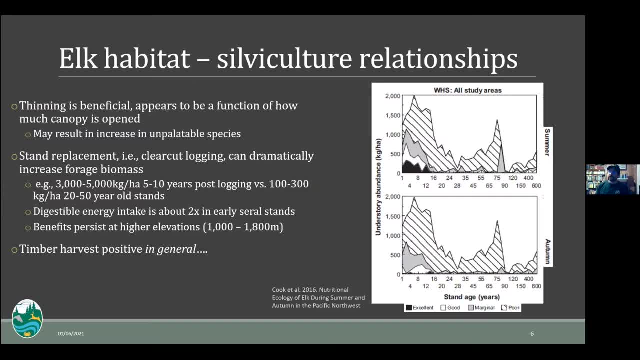 represents quite a bit of what's in the understory, kind of regardless of of time, And so this you know, as a sort of a side note, this also highlights one of the one of the unique things about what the cooks and many other folks have been working on. 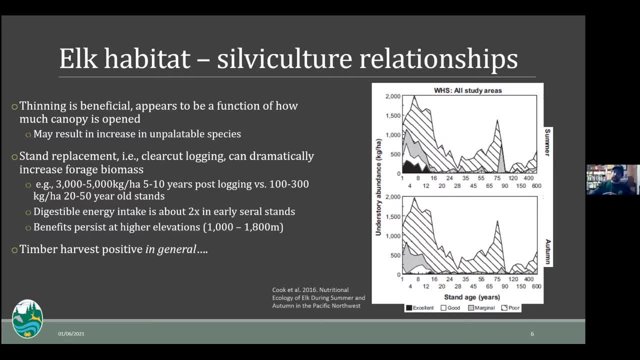 and researching a while is that for a long time, when it came to elk and other ungulates, we were really focused in on winter and winter is this really important driver- And winter nutrition and you know, is there enough food out there in the winter for them? 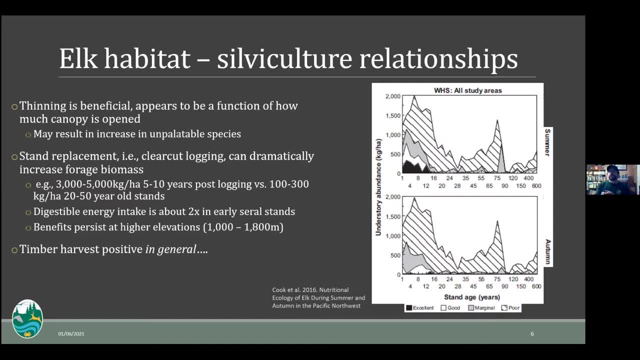 to get through. But what we're actually learning is that summer nutrition is playing a really outsized role in the dynamics of of elk and how well they're able to perform. meaning, you know, are they able to, to, to conceive, are they able to, you know, recruit a calf? are they able to? 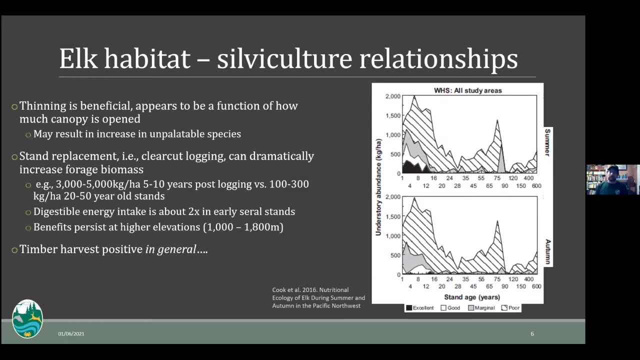 be, you know, are they in good enough condition that they can, you know, be lactators, for instance, So that summer nutrition is playing a big role? Yeah, Not an animal is able to accrue enough body fat to make it through winter. 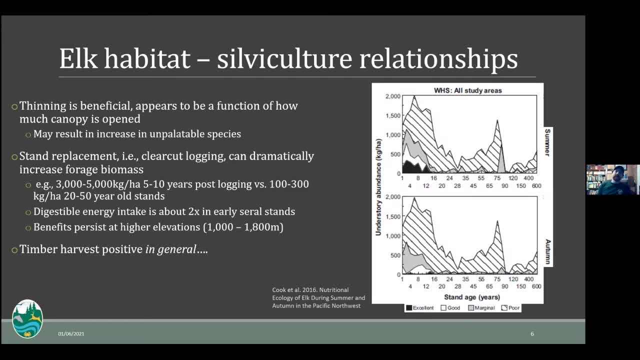 That's a. that's a pretty important component there, And I'll talk more about nutrition and actual body fat levels and things here in a few slides. So kind of take this back um. the digestible energy intake is about two times that in early. 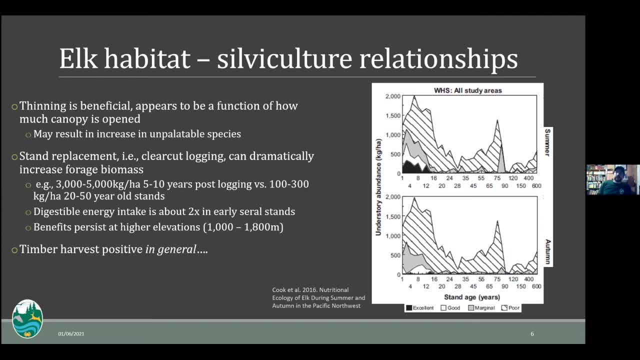 stands as it is in older age stands for those 10 to 15 years, it's, you know, about twice as good, uh, in terms of what's out there for elk to eat as a general. So that's sort of a rule of thumb and it- and it's important- sort of uh, um, that digestible. 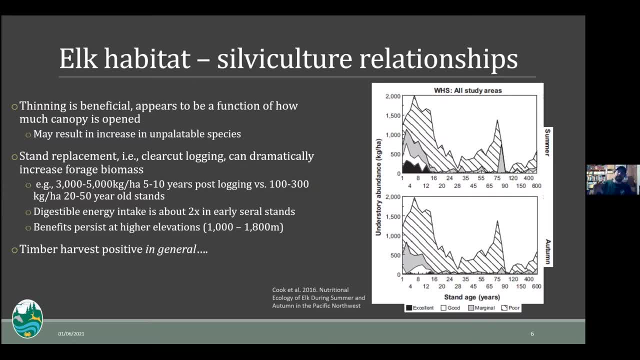 energy part is is sort of an important uh uh determination there, where again there's a lot of species, plant species- out there that you know are available to elk but they might not be all that good for elk. 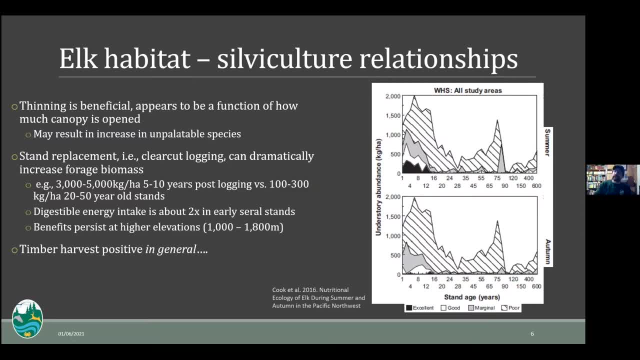 Um, they might be unpalatable or they actually might be kind of costly for an elk to consume. you know, maybe they can break it down. There are large bodied ruminants so they're a little bit better at being able to break. 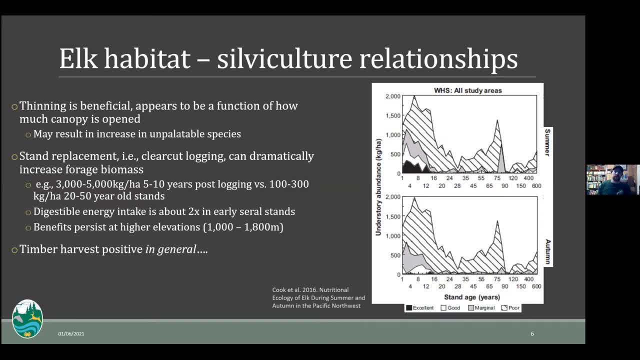 down low Digestible components of plants. but, um, there's a limit to that, And so there's a sort of trade off between efficiency and- and I'm digressing a little bit there, but nonetheless- these early stands again. uh, good for elk. 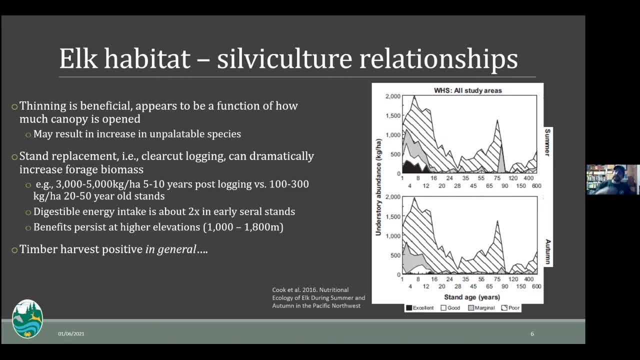 And then um. this study in particular looked at, uh, you know, both low elevation and higher elevation stands And one of the kind of. I think the interesting component here is that it the effects, uh, the benefits of um stand replacement. 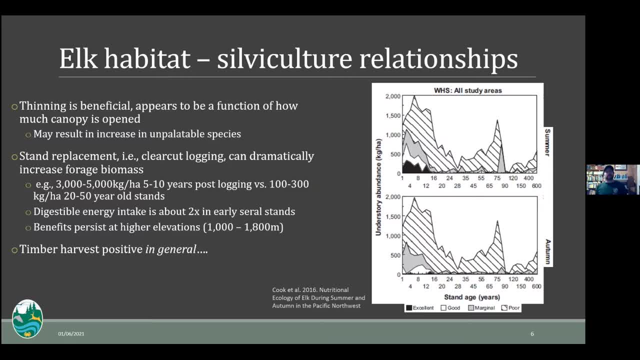 Uh, I'll put that log in here. persist a little bit longer in higher elevation stands than they do in the lower elevation stands, So uh, kind of bottom line. you know underscore that. you know timber harvest, uh stand. 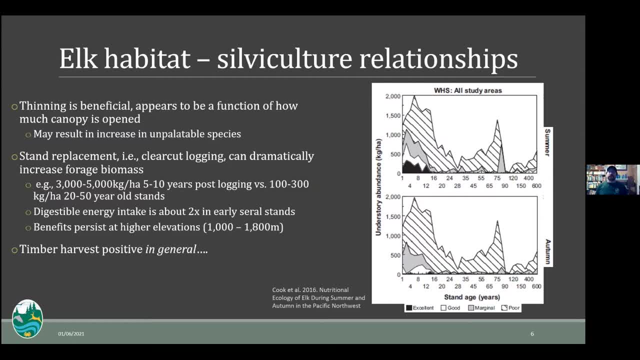 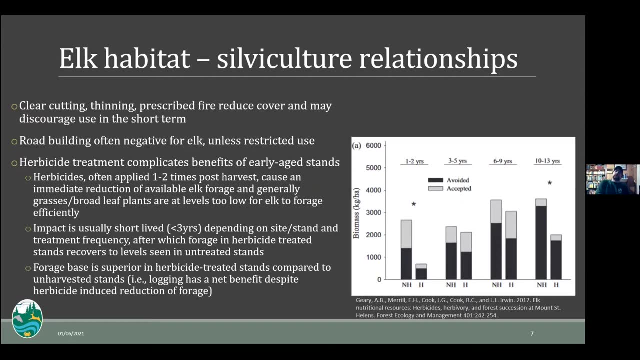 replacement, you know is is is good for elk habitat and good for elk nutrition. uh, in general, Of course there's there's. you know, there's always trade offs with everything in life And, um, One of the one of the trade offs here is that, you know, clear, cutting stand replacement. 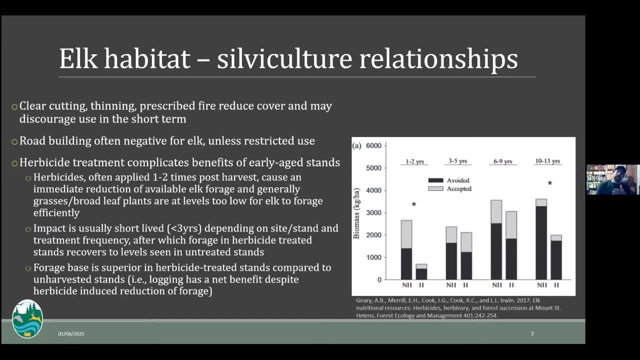 thinning prescribed fire, all these things we might do to a forest stand, uh, may discourage the use of that, of that area, of that stand by elk in the short term. Uh, you know, depending on on how extensive that disturbance was, it's it, it might be. 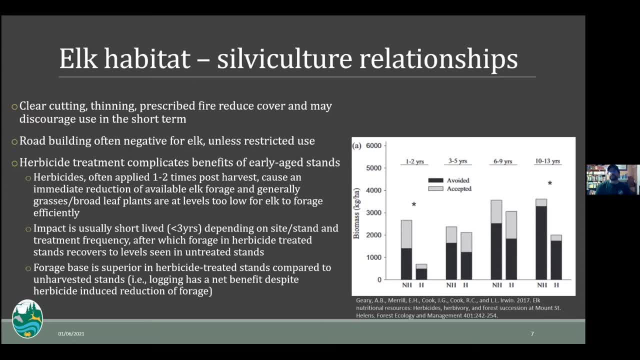 very short lived that avoidance, or it might be quite a bit longer um road building. If you know, civil cultural practices And and forest practices are are producing roads that are then being used and traveled after the fact and and sort of uh are allowed to have um uh sort of open access. 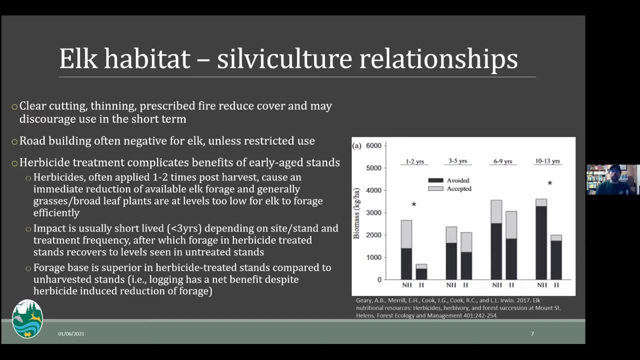 That's a bad thing for elk And, in fact, you could- you, you might actually, you know- negate any, any real benefit, um, in terms of elk use of an area, If you create a lot of good habitat. 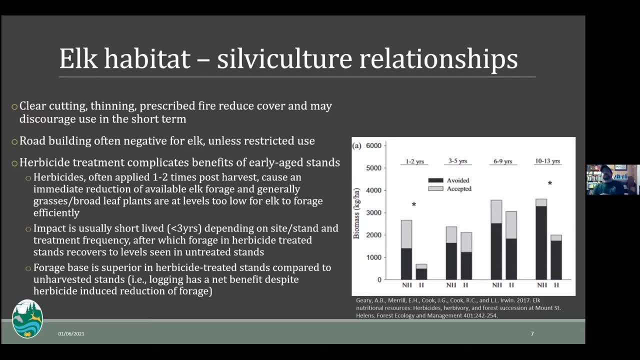 And good forage if you've got a road right next to it. you know elk really don't like that. They don't like that road disturbance. If it's a closed road, restricted use, you know you're probably not dealing with the. 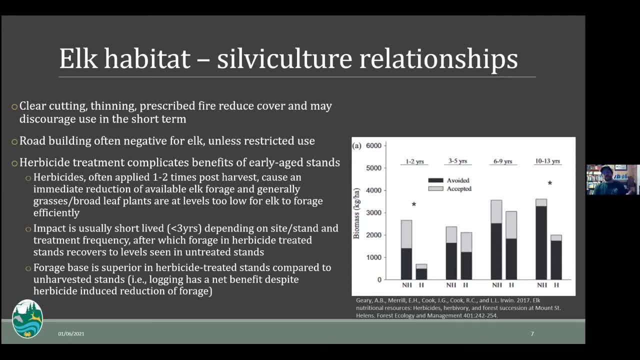 road itself, I guess, is what I'm getting at. The road itself is not necessarily the problem. that might result in elk avoidance, um, but that traffic on that road, and that's vehicular, that's dirt bikes, that's you know just. 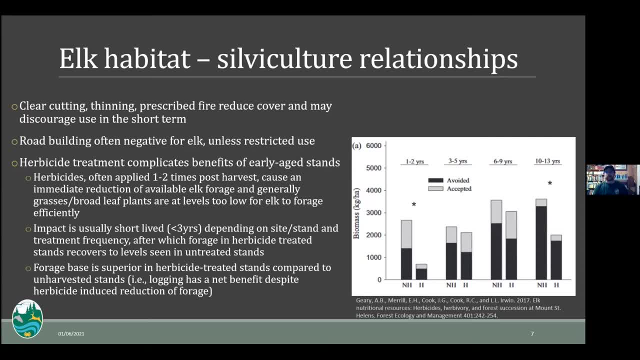 people walking uh sometimes can be enough to sort of discourage the use of an area by elk- Another one that I think is is really interesting and something that uh is often kind of brought up and talked about- and and of course we, um, you know, I, I, I won't be surprised if 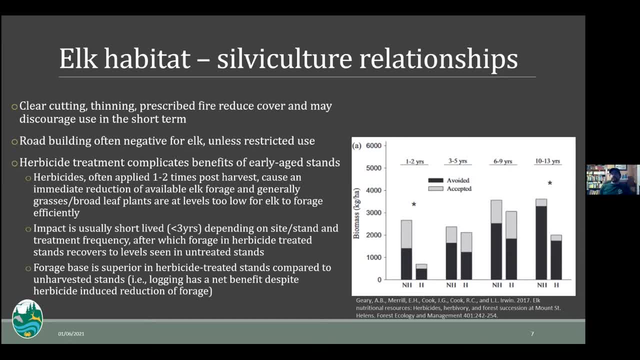 this audience. um has sort of forest herbicides and things like that on their mind quite a bit, And I'm sure that you folks know quite a bit more about it than I do. but one of the interesting questions is: okay, well, stand replacement is is good for elk in general, but what about? 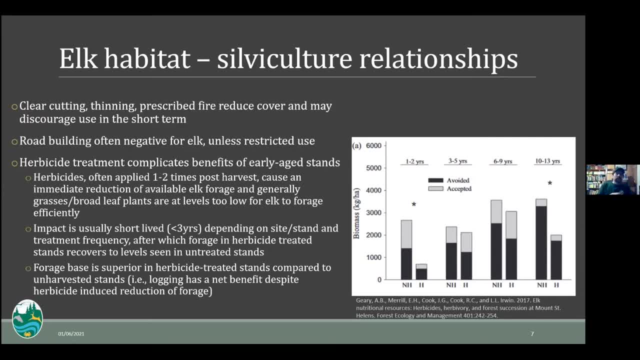 these associated practices Like Um herbicides. you know that that help, um, you know folks grow their conifers and and do their business, but it's actually actively sort of reducing the plants that are available for elk. 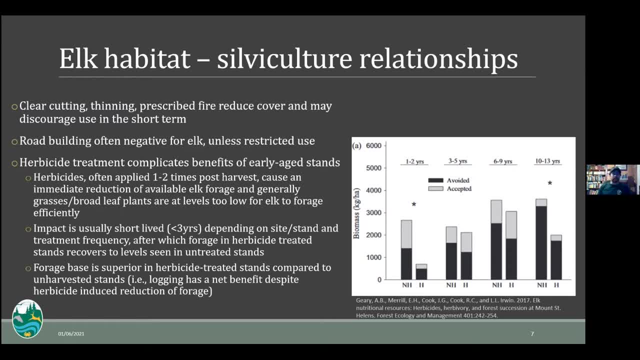 Um, and so some folks out of um University of Alberta, um, uh, Andrew Geary, under the guidance of uh Evelyn Merrill, along with uh some folks- John and Rachel Cook and Larry Irwin- Got together. 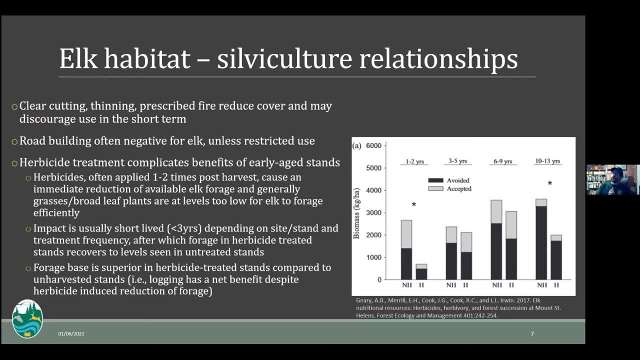 And they, they did, uh, um, quite some quite nice uh research to try to get an answer to this question. And and what they found is that, yes, herbicides, you know, applied one to two times post harvest. 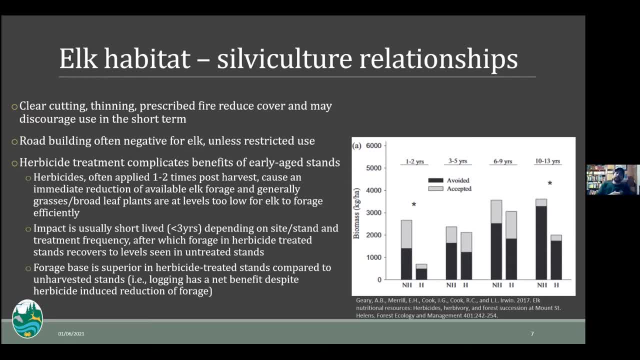 These are causing an immediate reduction in the forage that's available to elk. um, and what's left out there are at biomass levels that are that are too low for elk to efficiently forage in. Yeah, I just want to mention that a little bit in the last slide, where there's some trade. 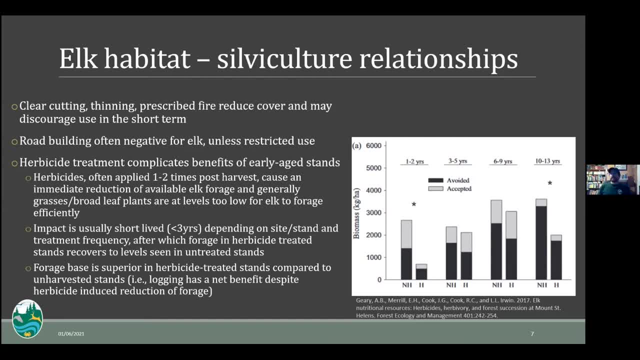 offs that were like there might be a little bit out there, but really an elk is not going to waste its time because it has an energetic apartment. It simply can't feed fast enough or consume enough across that area to afford to be an efficient payoff for them. 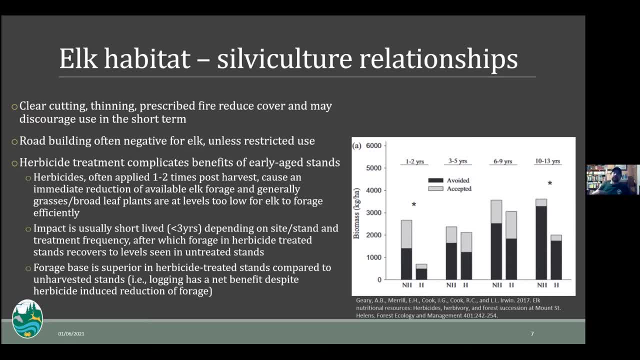 So that might discourage elk use. However, that impact is short lived, I'm typically in the order of less than three years and, uh, it sort of depends on the, on the characteristics of the specific sind wellbeing specific area, that specific stand, but after the sort of the effect of herbicides and this 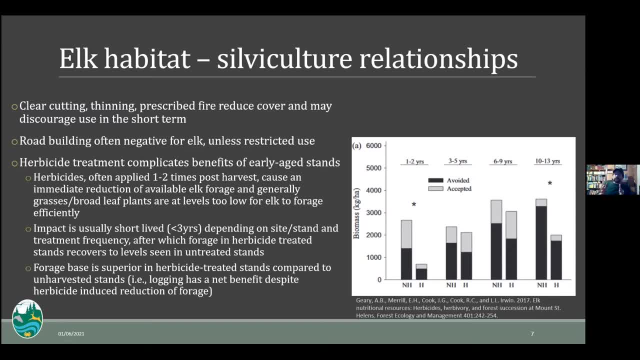 you know, about three-year window elapses. the treated stands are quite similar, in terms of biomass, to untreated stands, and so I'll divert your attention now from the text to that figure. here on the right, where we look on y-axis, we have biomass in kilograms per hectare. 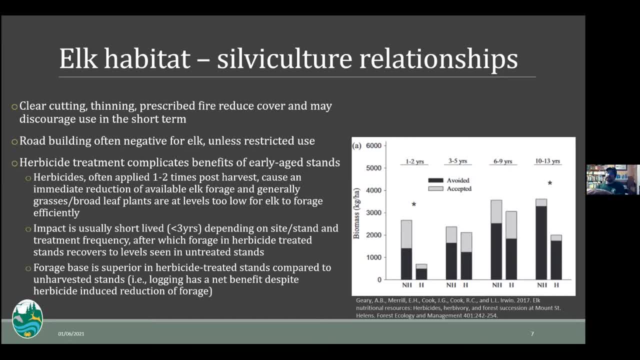 and then the x-axis. I'll try to explain this as coherently as possible. so we see a four series of two bars, and so look at only the two bars at one time. you see one that says NH and then H. the NH is no herbicides, the H is herbicide that carries through and is consistent. 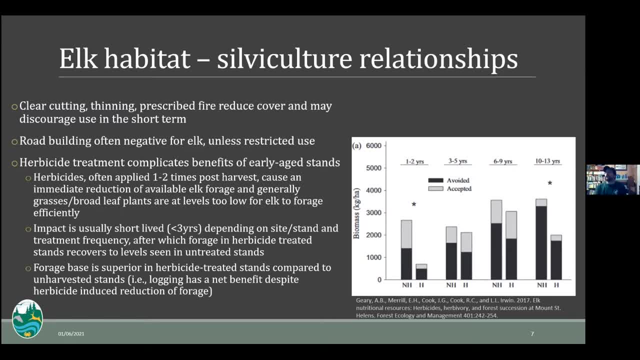 across and then you can see on the top here we say one to two, three to five, six to nine, ten to thirteen years, and that's, that is time. post treatment of herbicides. So another. you know there's a lot of information in this figure. I really like this figure. 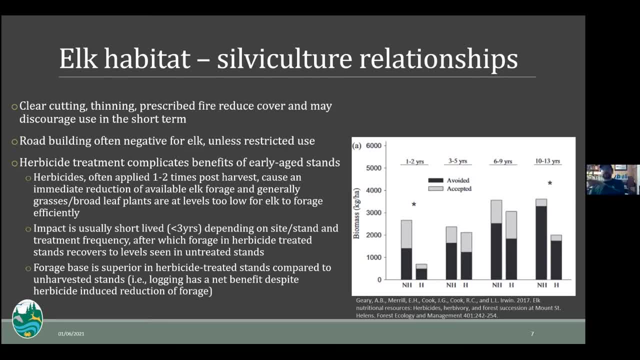 another component of this is it's a stacked bar, and so in the black you see the biomass of species that are avoided by elk. they're unpalatable, they're not really something they would prefer to consume, and then in the gray they're species that are accepted. so those are. 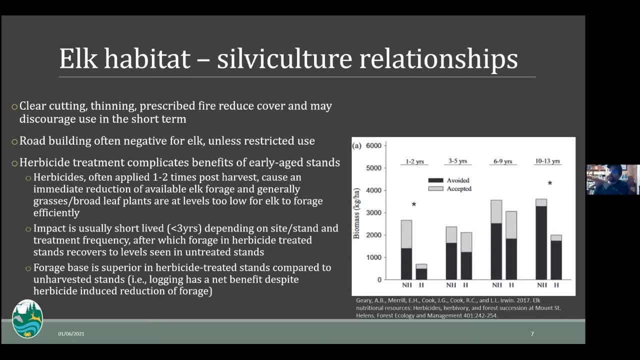 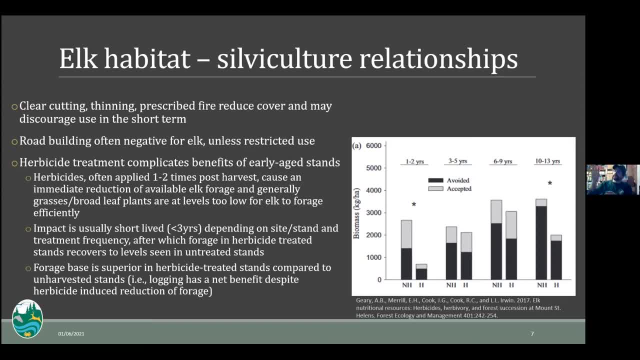 there's a lot of herbicides that are treated. the untreated stands, where there are no herbicides, have considerably higher biomass in them overall of both avoided and accepted species. but you can see, boy, there's a decent amount, it's almost 50-50,. you know, avoided and accepted there's. 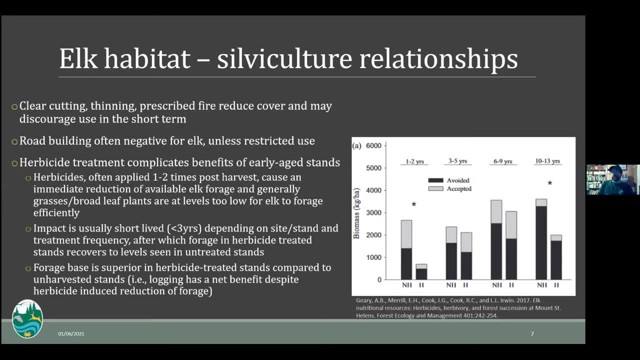 some. there's good eats in that, in that stand, compared to a stand that was treated by herbicides, where we have the majority of what's out there is avoided species and there's a little bit of accepted species in there, and you can see that, overall, though, the biomass is considerably lower. 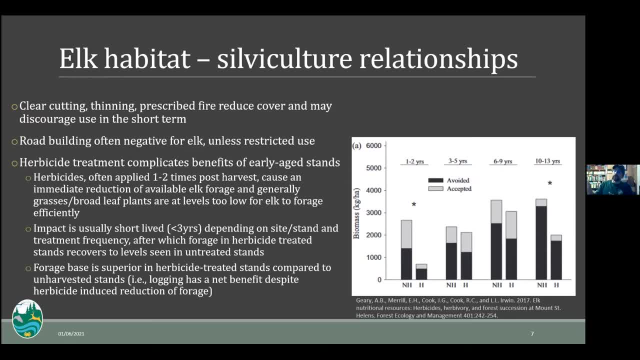 and i think that would just sort of tell you: well, yeah, geez, herbicides really do their job. that little star above there i i should have gone back and reviewed this paper, but i'm almost completely positive that, as an indication, there's a statistically significant difference between 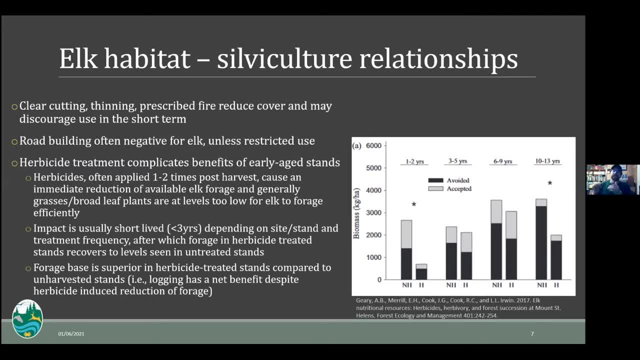 those two bars, and- and i don't think we need statistics to tell us that there is a a pretty apparent difference there. but what you can see is three to five, six to nine years um post treatment, that the levels of biomass that are out there sort of equate to one another. so 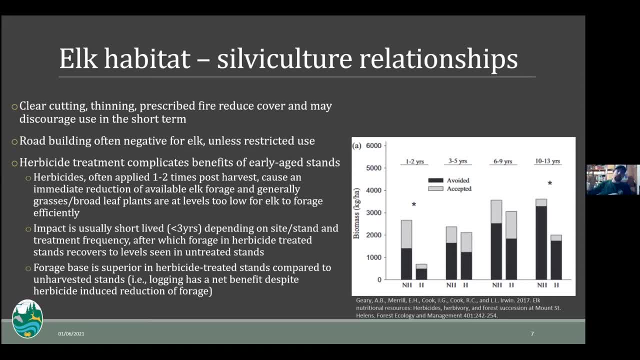 um in a treated stand, that no herbicide trans, no herbicide on the left and herbicides on the right. you know there's still a little less biomass, but not significantly different. and the ratio of avoided and accepted species of biomass, you know it looks, it looks pretty similar um, and that carries, that carries forward until that 10. 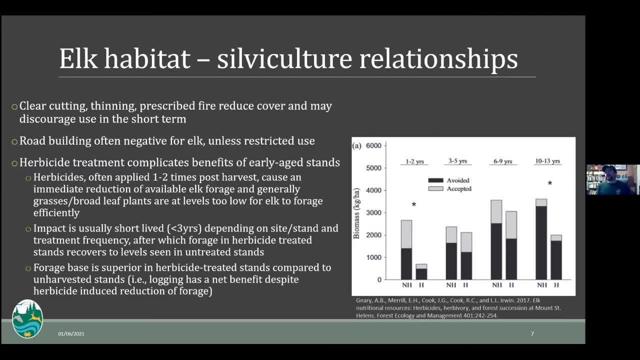 to 13 year window, where we seem to see a significant difference in the available biomass there. um, i'd have to go back and review that carefully to to offer up why that might be. but i think one important note there is that there's there's not a lot of accepted forage. that's that's. 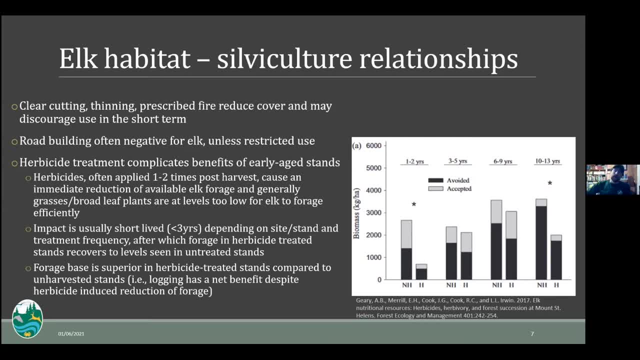 in that time period. so even then we're seeing these serial stands closing, transitioning probably more to the security cover type and less being less valuable as foraging areas. i think overall, to kind of summarize that is that you know the forage base is well, no, not to summarize this part. 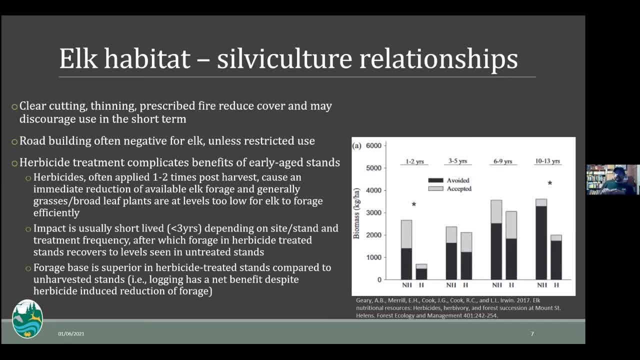 but, um, what that? one important thing that they found is that the forage base in herbicide treated stands compared to unharvested stands. so you got a stand that had a stand replacement event. you, you did some clear cutting, but just you used herbicides to give your- you know your- seedlings a. 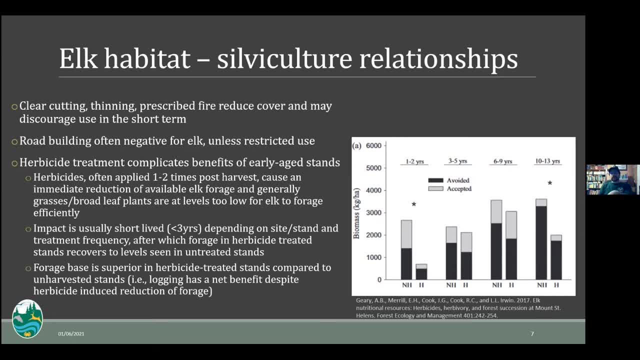 chance to establish themselves. and then you have a stand that's not harvested. maybe it's 15, 20, 30 years old. there's still a net benefit to doing that. logging the forage base is far superior in a stand that was logged and treated than it was in a stand that was not logged. so that's to say maybe. 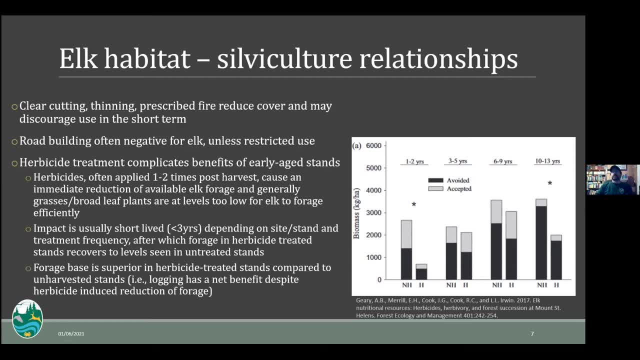 in a more simpler way that there's maybe that style of organization and denomination orextrawalk, that is лег mungkin, that there's a net benefit despite that reduction of forage that's caused by herbicides. So I think this is really interesting stuff and, and you know, Andrew Geary wrote up a 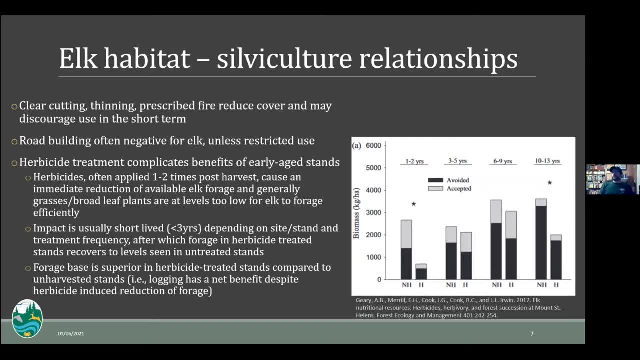 couple of nice reports. this is published work, but there's some, there's a lot of great information in there on kind of the history and some logging regimes and things like that of southwestern Washington that I would encourage folks to look at if you're interested. I don't know if I mentioned it, but that did that. 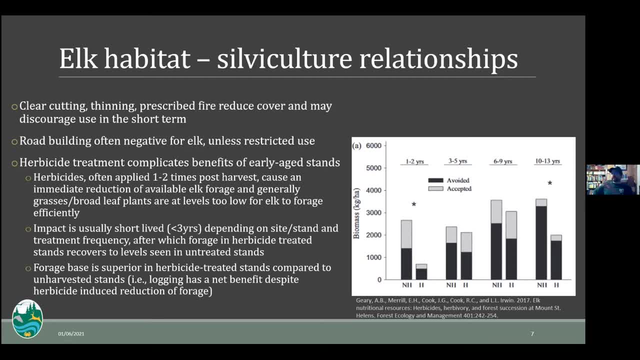 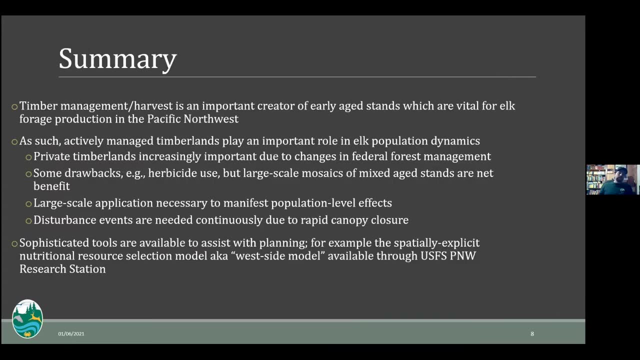 work did happen at Mount St Helens tree farm, so pretty relevant stuff here for for those of us in southwest Washington. Okay, so again painting, you know, broad brushstrokes, the, the timber management and timber harvest and silvicultural practices associated with that, the important creator of these early age. 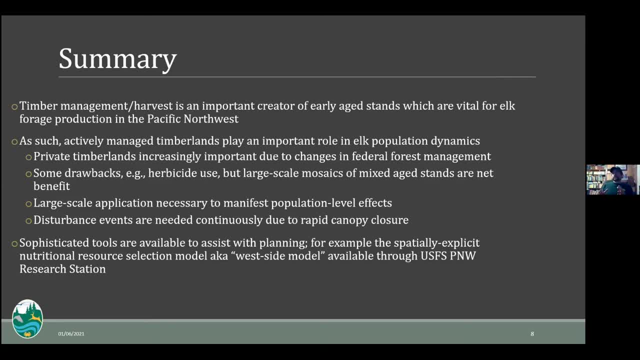 stands and and those early age stands are just simply, you know, vital to the creation of elk habitat and forage production, not only here at home and southwest Washington and western Washington, but really broadly across most of the range of elk. you know, a lot of what I'm talking about is specific to 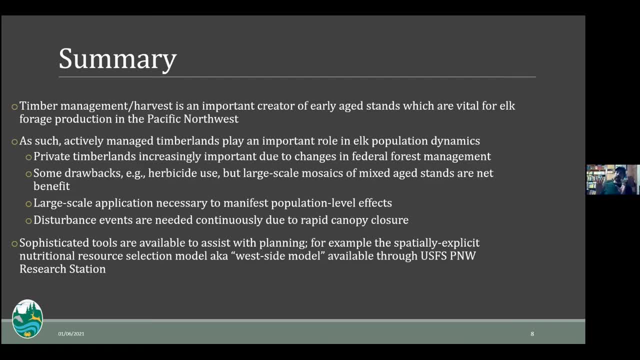 west slope Cascades, but these concepts really do, you know, kind of kind of weave through all different sort of ecosystems. so you know, with that of course these active timberlands are playing a really important role in the population dynamics of elk. Elk have to eat in order to survive a long time and they can't. 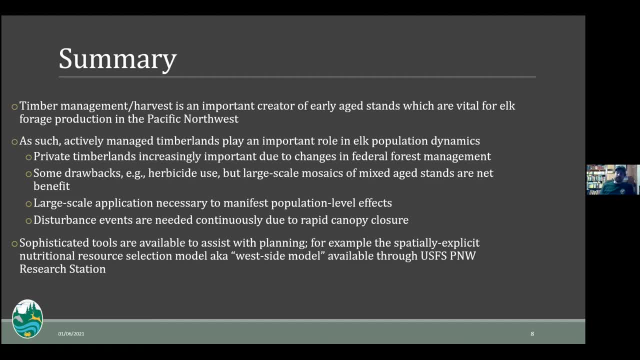 long enough in order to get pregnant and have babies and bring them successfully through their first winter and recruit them into the population as productive members themselves. So that's really important and fundamental. And the private timberlands- and I think this is really really interesting, One of the things that I continue to learn as a student of this- and 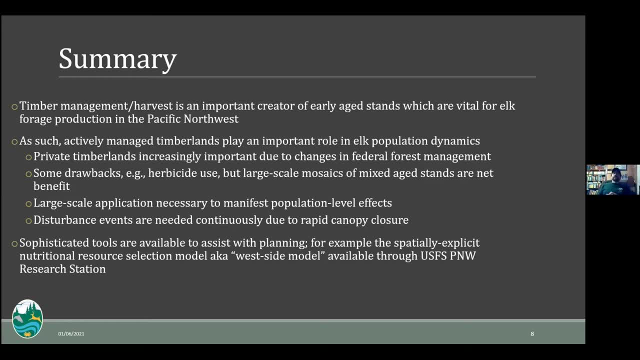 someone who didn't grow up with so much private timberland, you know they're playing such an increasingly important role over the last couple of two, three decades due to the changes in federal forest management, federal forest practices. Just thinking of kind of like the 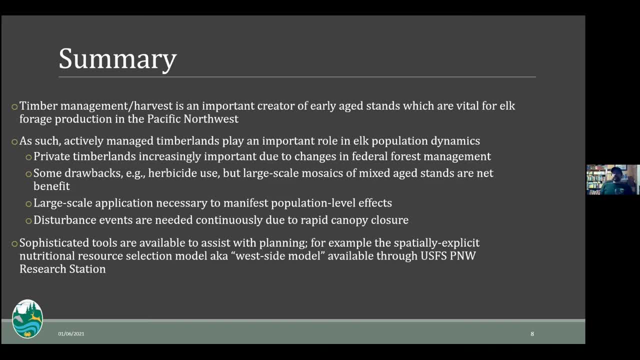 Mount St Helens tree really managed forest lands that you know aren't necessarily managed as actively as they used to, So a lot of the elk habitat is concentrated in some of these private tracks. There are some drawbacks, of course I mentioned. 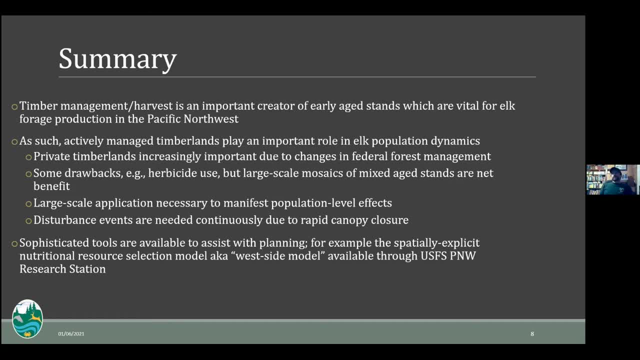 things like roads And of course I just, you know, showed you some data on herbicide use. but the large-scale mosaic that we find of these mixed-age stands across. you know, just zoom out to southwest Washington- have a net benefit, or at least you know, likely seem to have a net benefit. And then you know: there's a lot of you know, there's a lot of you know, there's a lot of you know. And then you know: there's a lot of you know, there's a lot of you know, there's a lot of you know. 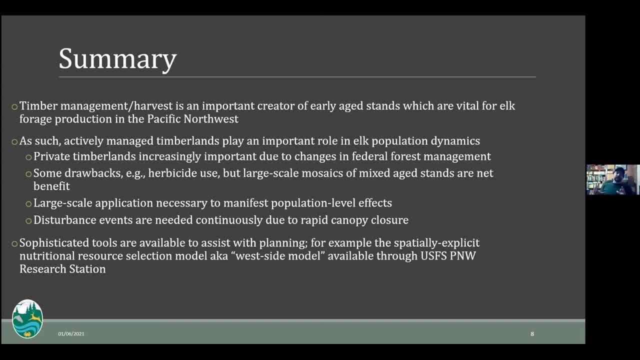 these things that are also part of the process of gathering these algae in some sort of communities that are then are able to support elk in numbers that we otherwise wouldn't be able to find. We wouldn't be able to sustain. We would simply see really closed-in forest lands and a very limited amount of food. We just wouldn't have the elk that we have now. 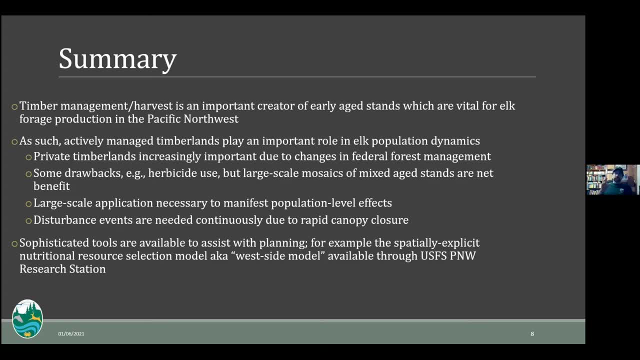 Northwest Research Station have put together over the last couple decades where you know you can still benefit elk at a small scale, and that's great and there's nothing wrong with that if you've got, you know, 10 acres of trees or something that you're going to go manage or thin. 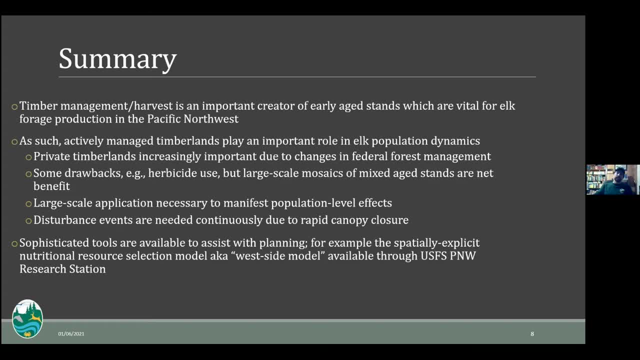 out, but as a Department of Fish and Wildlife, and thinking about how do we manage for large, robust, sustainable populations of elk. you know, we want to think about landscape scale, We want to think about large tracts of land that we can create this mosaic of. We've got security covers. 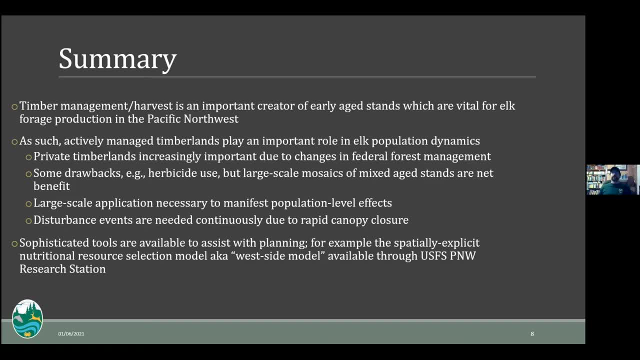 and mixed-aged, different cereal stages that provide for the different needs that elk have and that these disturbance events you know critically important to this, are needed continuously because, of course, trees grow and they continue to grow and the canopy closes and time goes on, marches on and we need to renew those early. 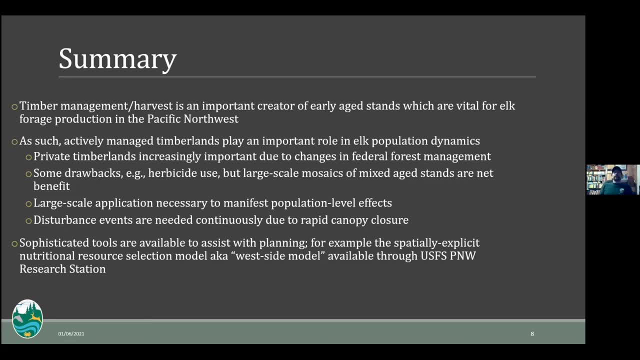 cereals stages if we're to create a stable kind of trajectory in elk populations, where you know we don't. we would love it if we didn't have boom and bust cycles in elk because we have, you know, periods of lots of timber harvest or we have, say, a volcano erupt and then we see. 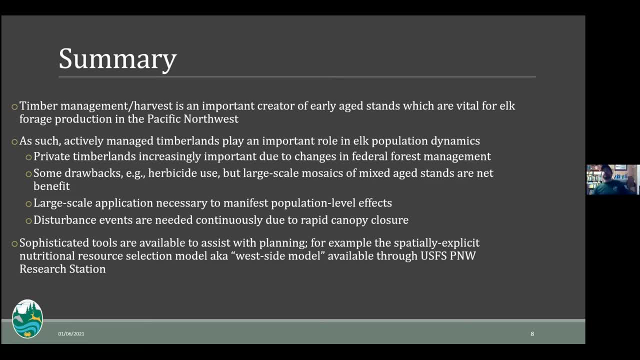 big growth and then feedbacks from not enough habitat out there and we see the population go down. We'd rather, you know, have that mosaic out there continuously that the elk population can sustain in a stable way. And for those of you that are interested in maybe taking this a bit, step, a step further, making 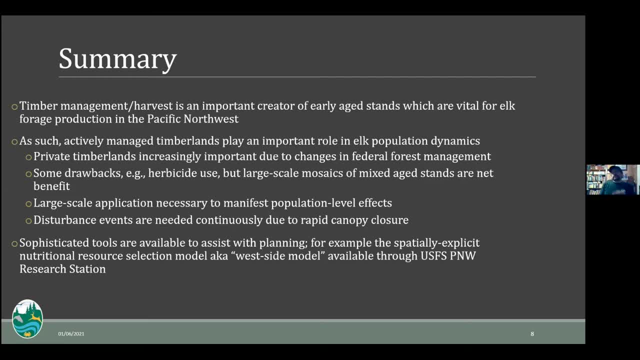 this a little bit more sophisticated maybe, and really getting into the weeds, say: you've got an idea, you want to implement some forest management on your tract, but you kind of want to be strategic about it. There's some really sophisticated tools that are available, notably out of the Pacific Northwest Research. 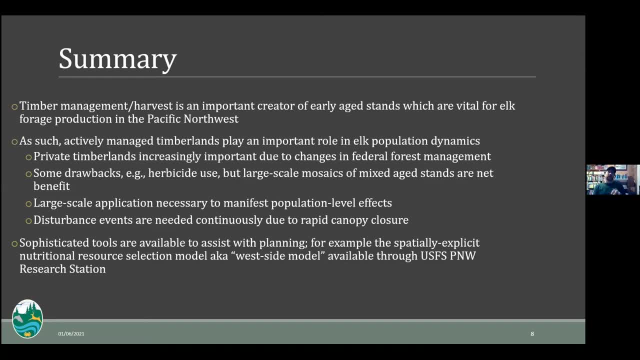 Station. some folks- Mike Wisdom and Mary Rowland, and the folks I mentioned earlier, the John and Rachel Cook, and a multitude of other folks- have put in decades of work to create this. what's this fancy sort of name of a spatially explicit nutritional resource selection model, also called? 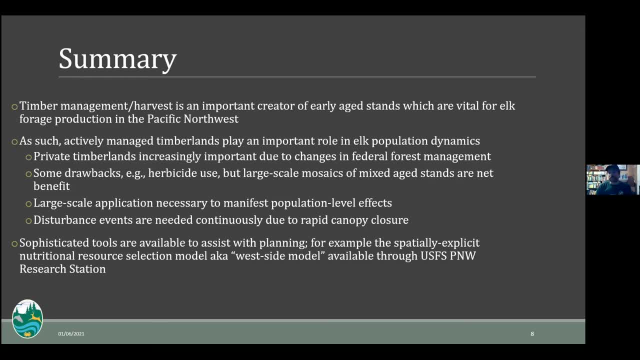 the West Side Model. but really what that is is: it's a model that goes in a geographic information system, a GIS, and you use it. you can use it in a multitude of ways, but you can use it to assess the habitat suitability. you can assess the. 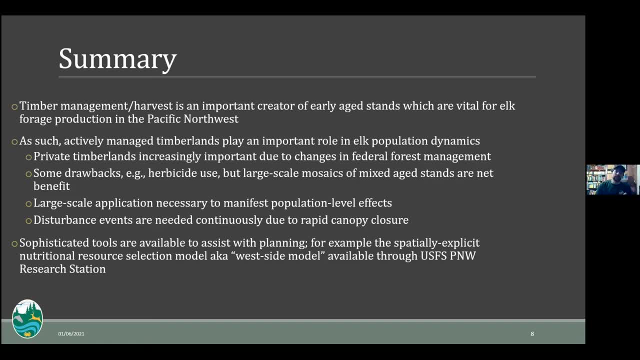 probability of use by elk and you can manipulate some factors in there. So what if you're going to put a road in somewhere or you're going to cut three forty-acre sections- what that might do to the probability of use? you can eliminate some factors in there. so what if you're gonna put a road in somewhere? you're going to cut three? 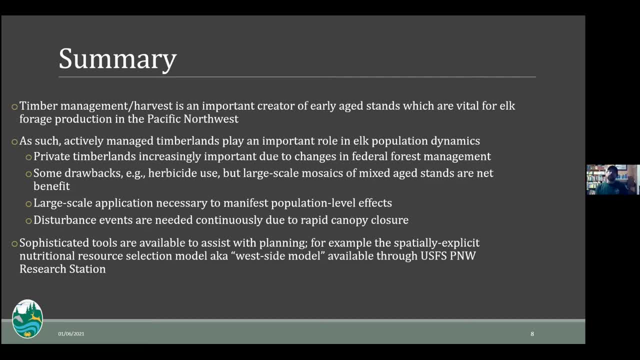 forty-acre sections, what that might do to the probability of use, and then kind of slide these through, kind of get a sense of what that is conceptually. So you know this is a pretty complex process. It takes a lot of time to think about it and then you kind of need to do a lot of trial and error to make sure that there's enough evidence that we're 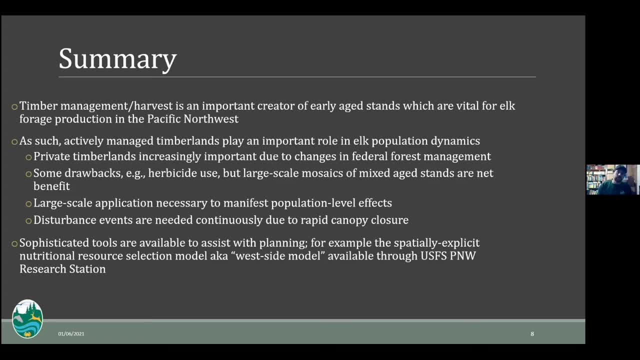 to the probability of use. Now again, this isn't necessarily the most approachable technique. I don't know how user-friendly they've been able to make this. I haven't looked in a while, but if you're interested in that, you know contact me or contact them directly at the Pacific Northwest. 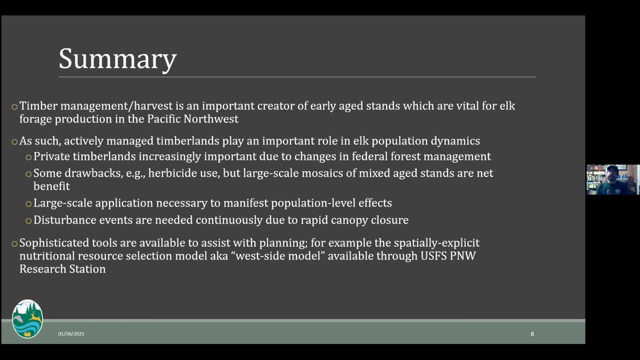 Research Station and they can probably guide you. I imagine they're very eager to have folks implementing those resources and using those. It's probably geared a little bit more toward, say, forest- you know the federal forest managers- but can also have some utility for other folks. 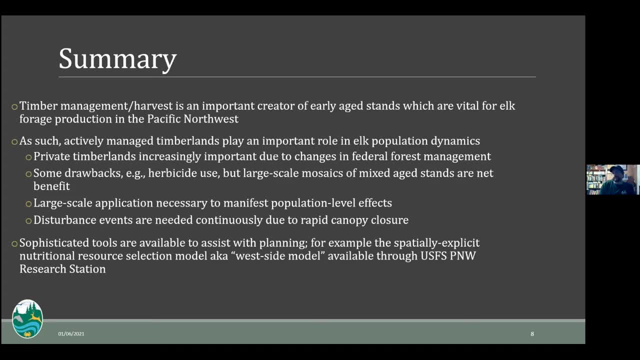 that are interested in trying to find this balance between, you know, timber management and also supporting, you know, healthy, robust out populations. So I think I offer out some resources here and you know I'll share the. I can share a copy of this, so folks. 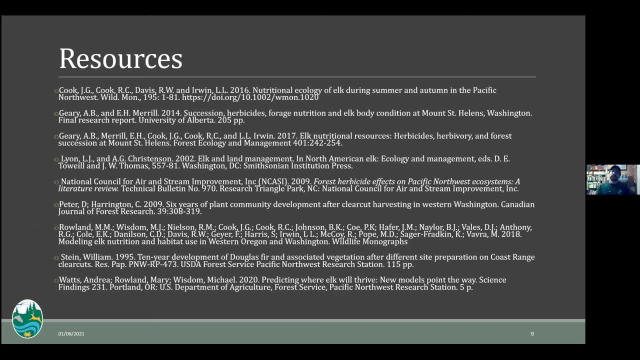 have this. This is just a small sort of select snippet of what's out there. You know there's probably 60 to 80 more articles that I could have put up here that would have been worthy of review, So I'll throw these out there. We can get them to you so you can review them at home and, if you, 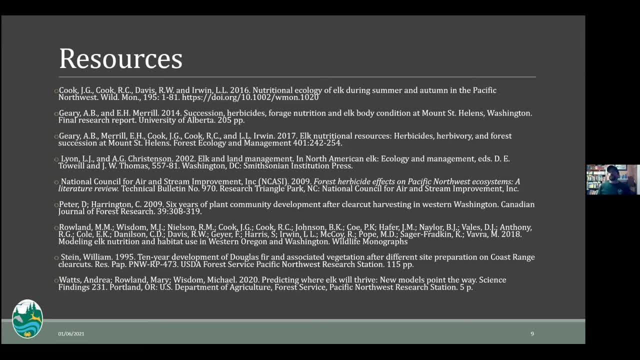 have an interest in any of these articles and reviewing them- and you can't access them because sometimes they're behind paywalls- reach out to me and I have these articles and I can get you the articles if you're interested. I'm interested in reviewing them further. 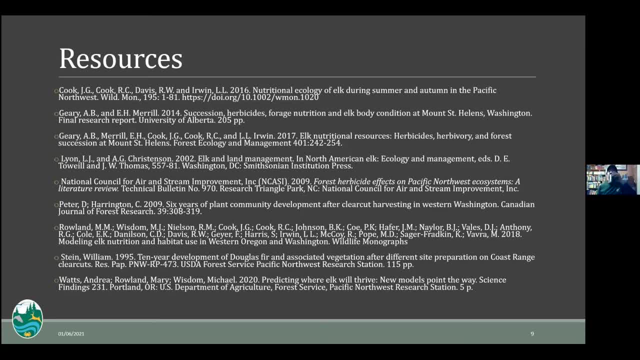 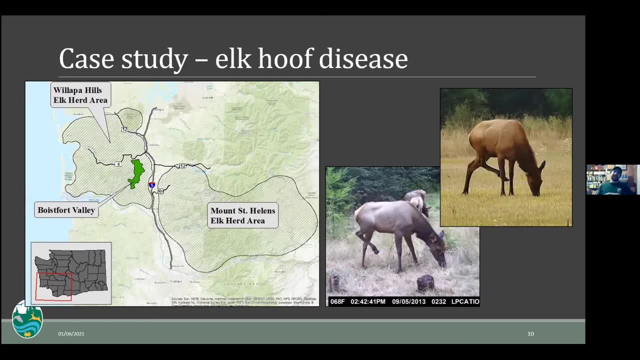 Okay, so, moving to the second part of this talk, where I'll attempt, I'll say that I'll attempt to try to tie in some of these concepts with Elk Hoof disease and what we've seen with Elk Hoof disease and what we're learning about Elk Hoof disease. So I think probably the majority of 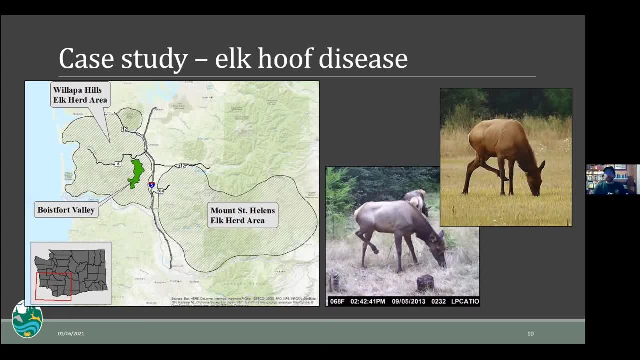 folks in this audience are aware of Elk Hoof disease. If you're not, you can't read this article. It's a bacterial disease that invades the hoof tissues of elk and causes lesions. deformities, is clearly a painful condition and you can see here there's a sort of 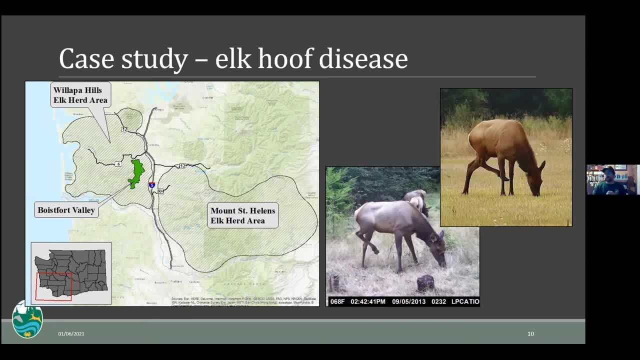 characteristic classic photos of elk that have infected hooves. they hold them up. it causes a limp and an abnormal gait And you know, of course it often leads to some of these secondary effects Of you becoming malnourished. 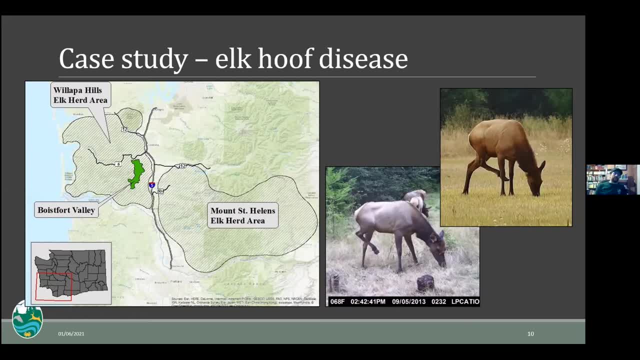 the infection progresses because if it causes a secondary infected and it undoubtedly, you know kind of contributes to the demise of the animal, Unless that's interrupted by, say, you know, being harvested or something like that. The disease, we don't exactly know when it emerged, but it emerged probably in the early 2000s. 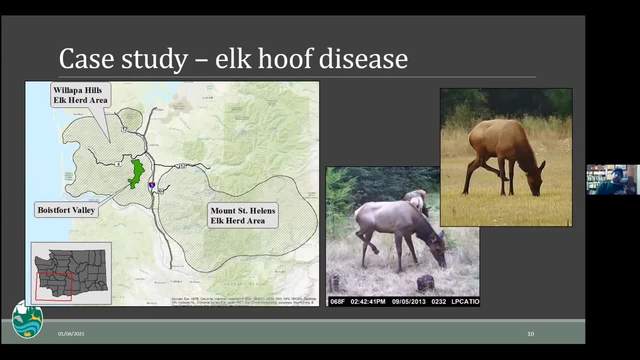 in the Boise Valley That's highlighted here in this map. on the left that's the Willapa Hills elk herd area and you know a number of years, maybe five to eight years or so after its emergence. we're not entirely sure. again, it's kind of hard to know. the disease crossed over I-5 and got into. 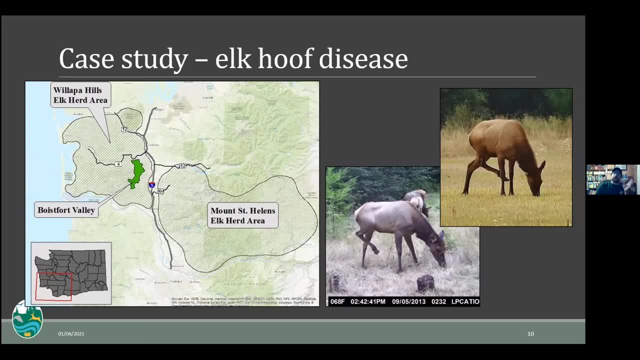 the Mount St Helens elk herd area and the core of the Mount St Helens elk herd population in that sort of you know Toodle River drainage and when it got into the Mount St Helens elk population it really spread quite dramatically in its distribution and it also increased quite 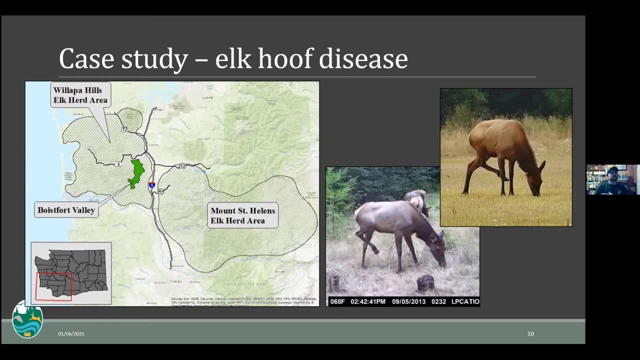 dramatically in its prevalence, the number of animals that were affected by the disease, as opposed to what we saw. say, the Willapa Hills, where there were definitely animals. it was a, it was cause for concern, but we weren't seeing. you know, for instance, over half the groups in an 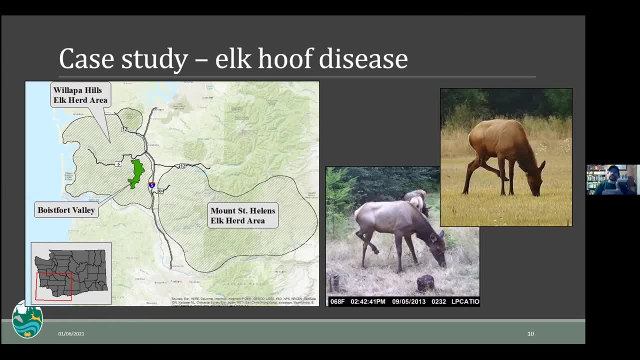 area that were affected by the disease and so we're not seeing that in the Willapa Hills survey having at least one member with the disease. I mean, there was a lot of animals especially. you know, probably 2013 to 2016 is when maybe we saw the peak in prevalence. 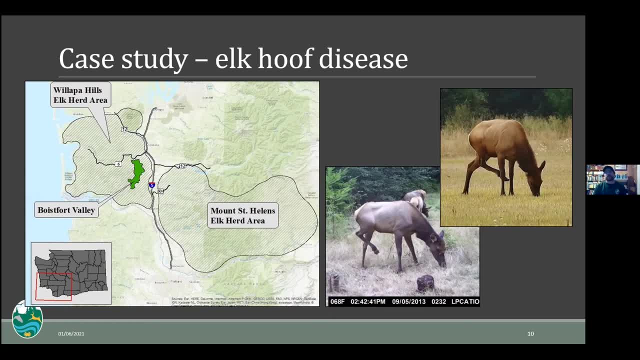 the reasons for this sort of differential pattern in the disease when it got into Mount St Helens aren't really understood and they may not truly be perfectly understood, but a reasonable speculation, at least in hindsight, is is due to the background, nutritional limitation and condition of this. 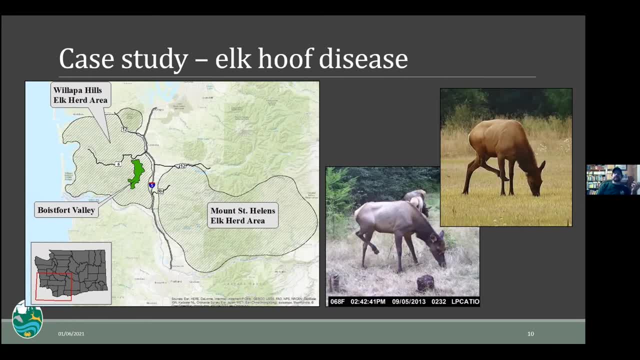 population, sort of population-wide limitation. so I mentioned a little bit earlier, I think, a couple of times about the eruption of Mount St Helens and again, I think a lot of the folks in the audience are well versed in this history. but that eruption, you know, was a cataclysm that destroyed a lot of. 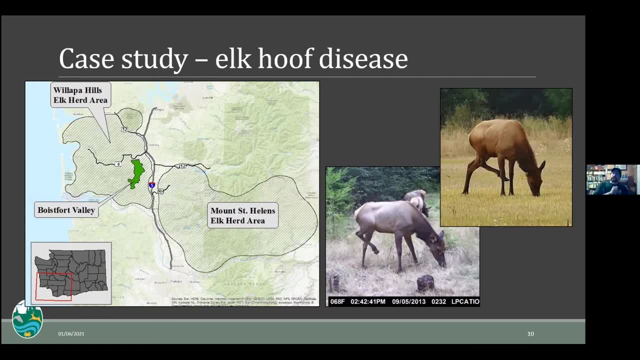 elk habitat, a lot of elk and a lot of others, and I think a lot of the folks in the audience are well versed in this history. but that eruption, you know, was a cataclysm that destroyed a lot of other wildlife and was it was a tragedy on a really large scale, but one of the outcomes from 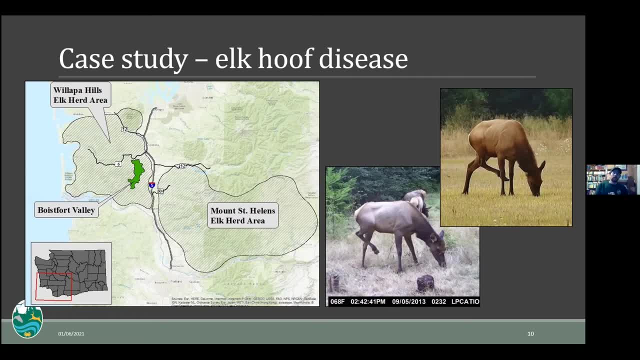 that was the creation of massive, massive tracts of early cereal stands and we we saw elk recolonize that area. there was lots of replanting and for that 10 to 15 year period post eruption it was really really high quality elk habitat and you know, really you wouldn't have wanted to be an 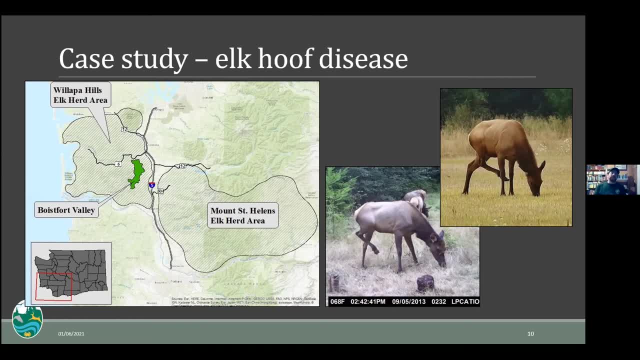 elk anywhere else in the world. you know you wouldn't have wanted to be an elk anywhere else in the world. you know, really you wouldn't have wanted to be an elk anywhere else in the world besides Mount St Helens at that period of time, as the canopies began to close, however, well and so. 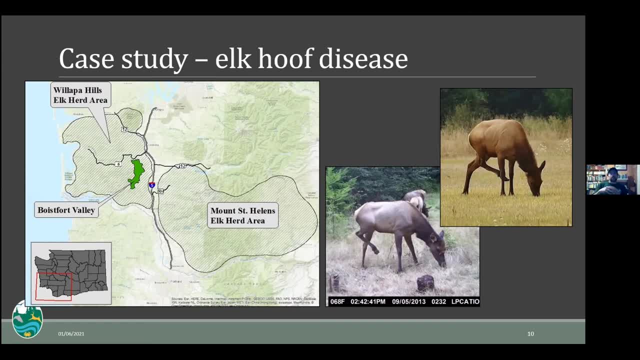 I guess I'll finish up by saying we had a. we had the population really grew and became very, quite, quite dense and you know the the Mount St Helens elk population has a storied history of of really being one of the premium populations and and really it was a destination population for a lot. 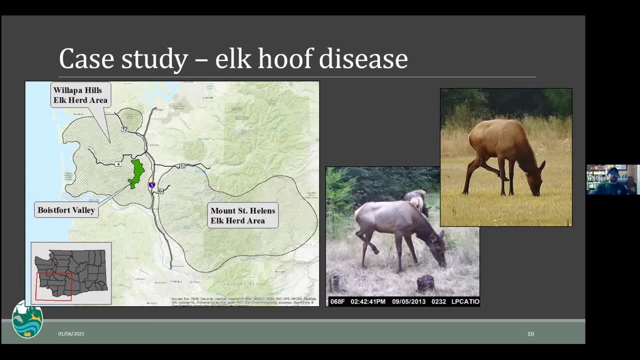 of people to come and view elk and to hunt elk. but as that population, you know, kind of reached its apex in density and the number of animals that were out there, we also started to see changes in those in the forests and in that early cereal stage began to transition into later stages. that 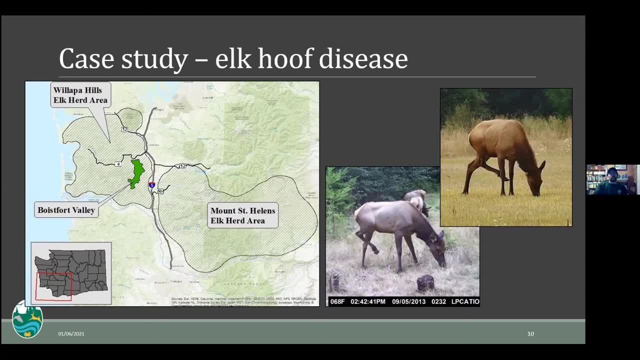 15 year period and onward, where we have canopies that are closing, the benefits of those early cereal stages in terms of forage started to become diminished while they're still active. you know forestry happening at that time. we also see some changes that happen on the federal forest. 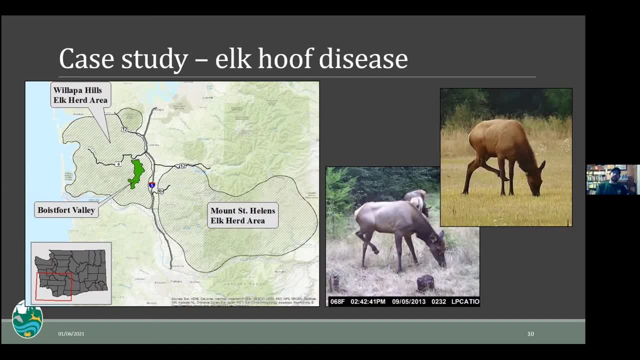 lands in the in the 90s that reduced some of those forest management practices and civil cultural practices there. and so we see we have the forage resources becoming reduced. some changes at the federal level, some changes on habitat sort of area. well, population area wide, but we have a very dense. 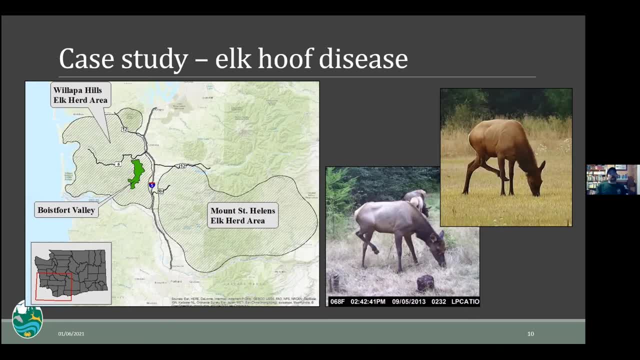 population. so as the population ended into the 2000s, we we started to see these feedbacks are called density dependent feedbacks- in this population where um only has kind of had this, this tendency, that if they they can achieve really tremendous and rapid growth um and overshoot their carrying capacity and 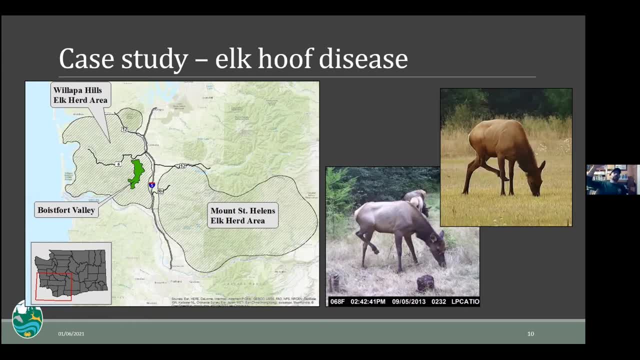 meaning they overshoot what's available in terms of nutrition in the landscape. when they overshoot that, they can actually kind of hang out up there for a while. you know, just teetering around, you know carrying capacity, but when they're when that happens, you often see feedbacks of, say, low. 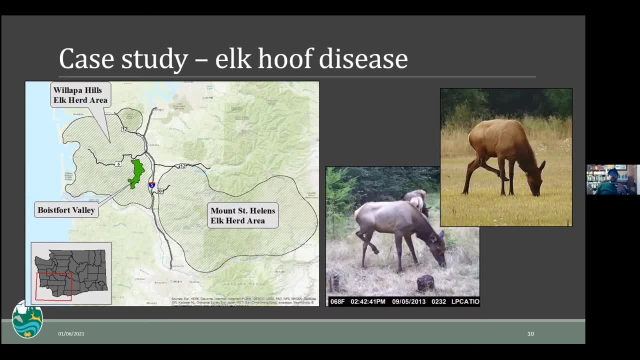 pregnancy rates. um, you see, uh, maybe low juvenile survival and ultimately you might see the feedbacks in adult survival. that's kind of the last thing you would expect to happen. and those are all sort of functions because there's not food out there and it's a hard living and and their body condition. 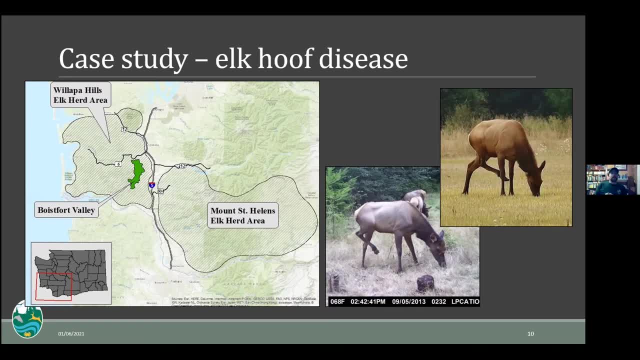 decreases. we started seeing that in the early to mid-2000s. we started seeing um. it's a little harder to tease out some of the productivity issues, but one thing that I think uh is kind of always really surprising to me is that we would have winter mortality counts where 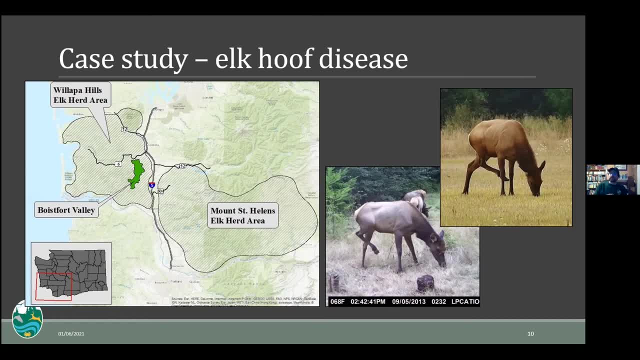 we would encounter lots of dead elk. um, you know in March that that had died that year and that's really not something that you see very common. I mean, even in extreme winters like think about Yellowstone and other areas where you have really, really extreme weather- you don't have lots and 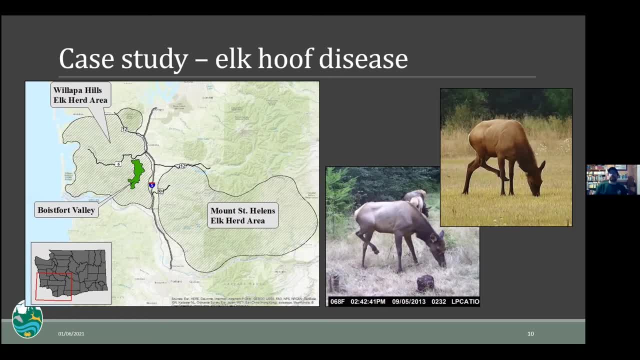 lots of elk just tipping over, unless they're nutritionally limited. so, um, the, as, as we continue to document those, those limitations, um, and we began to try to manage against that and reduce the density of this population through harvest, the disease emerged and it really spread to this population quite rapidly and it remains. prevalence remains highest. 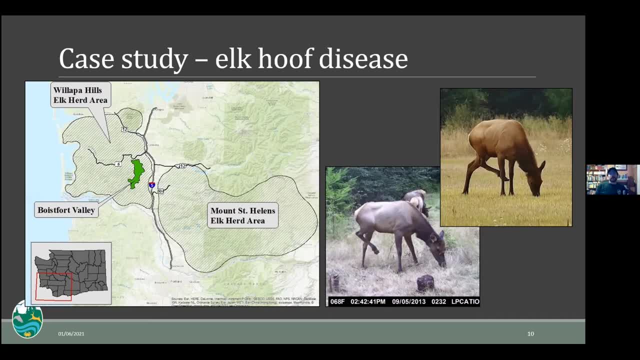 in Mount St Helens, um across the state, the. the disease unfortunately has spread in its distribution to affect quite a number of our out populations, but prevalence still remains, to this day, highest Mount St Helens and the nutritional limitations are probably highest in the Mount St Helens elk herd. so we initiated some research in 2015 to 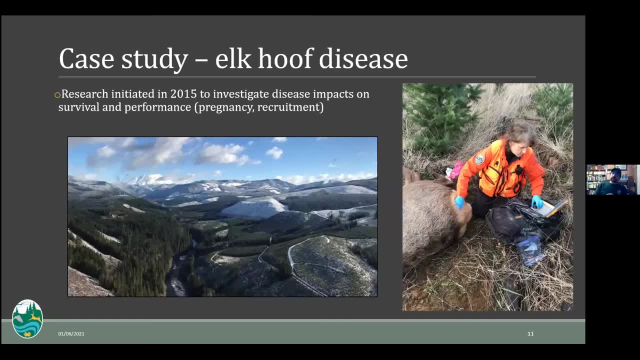 try to investigate the impacts this disease might have on the survival and performance of animals. uh, in Mount St Helens, and so this is just an image here of, of you know, this landscape of the of the mosaic of the Mount St Helens tree farm. you can see the monument and the mountain itself in the background. 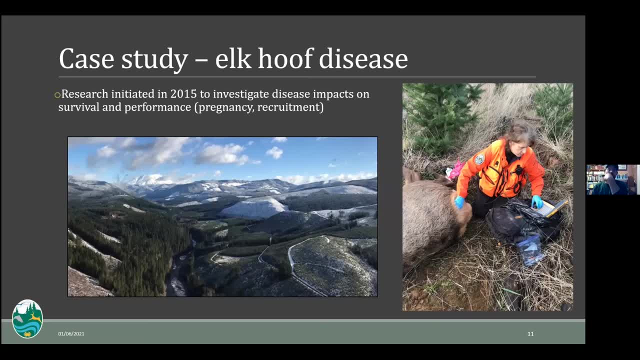 during this project we captured 180 animals, over 257 capture events. when we capture these animals, we monitor them, for we assess their body condition, we get estimates of body fat. that's what Dr Mansfield here, our wildlife veterinarian, is doing. we uh, we determine pregnancy status, lactation status and 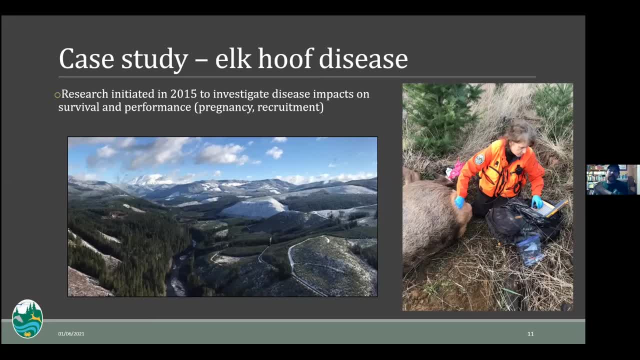 of course we assess their hooves and then we throw a collar- GPS, radio collar- on them to monitor these animals through time so that we can estimate their survival, which is really important statistic to understand the population Dynamics and also to understand why these animals are perishing or cause specific sources of their mortality. so I'm going to breeze through a few. 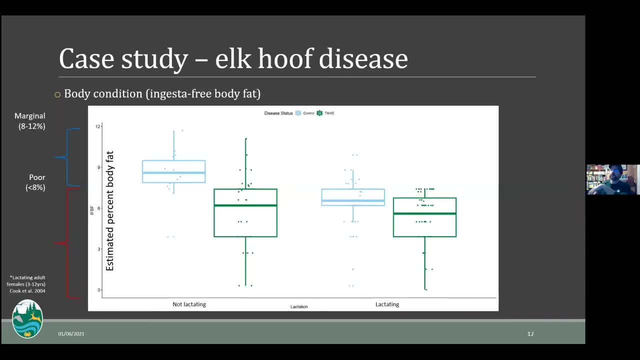 results. but I think this is the one that I kind of really want to show a figure on and and and just underscore this nutrition. right here we're looking at body condition as estimated through percent body fat. um, this, if we, if we just look at the at the bins here, this is a box and whisker style plot, and so when blue, we have animals that 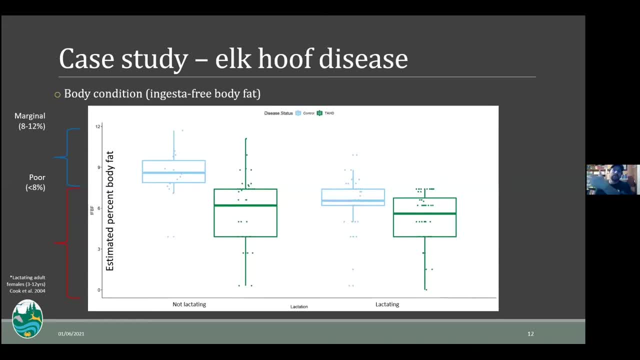 do not have the disease at capture and in green we have animals that do have the disease at capture. so we have an uninfected and infected, and then on the lab you see we have them in pairs, where you have animals that are not lactating and animals that are lactating, and I should have 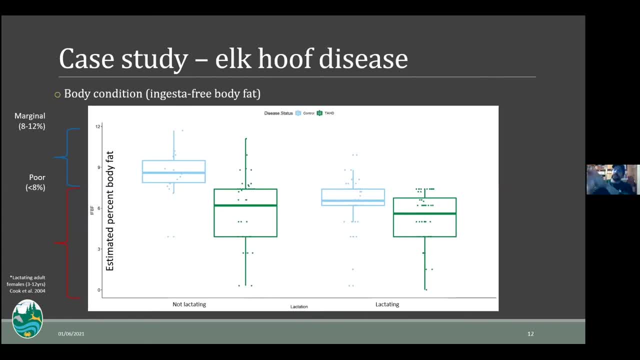 mentioned that we only captured adult female elk, because they're really the drivers of the population Dynamics. so what this shows you is the spread of the body fat of the animals that we captured, and you can see that those animals that are green in this box. this is the range of data, of values that we saw. 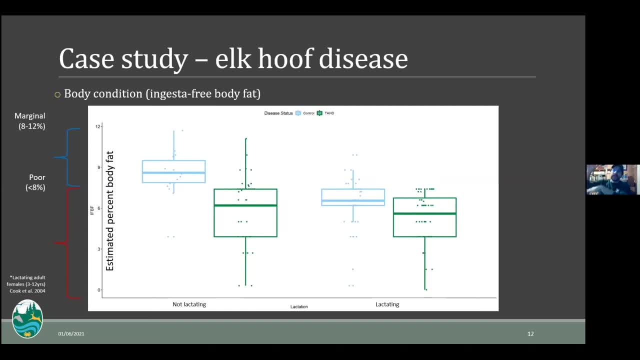 that bar. there is kind of a good way to look at the central tendency, that's the median of of where we sort of you know, expect these animals to be. so you can see that overall, animals that are infected with a disease in green have lower body fat. 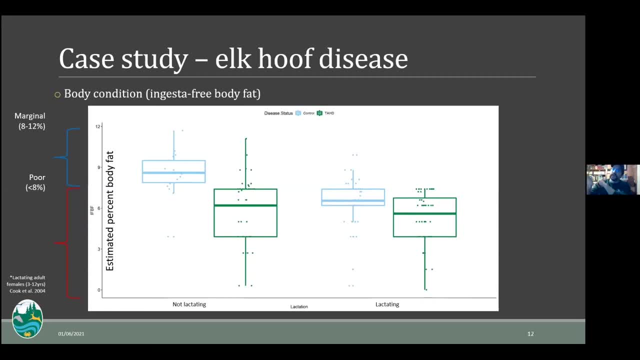 animals that are larger and animals that don't have the disease in In Bloom have higher body. on the left I've sort of created a few bins here where you see poor less than 8% and marginal is 8% to 12% And that's just sort of to say that you know if you put the words survival probability. after that or whatever other description is what you kind of find. So if you have less than 8% body fat, you have a really poor outlook to be making it through winter. If you have 8% to 12%, yeah. 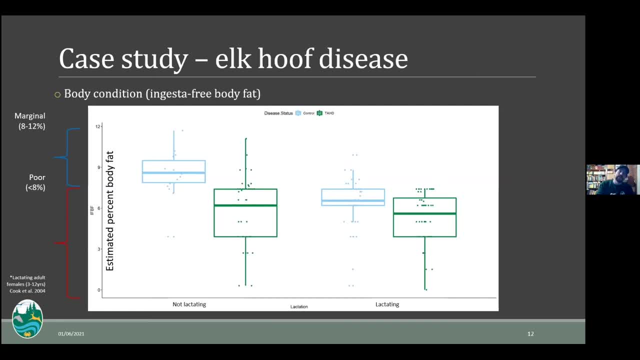 it's okay. If you have less than 8% body fat, you have a poor probability of becoming pregnant. 8% to 12%: yeah, it's okay. So that's kind of the relationship there And that's what to tell. 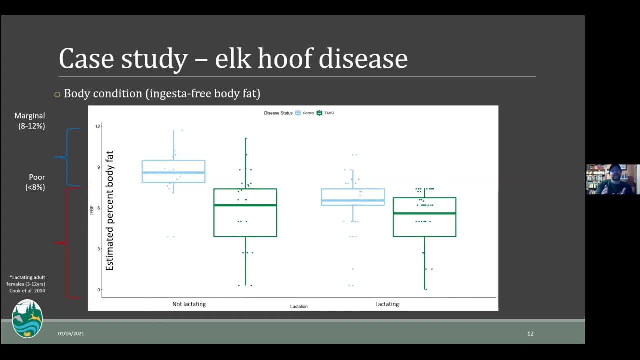 you here is if you just kind of look across. well, none of the animals we captured exceeded even marginal body condition. So that's important. This underscores that background nutritional limitation, but that those animals that do have this disease they are in lower body condition. 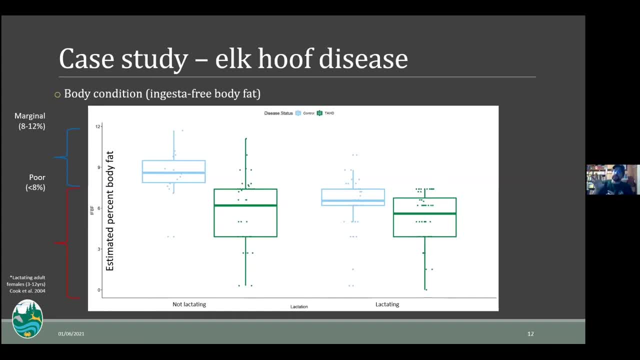 It does seem that the effects of the disease have an effect there in reducing the body fat, And that just makes sense. right, You're fighting off this terrible disease. It's metabolically costly, you know, energetically costly, to fight a disease off like this. So it makes sense that. 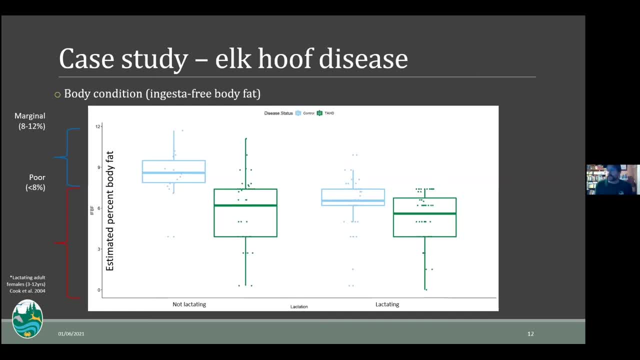 you're not going to accrue a lot of body fat going into winter, And so I've talked a little bit about you know how body fat and body condition really have important feedbacks down the line in terms of an animal's ability to become pregnant, to conceive or even to go into. 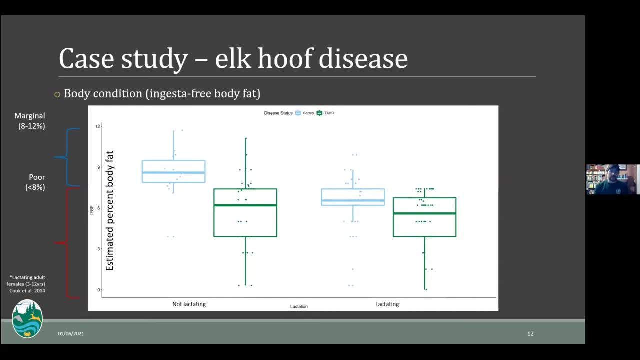 estrus. And then if you look at the body fat, you're not going to accrue a lot of body fat going into winter. Then raise the calf or bring the calf to term. raise the calf for summer has all these downstream effects And I'll just show you a few things here. Ignore the graph for a moment. I meant 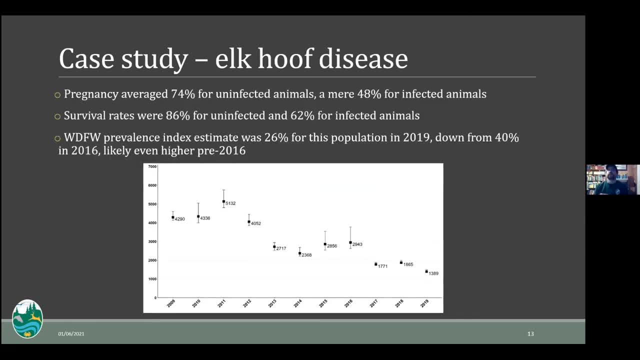 to have that sort of transition in. But for those animals that don't have the disease, that are uninfected, we have an average pregnancy rate of 74%ler, Whereas infected animals- this is just a really surprising statistic. Whenever I see it- is 48% for those animals. 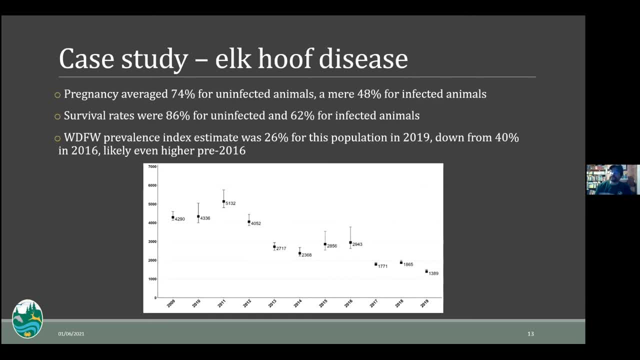 that have this disease. that again just bears out this important relationship between nutrition and these downstream effects. Normally you'd see that you know quite a bit higher. it sort of depends on you know how many you know yearlings and how many old age individuals you have out there. but it's not. it's not great. we would expect it to. 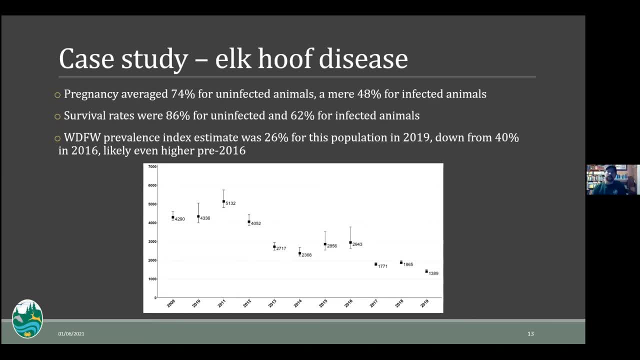 be higher for any elk population anywhere else. for uninfected animals it's. it's a little lower than you'd want from a population you want to see growing, but certainly drastically low for those animals that have the infection. Survival rates were pretty similar. remember I said you know you. 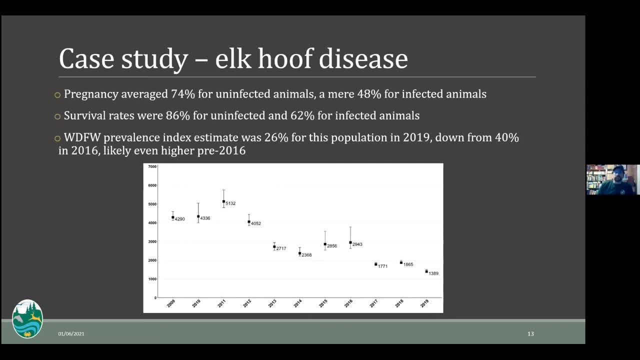 have a poor probability or you have a marginal probability. well, elk are really tough animals. so you know, even with the body fat levels, they are going into winter with those uninfected animals. so that about an 86 percent annual survival and whereas those infected animals, those animals with hoof disease of all types, 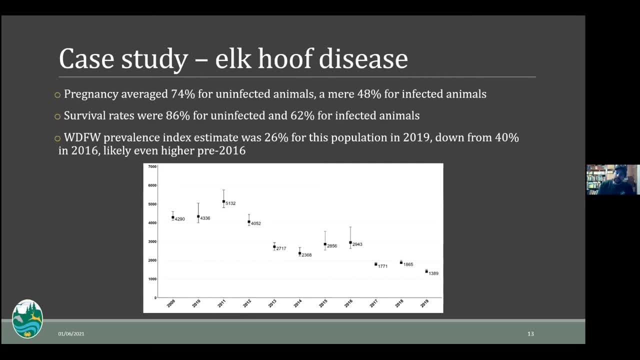 of grades because there's a. there is a bit of a spectrum of infection. it's 62% in a normal population of elk. you know you're gonna see if it's, if it's a hunted- you know where there's female elk being hunted- you're gonna see. maybe 85 or so percent depends on your management objectives. if 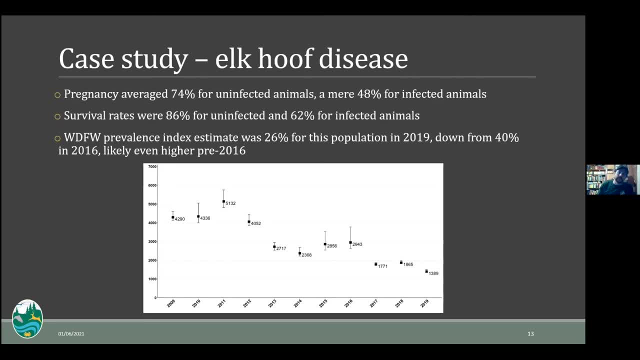 you want the population to go down or not, but you'd normally see something like 90 or higher, with an unhunted population of 90%. survival for female elk and then- so that's just to say there. that that's 62% for infected animals- is again, you know, really quite a bit lower than what you'd. 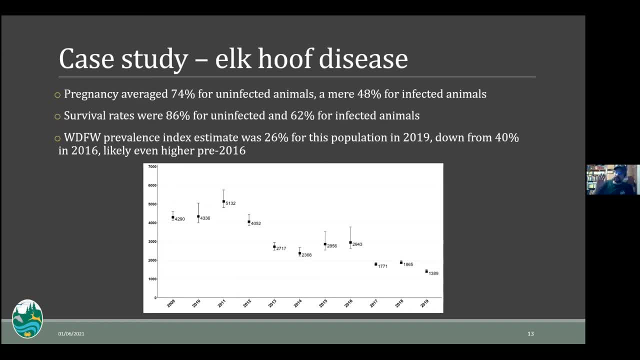 want, and these are ingredients of a recipe for population that's not going to be performing very well and not going to maybe rebound really quickly with these rates, depending on how many of those animals that you have, they're infected. you know the uninfected animals they have. so-so rates of pregnancy and 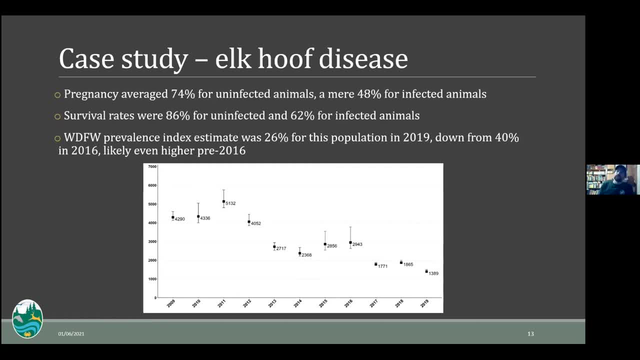 survival. but those infected animals, if they comprise a large majority of the population, they're going to be really well affected. So that's really weighing it down. so prevalence is really difficult to estimate but we've come up with a few ways to do it in the 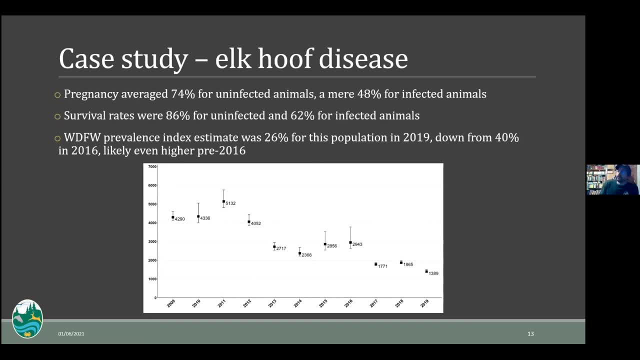 Department of Fish and Wildlife and the primary way that we do is through hunter reporting and that's a more of an index estimate of what prevalence is. but nonetheless it's 26% for the for the Mount St Helens elk population in 2019. 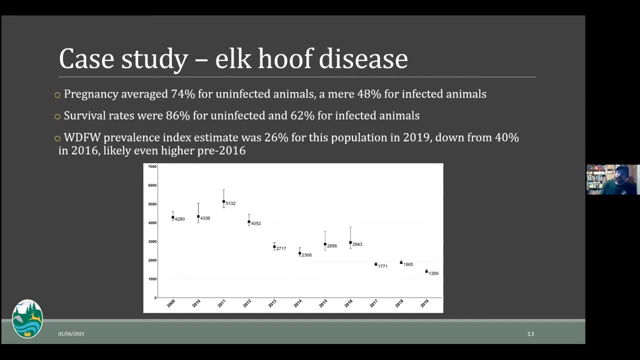 the core units down from 40% 2016. so that's a good trajectory and that was probably even higher in 2000, before 2016, when we initiated that that estimator. but I put the figure down here below to sort of highlight what that might mean. 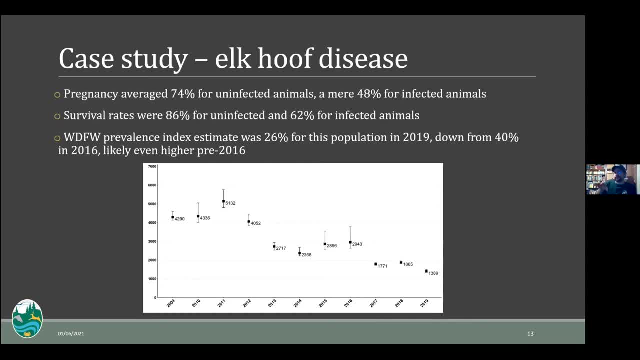 for the population trajectory. so these are estimates of what the population in the the core of Mount St Helens. we survey them almost every year, usually every year. COVID stopped us last year but you can see in 2009 to 2012 we've got. 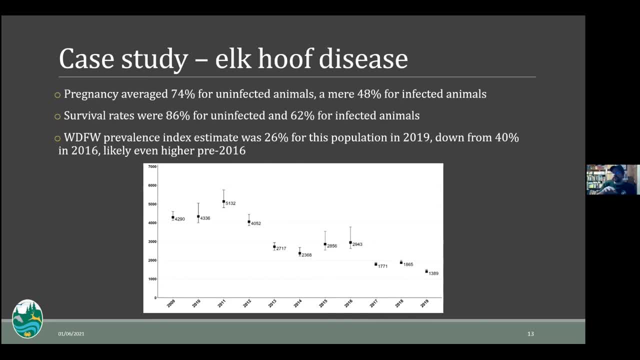 a population that's pretty high. you know Cebu and San Diego are pretty high and Booms and Busts and that's at that time we're actively trying to reduce the population, lower its density, to stem off some massive overwintered eye off or 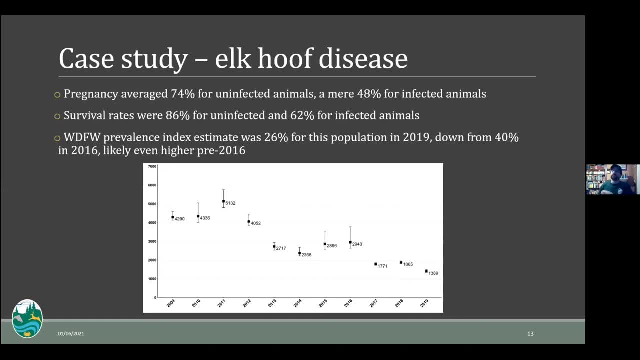 whatever it might be to get the population back in line with with its habitat. and then the disease emerged and that story began and we pulled back on antlerless harvest but we continued to see those declines and in here we see a few really bad winters and you can imagine you have a bad winter event like 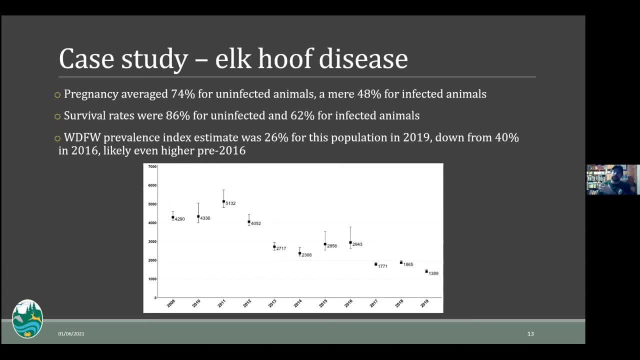 in 2017 we had a pretty rough winter. you have a lot of animals that are in pretty rough condition and you know some animals that are in really bad condition. that's going to have some overwintered mortality and consequences for your dynamics. but the the underscore here is really that the rates that we've monitored, that we've 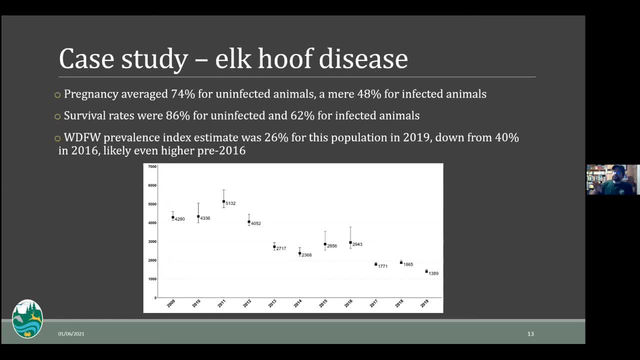 measured we're still. the next step of this analysis is to actually use projection simulations to see what might happen in the future if we're able to reduce the prevalence, say maybe to 15 percent, what that might mean for our expectation in this population moving forward. because you know, we, we all know how storied this, the history of this, 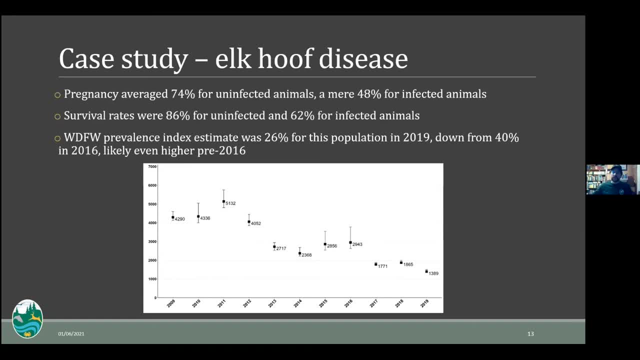 population is and what it might be able to achieve. we have a different habitat landscape. that's out there- but we'd like to see this population kind of tick back up and come back to more objective levels. right now we aren't at objective levels in those core GMUs and so if we're able to reduce and manage prevalence, we might see that and see that those at the core GMU issue. 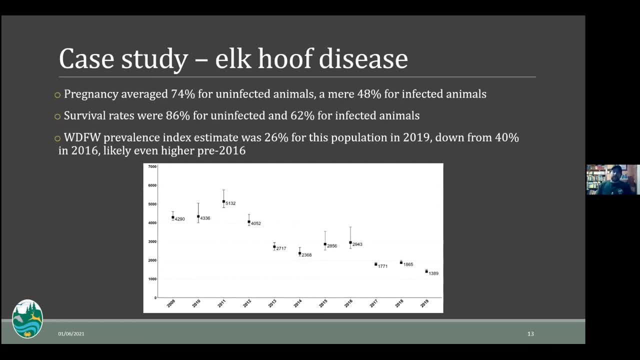 that tick up quite a bit more rapidly And we might see it come up no matter what, even if population prevalence stays kind of where it's at. So to kind of try to wrap that up, I know I've sort of belabored a lot of this- 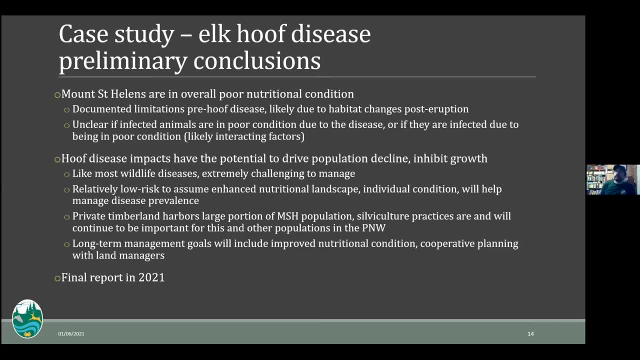 the Mount St Helens out population overall is in poor sort of nutritional condition And these limitations have been documented before hoof disease and were well known before hoof disease emerged and that they were likely due to the effects of the eruption, the boom. 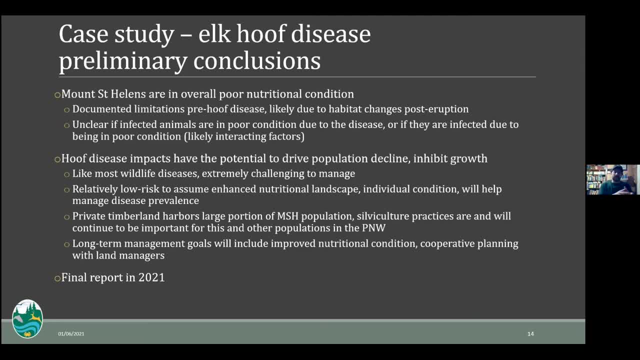 and then the post-boom sort of feedback: overshooting carrying capacity. It's not entirely clear whether the infected animals we see that. you know. does the disease infect an animal because it's in poor body condition? Does an animal that's in poor body condition? 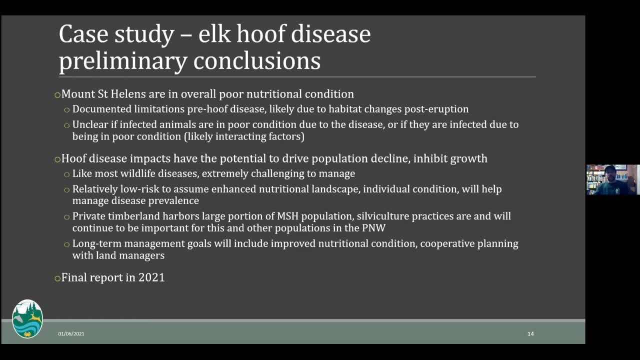 contract the disease or are they interacting? It's a bit of a chicken or the egg question, but I do think that, based on what we've seen, you know we have background nutritional limitations. an animal contracts this disease and it's even poor. 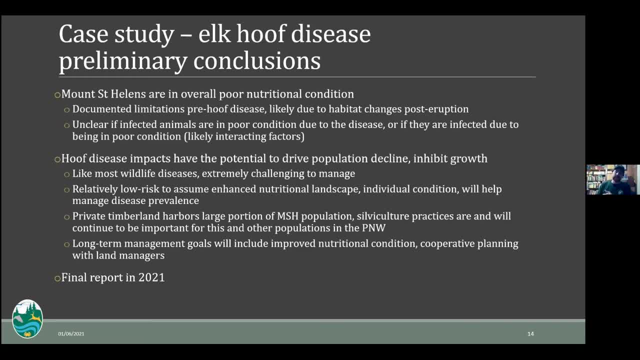 it's an even poorer condition and we don't see that really. in some of the other areas where maybe we have elk populations that are in better condition, Hoof disease impacts might have the potential to drive the population decline. We're teasing some of that out with this analysis. 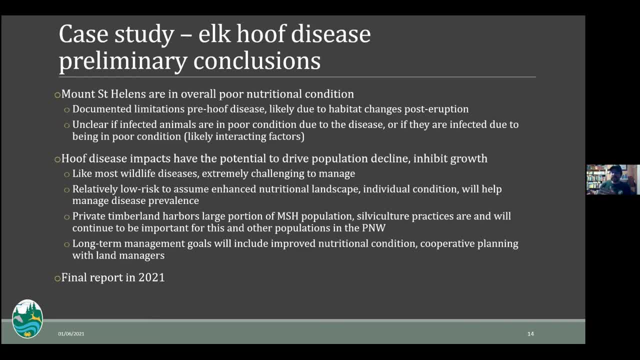 and you know, inhibit the future growth of this population. But unfortunately most wildlife diseases, and especially hoof disease, are extremely challenging to manage. There's really unfortunately there's no silver bullet, there's no magic solution, there's nothing we can really go out there, and you know. 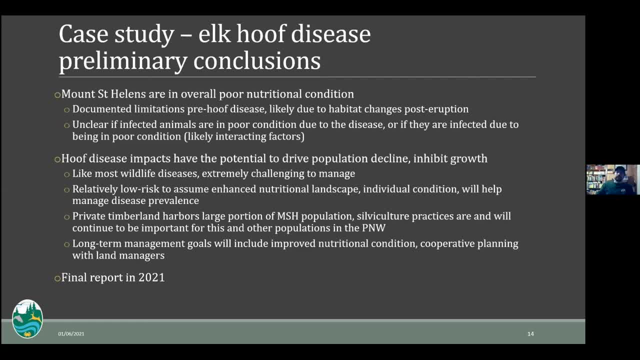 we would have done it if we could have, but unfortunately it's here to stay and we have to learn how to manage it. And it's, I think, relatively low risk to assume that if we're able to enhance the nutritional landscape or enhance the individual condition of animals, 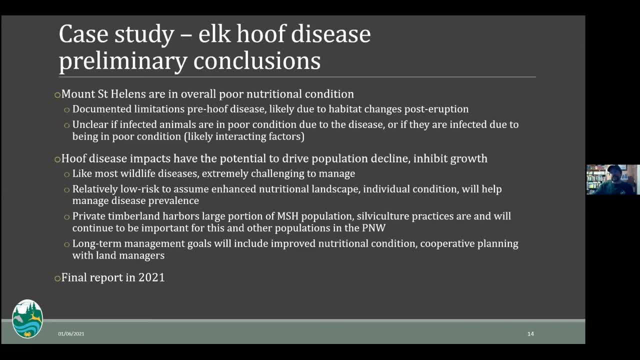 and the overall population level of condition, we may be better off in terms of managing this disease. Animals, that is to say, the sort of animals in better condition, better body fat going into fall, not only do they have better outcomes for pregnancy, 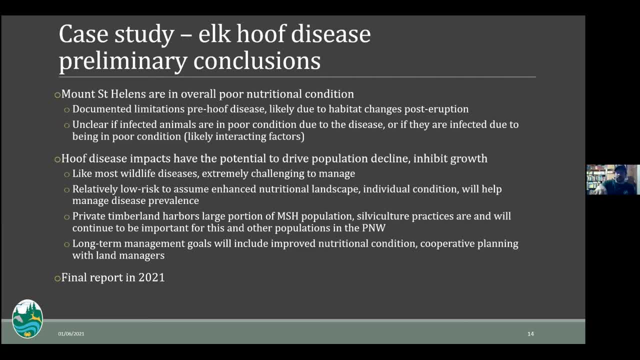 and survival and recruitment and those important factors for growth of the population. but it also may stem off the infection from becoming infected or it may help them from achieving really severe stages of the disease where it's maintained more at an early stage. Some of that's played out a little bit. 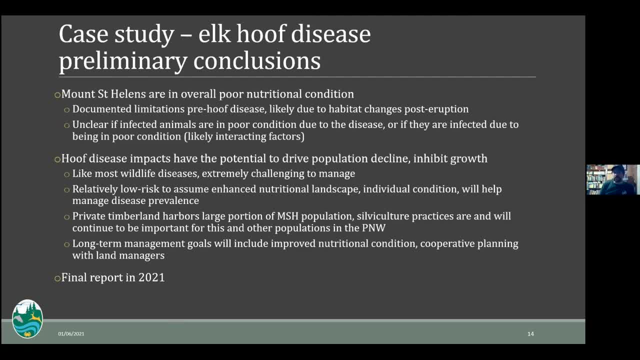 in the domestic livestock literature and, I think, something that will probably hopefully learn more about. you know, as we move forward with a lot of the research programs that are going on with hoof disease, Private timberland harbors a large portion of the Mount St Helens Elk population. 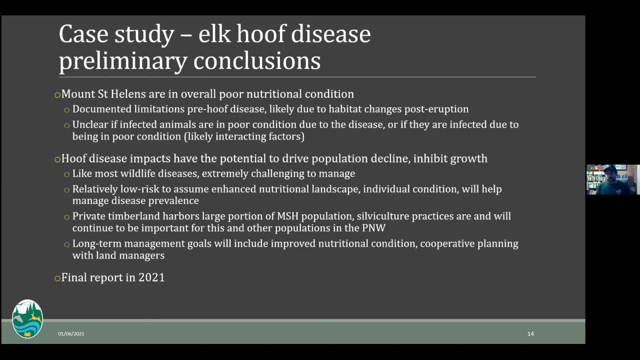 and is therefore, you know, really important. Those silvicultural practices, forest management practices, are really important for this population And of course we zoom out and they're, you know, these silvicultural practices are really important for drivers for elk across this region. 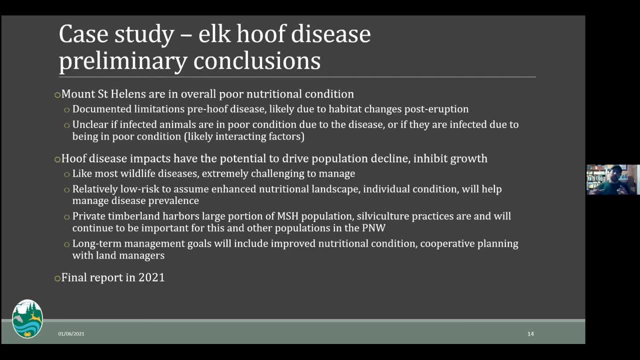 the Intermountain West and the Pacific Northwest, And that you know when I think about kind of long-term goals. you know as elk management and department managers, these populations, you know we really have to think critically about integrating nutrition here. 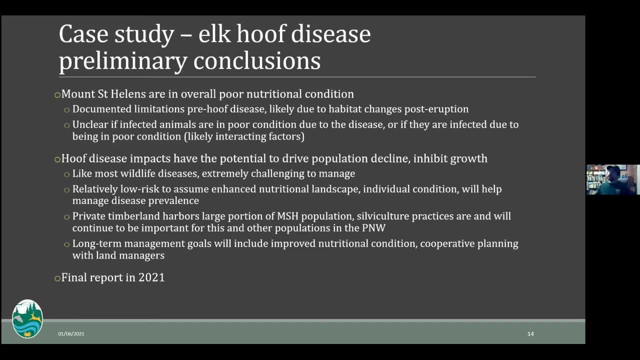 and working with our cooperators- land managers and in a partnership, to try to be strategic about, you know, growing good elk habitat, achieving multiple independent objectives, finding that nexus where we all kind of win and we have good elk populations. So that's what I'm working on now. 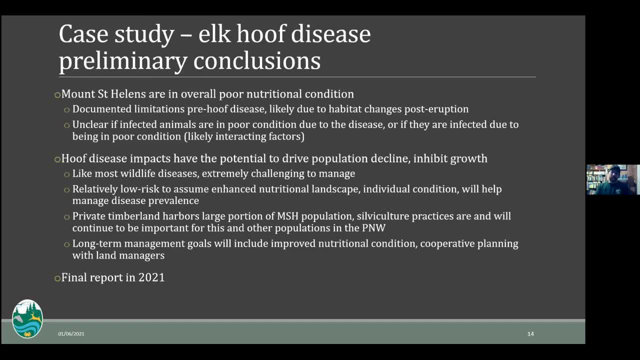 Thank you And wrapping up this analysis, wrapping up this report. it's due in 2021 and I'm eager to have it out there and have folks be able to consume that information. So with that, here's some additional resources about hoof disease specifically. 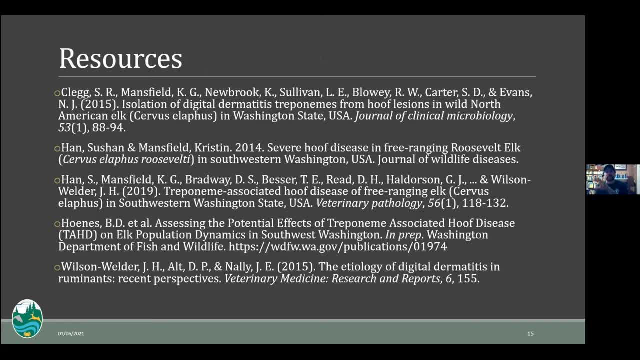 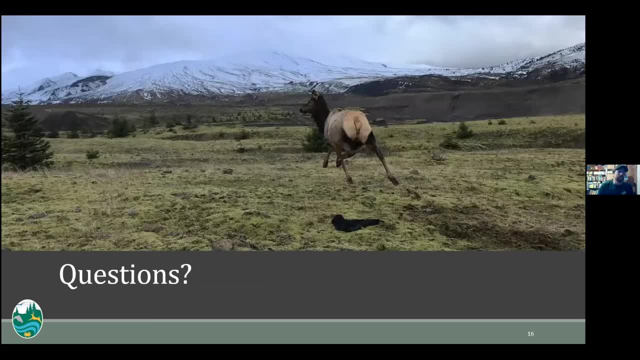 We can show this presentation so you folks can see those And hopefully we have some time for questions And I'll hand it over to you, Paula, Thank you. So we do have a question. So if any of you do have a question, 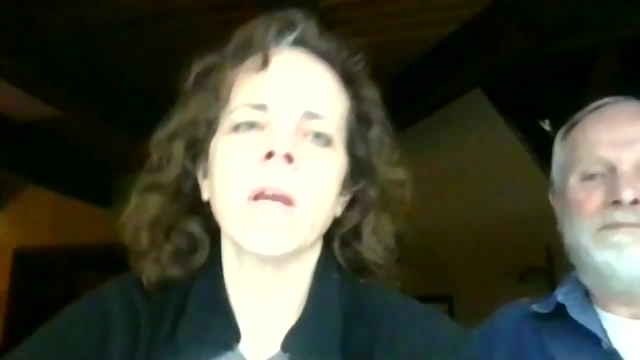 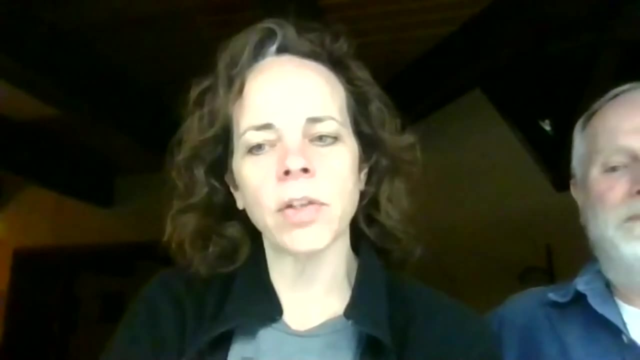 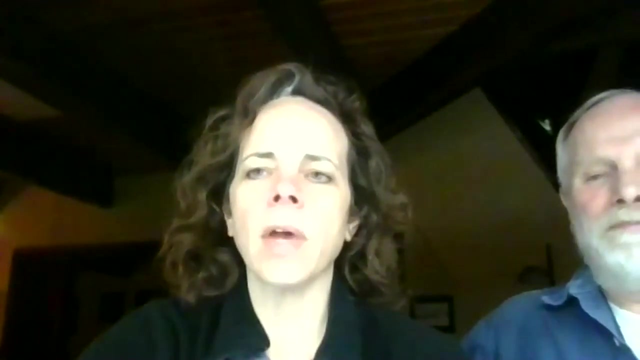 since we do have 30 plus people on here, if you could just type them in the chat and then I will ask Kyle them. So Bill asks for the body fat slide with the hoof disease. what month of the year was the data taken? Early lactation June to July. No, those were taken in December, So they're already. we're probably already seeing those estimates are a little bit lower than what you would expect to see. you know October, And certainly so that peak that we find. 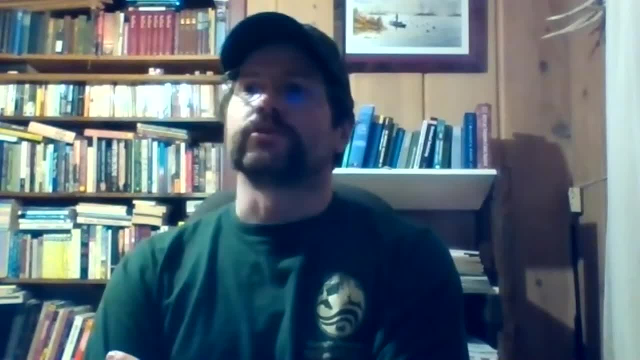 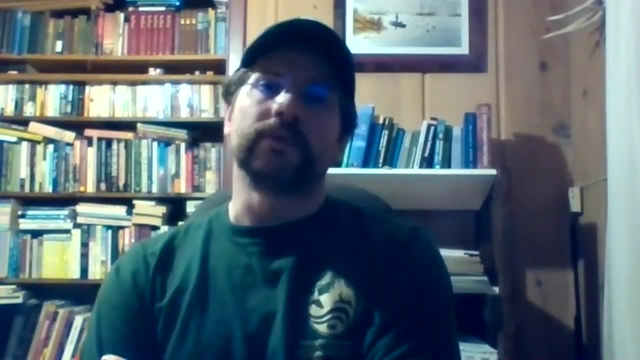 in August or September. The majority of elk we captured in December mid to, sort of you know, late December. And then we did have our first capture was in February. but I don't present those data because the you know the body condition. 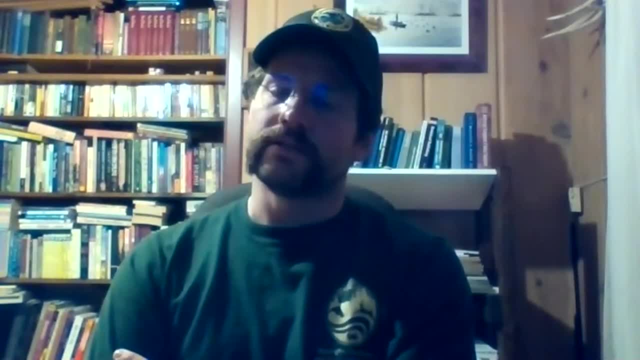 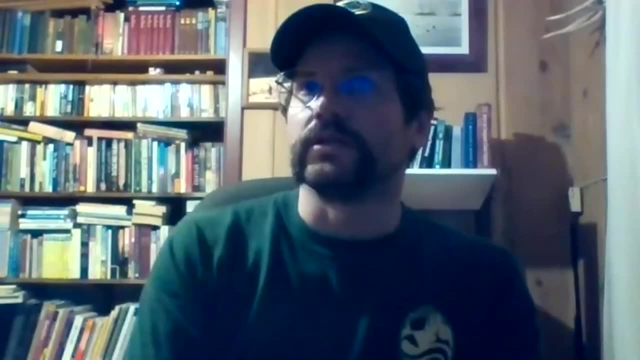 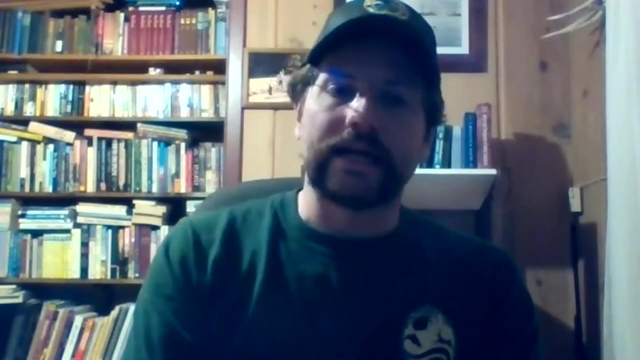 that you're seeing in February. you know you can't really bend that with body conditions. you see in December as well, And so the lactation- all those estimates are coming from December. Lactation is not necessarily that the animal is still nursing, but you can palpate. 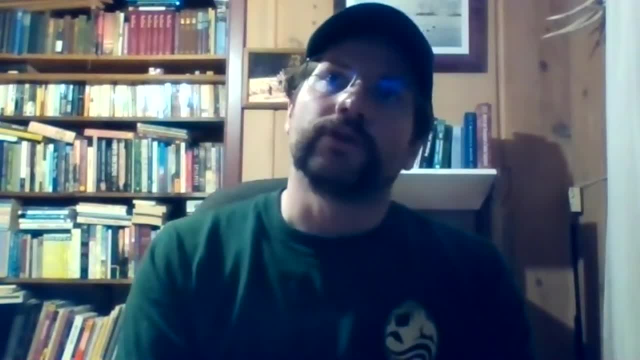 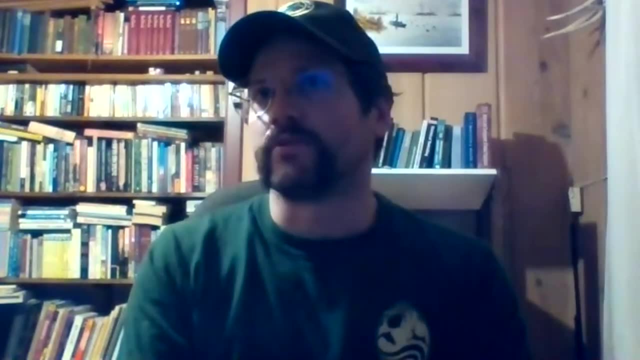 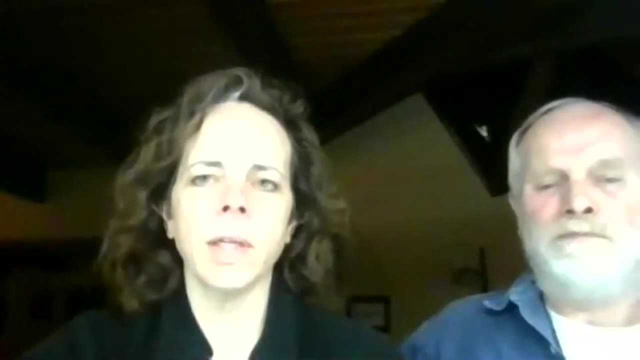 and see that they were actively nursing a calf that summer and into the fall. I got a little bit of information. Okay, anyone else have any other questions? I don't see anything coming through If some of you haven't done zoom before. 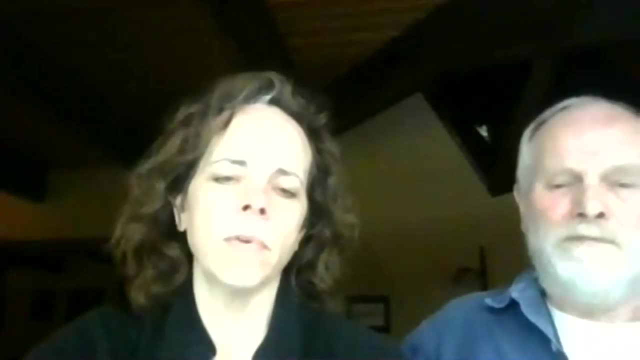 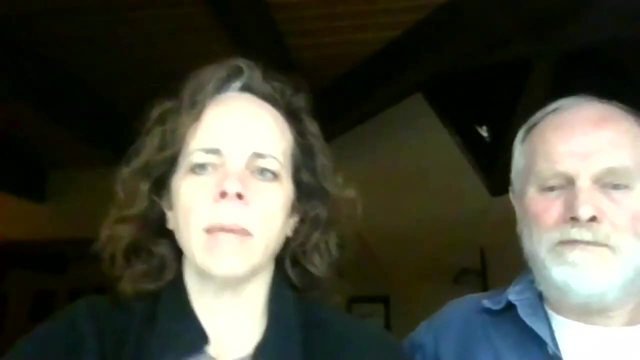 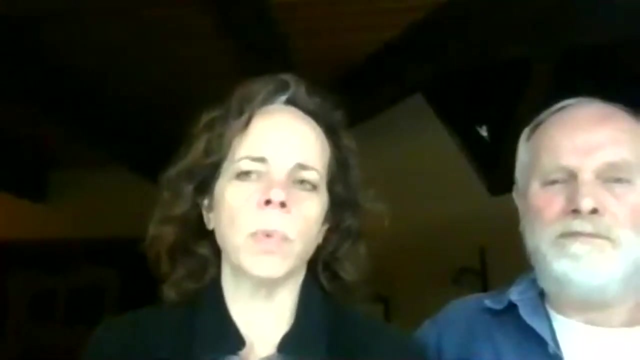 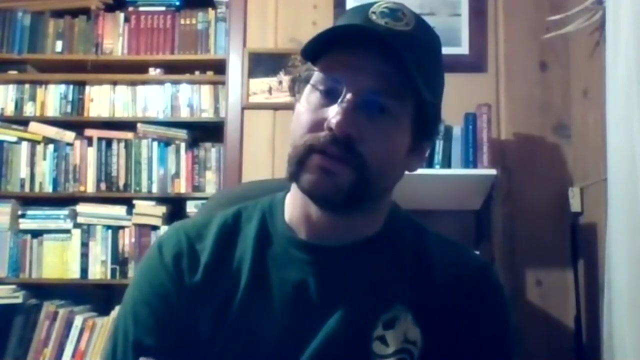 if you take your cursor to the bottom of the screen you'll see a little chat box and then you could type it in there. So Judy asked: do we know how the disease is spread? good answer for you that would be: you know definitive and and you know leave. 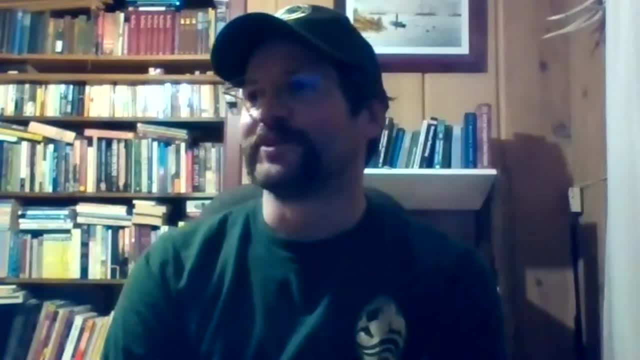 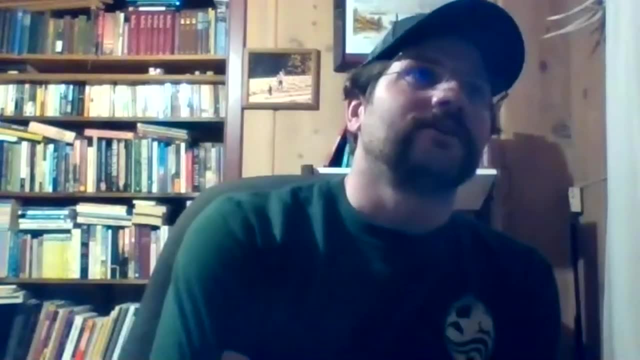 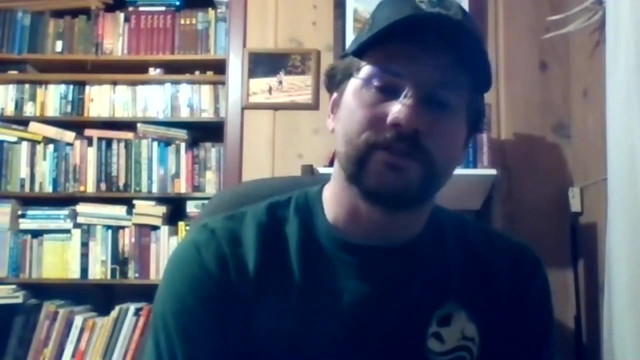 us all very satisfied with knowing how it does move around. we don't know. you know it, dr Martin- while that at Washington State University has a very sophisticated research program where they have elk that are in captivity and they're trying to learn more about how the disease is spread. I mean, they're 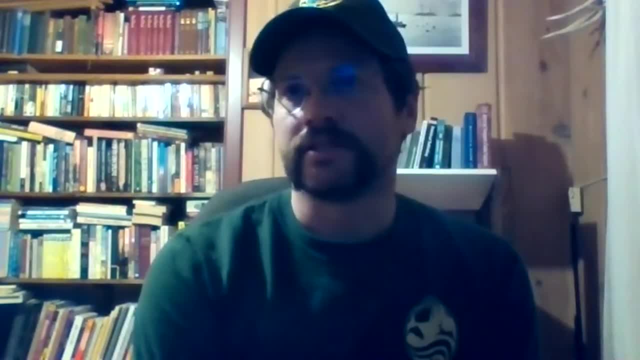 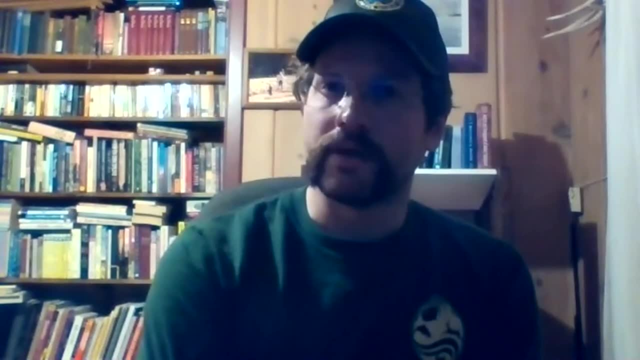 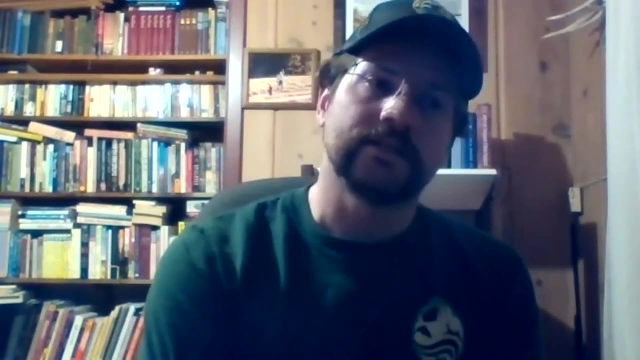 they're trying to learn. you know fundamental but extremely important to get the fundamentals on. you know how, how does an animal contract the disease, what bacteria are there and necessary to contract the disease, and also you know how is it transmitted. I I don't want to speak for dr Wilde's program and her 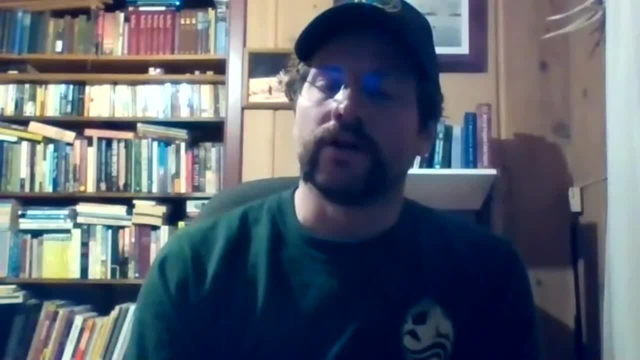 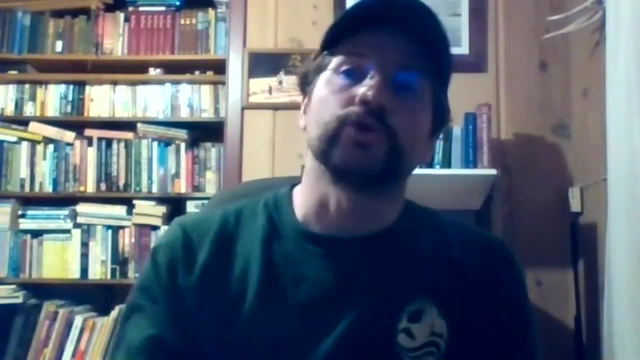 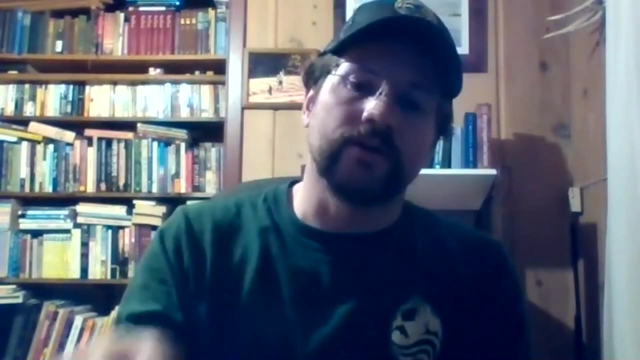 research, because I don't want to, you know, inadvertently mischaracterize any of their research plans. that is to say, though, that you know it's worthy of checking out their web page. I got a great web page, and their research is really exciting, but the disease is is bacterial, and it has the exact almost 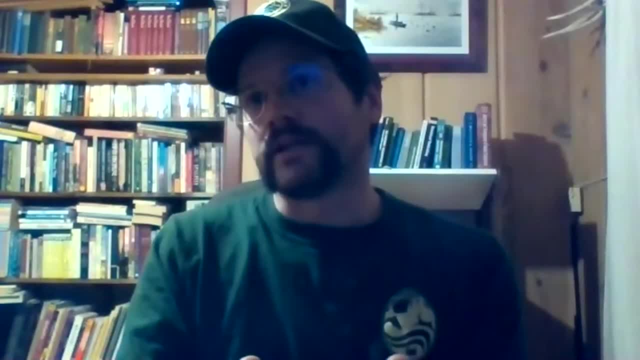 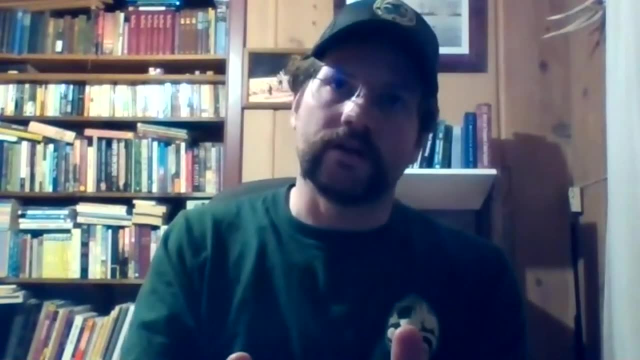 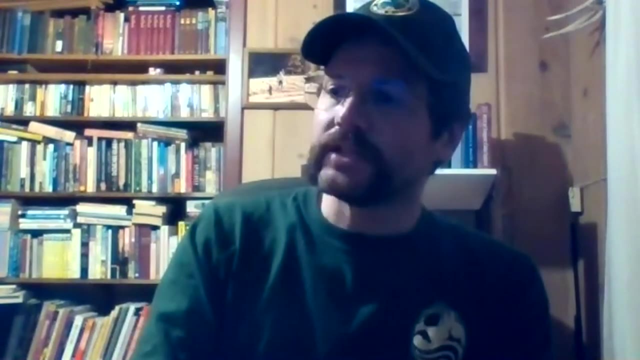 the exact same microbial profile that we see in a disease of domestic livestock. it's called digital dermatitis or hairy heel wart or raspberry heel. it's pretty common in dairy systems. there's a little bit more research has happened there on trying to understand the disease and how it's been trained, how it gets transmitted and it. 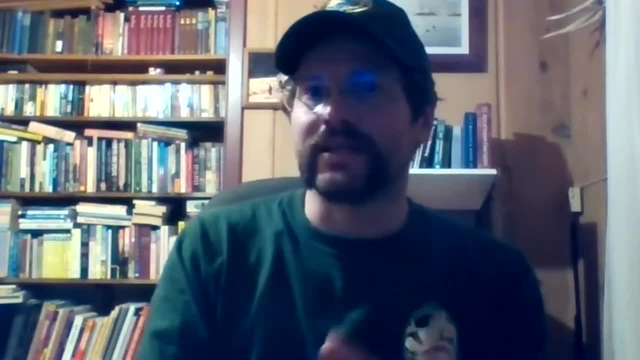 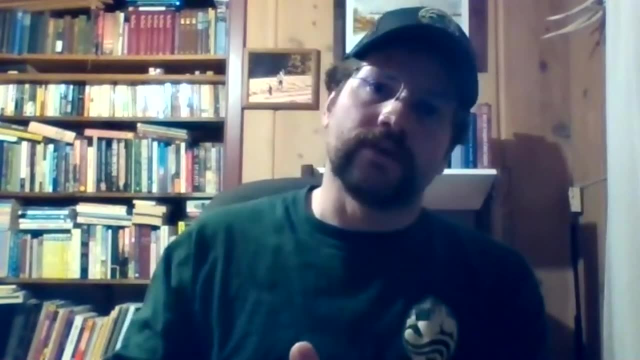 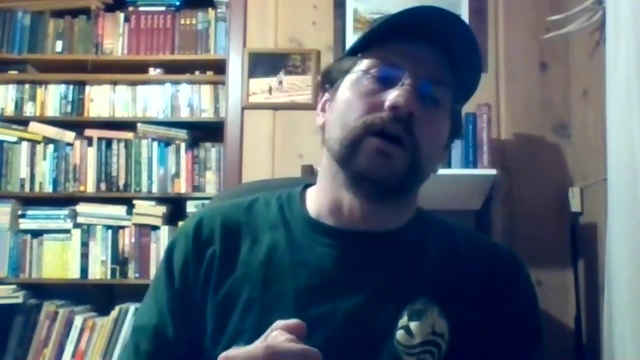 seems like there's pretty good evidence that it's transmitted often through the environment, and so in a dairy system that would be through the, the slurry, the mud and the water and the urine. you know, it's sort of a great breeding. you know broth for for bacteria to grow in, and so and you have an infected cow and 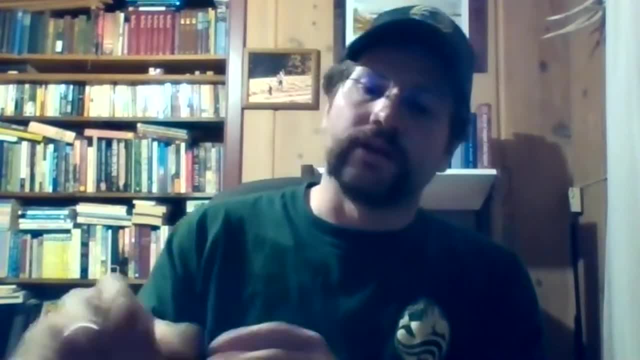 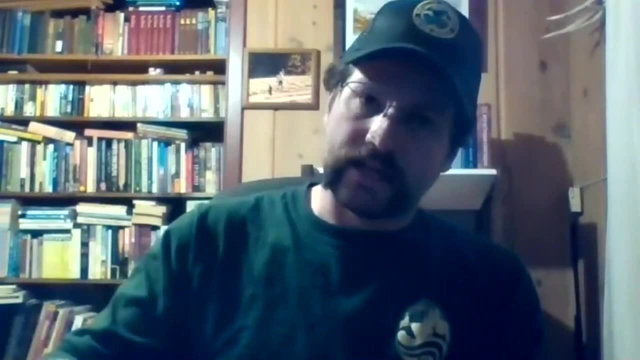 you have an infected animal and you've got a cow and it's it's shedding the bacteria into that system, into that environment, and then an uninfected animal encounters it by just taking the hoof step down. so we could speculate that that's how it also transmits an elk and I think that that makes a lot of. sense but there's a lot of questions on. you know, does it take? you know pre-existing factors. you know elk walk in really rough areas. they have little micro puncture wounds um. from dairy research, domestic livestock research that is often brought up is that these animals? are in constantly wet conditions and you know, just like you sit in a bathtub too long, your skin gets soft and it's called maceration, and and so that might allow. being in really wet, moist conditions constantly might allow bacteria to invade tissues and skin and they otherwise wouldn't be able to. 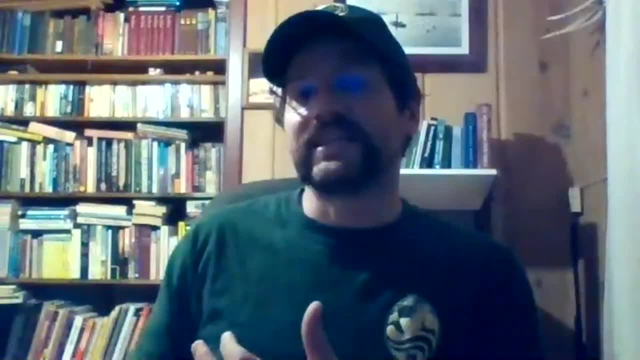 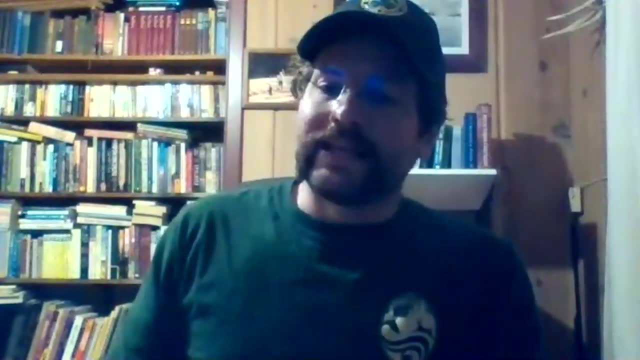 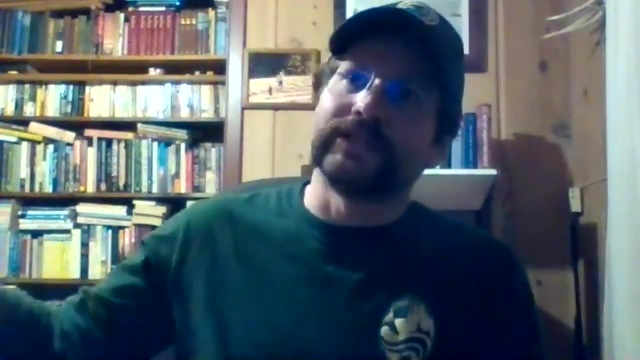 or at least allow initiating bacteria to get on there. but um and that that that felt good to to say that. you know, before we started seeing the disease and in the blue, you know, we, we detected it in the blue mountains outside walla walla. it's been detected in large and pretty large. 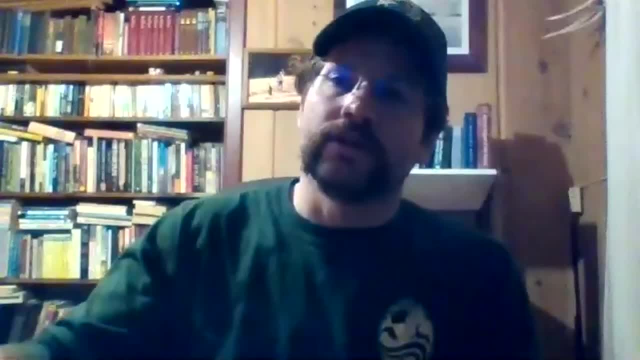 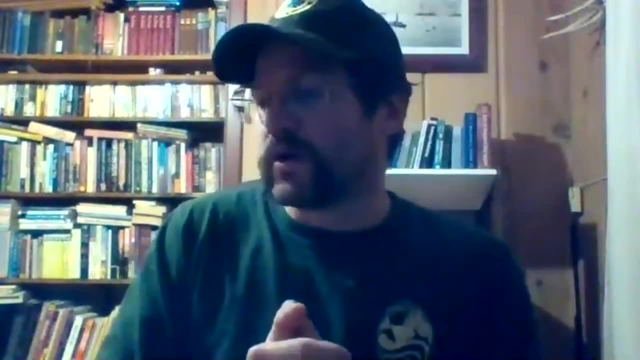 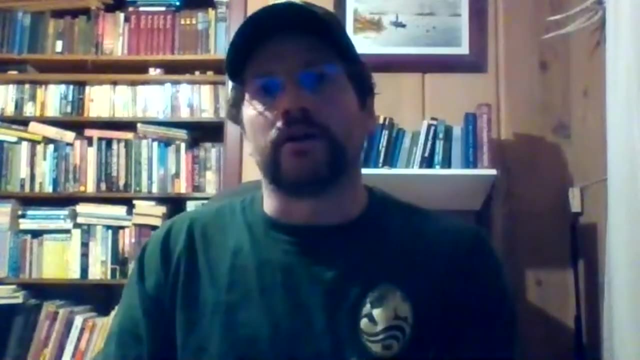 geographic areas of idaho, uh, oregon and now northern california, which is, you know, pretty wet place too. but i think that that still makes sense. but i think there's just a lot going on here in this disease process, you know, and there's a lot of bacteria involved and some of them maybe 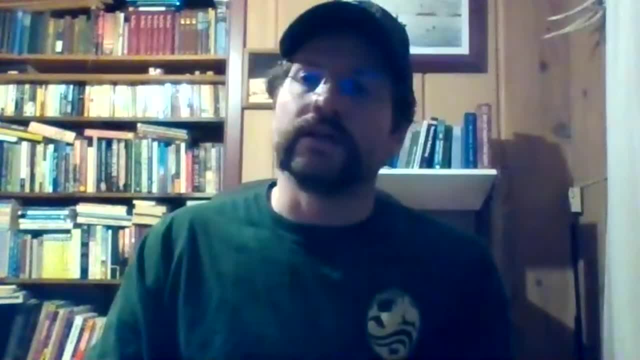 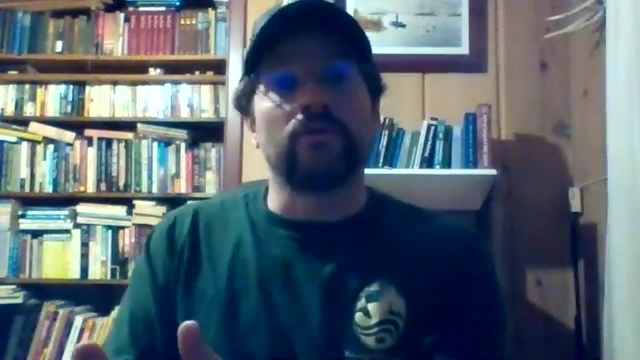 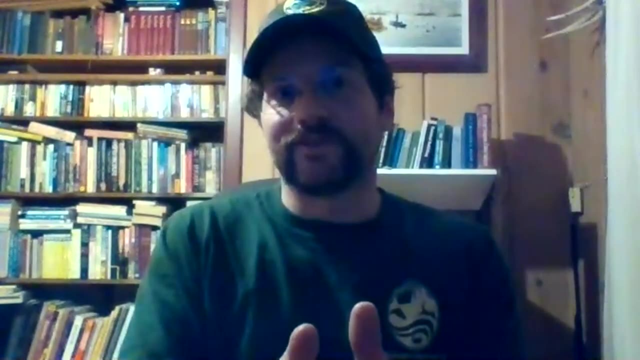 initiate, play good, important roles in the initiation of the disease and then not play a role anymore as a, as other bacteria um take advantage of that, initiating microclimate in in the tissues and then invade deeper tissues. so a lot to learn um, and another thing too, i think. 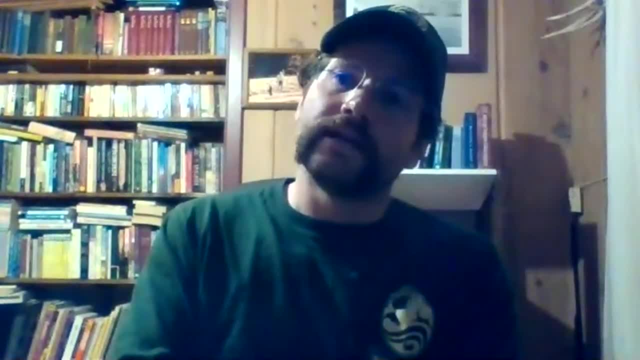 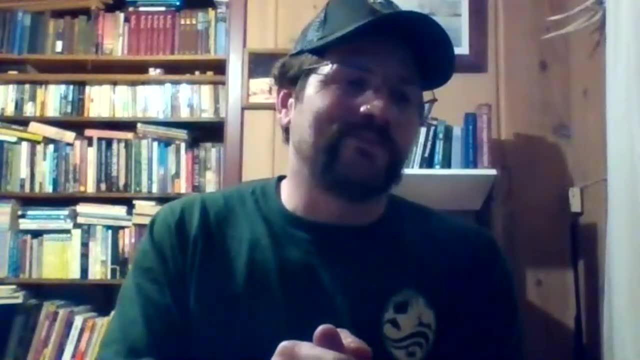 that you know, we we don't know how it spreads, but i i feel pretty comfortable saying that it isn't just elk moving the disease around. um, maybe it went from elk to elk and willapa hills and elk to elk jumping over i-5 into the mount st helens. 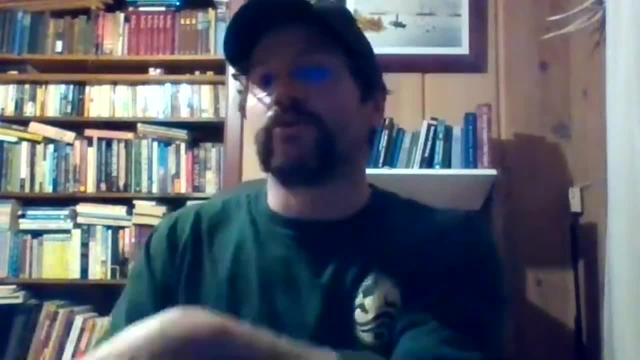 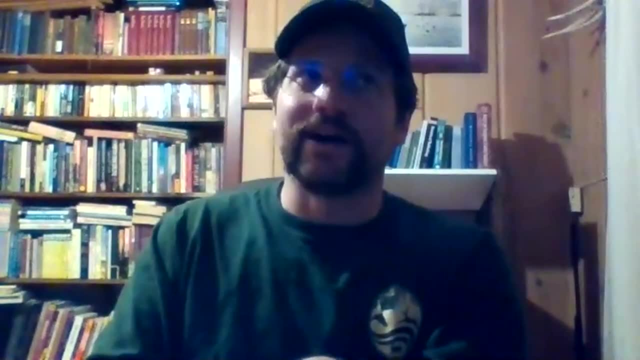 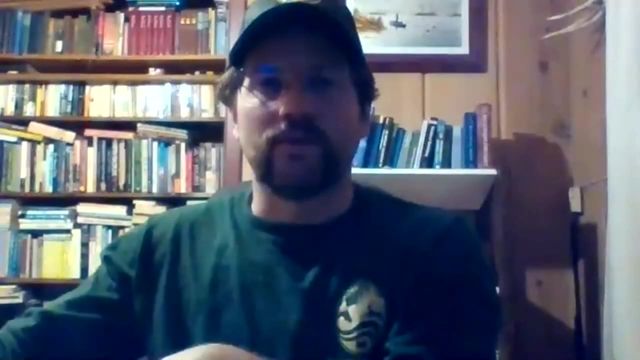 population. that makes sense. uh. what doesn't make as much sense? uh, how it got from mount st helens and trout lake to outside of walla walla in the blue mountains of washington- pretty big sort of dead zone there. so something else is probably going on, you know, and it's, and it may be human mediated. 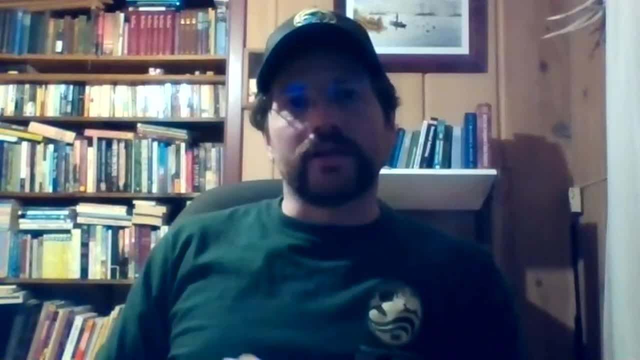 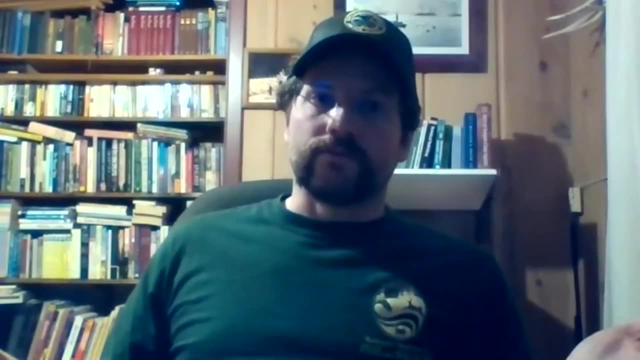 um, it may be. it may frankly be spillovers from domestic livestock reservoirs, where you know the disease in domestic livestock is present. i mean it's ubiquitous in the dairy systems, um, you know, and causes it's a major cause of lameness in dairy. so we don't know. um we have some ideas. 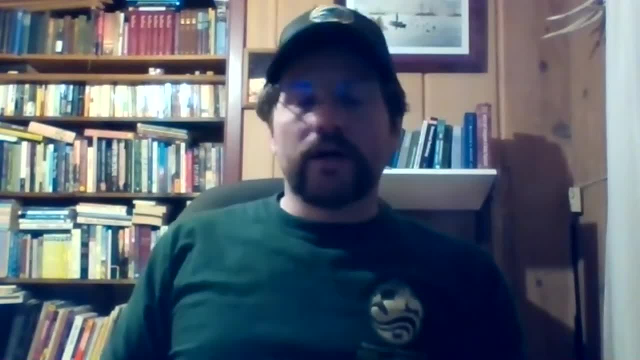 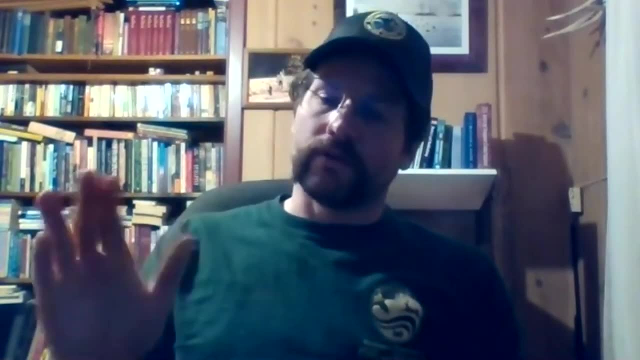 and unfortunately there's not a great solution. you know we don't know how to do it, but i think you know interrupting transmission would be a great solution to managing the disease. but we haven't quite figured that out yet outside of, if you have, you know, the common sense thing. 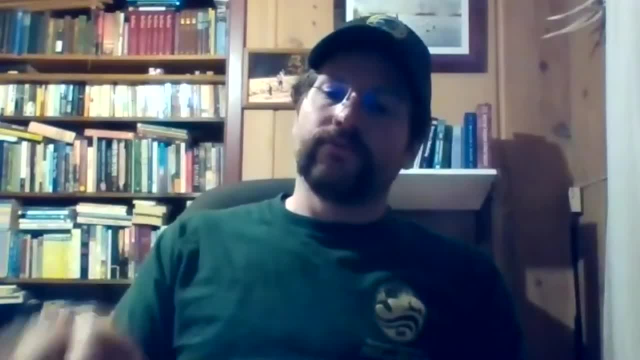 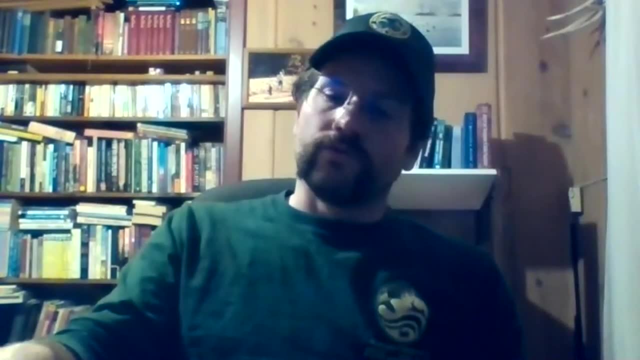 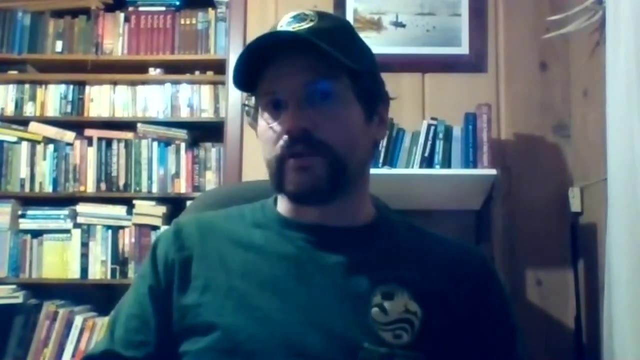 of an animal is sick and it's depositing these bacteria into the environment. if you could remove that animal quicker, um, it may shed less and therefore it may infect fewer people. um, you know, i think it's interesting. now, with covet 19, a lot of us know a lot more about disease spread and. 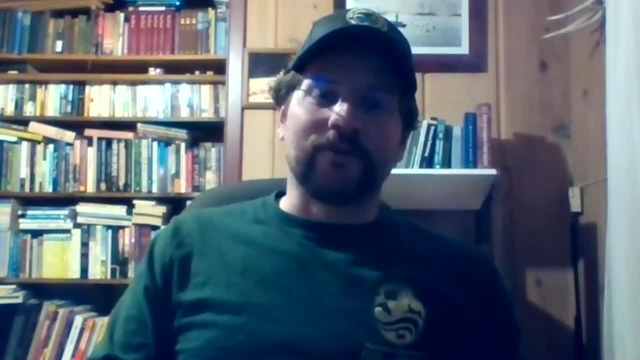 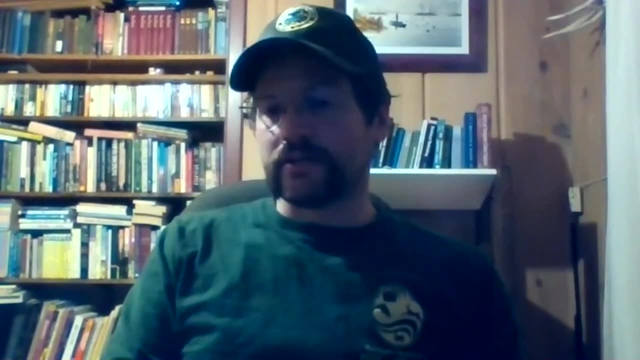 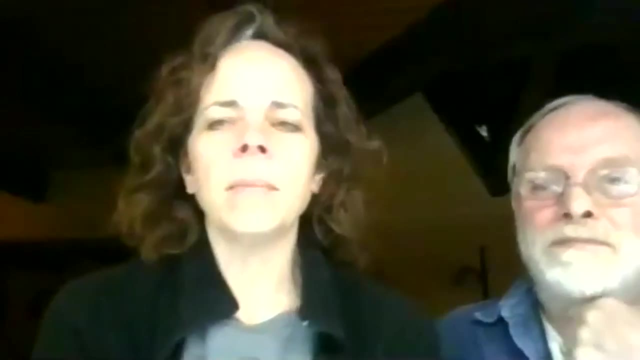 transmission, interrupt, that kind of stuff, and so a lot of the similar concepts apply here. but um, you know, we we don't entirely know. so okay, um a couple of questions from rick, so i'll ask them each individually. um, his first was: um was the 1970s reduction of harvesting in the federal 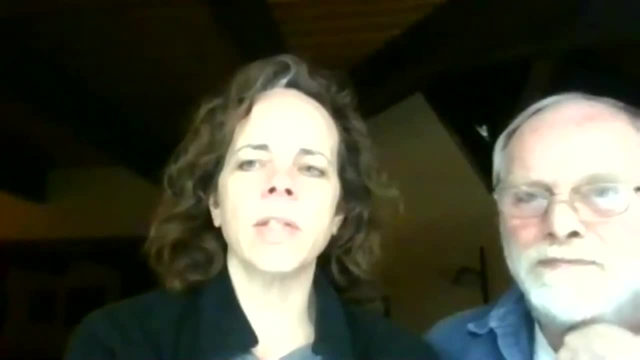 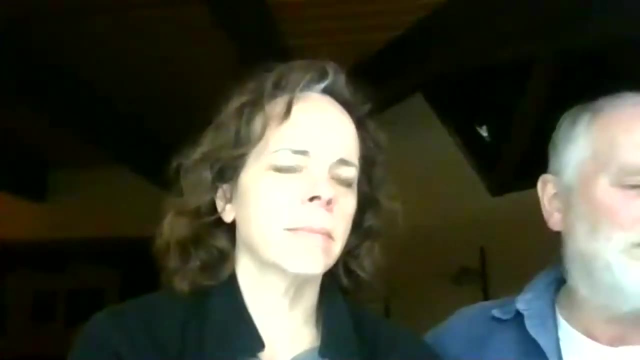 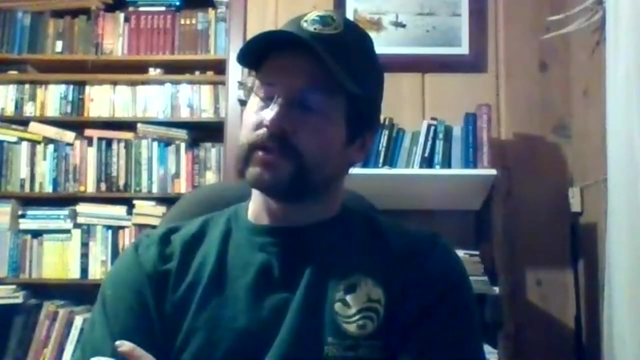 forest part of the problem limiting elk browse. well, i'll be honest, i don't know a lot about um forest management. you know- real, you know- a lot of details about forest management in the 70s. um i know a little bit more about it in the 90s when we started to. 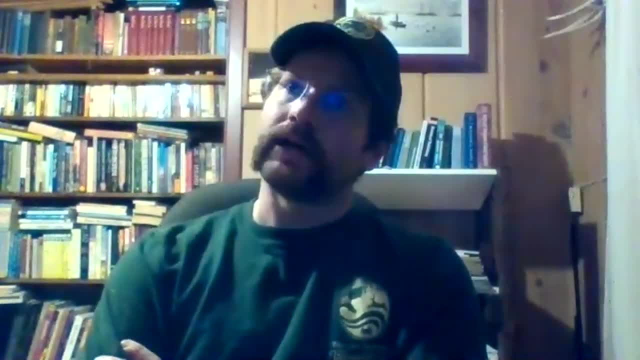 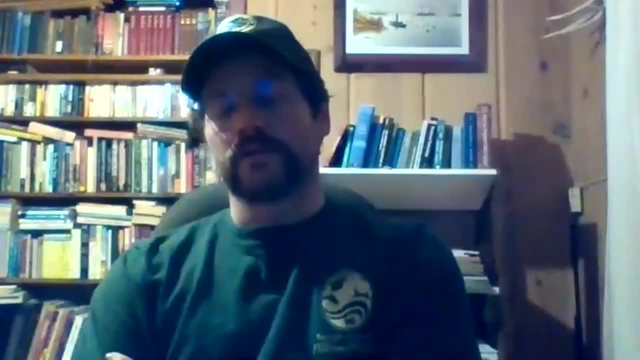 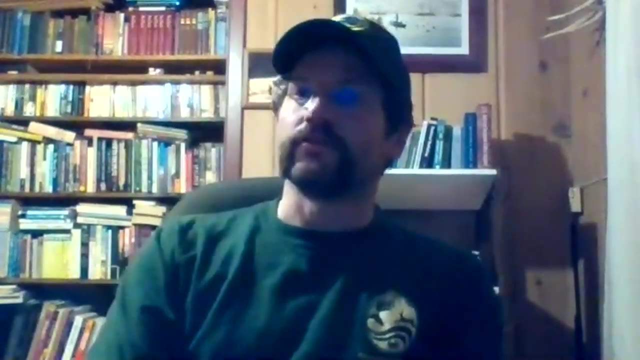 see reductions in the activity due to this sort of the force. you know the the national level force management plan and the reactions to, you know, concerns over spotted owls, marvin mirror was that kind of stuff, but um, yes, i mean i think that you know we're seeing across the board. 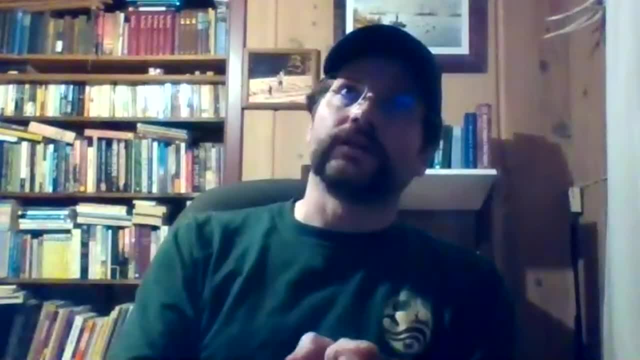 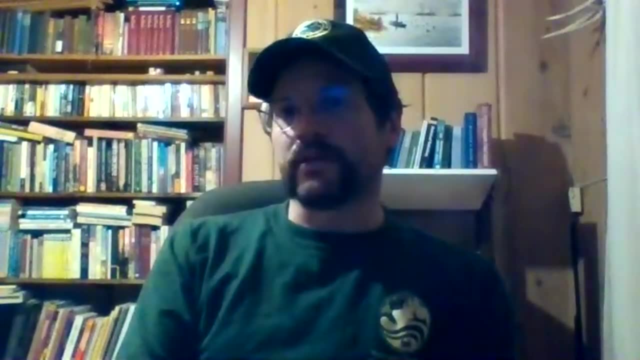 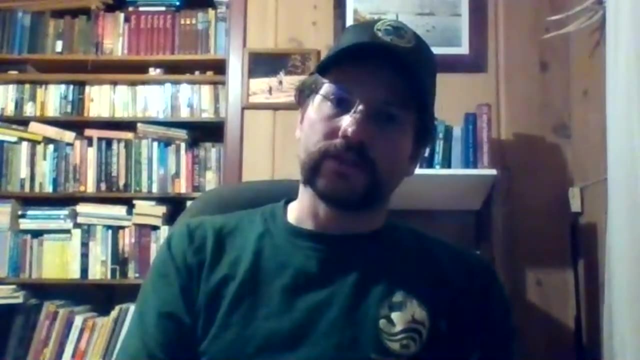 where we have reduced active timber management and harvest happening um on large tracts of land and that, you know, kind of usually means the the federal forest system um that we're seeing less habitat be create, forage habitat being created and therefore there's just sort of feedback that 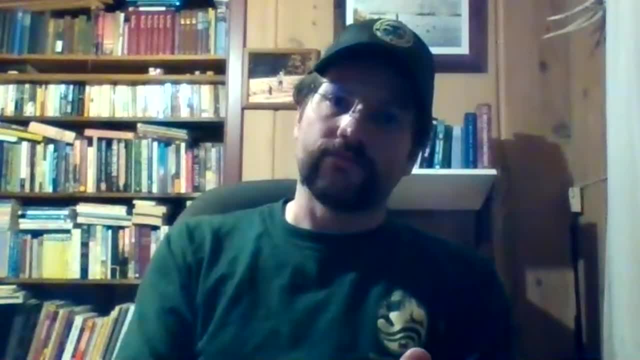 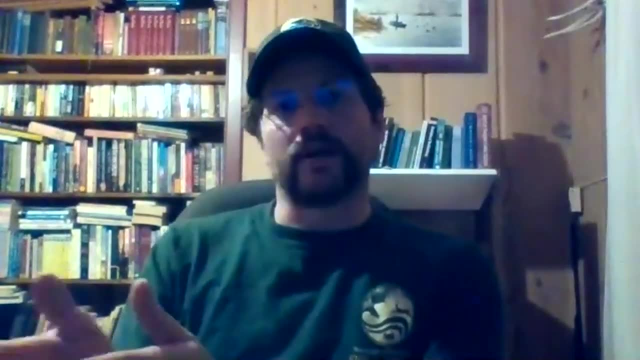 you know it's just: you've, you've got a. you have to stay on top of it. you have to. you know, the the forest gets older and so you have to constantly be kind of resetting the, the, the, the, the, the, that, that forage window, that serial window for elk. so yeah, i don't know if i can answer that. 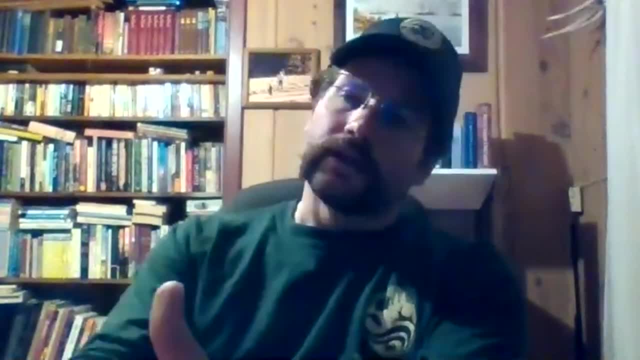 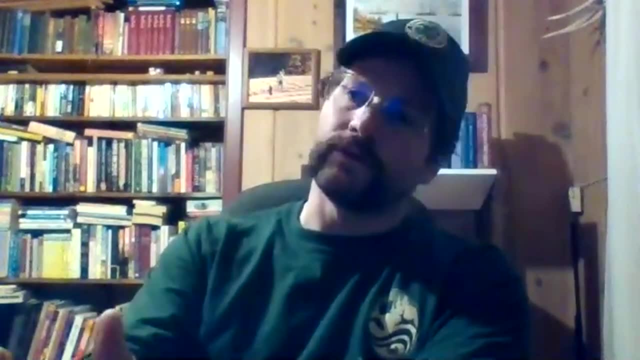 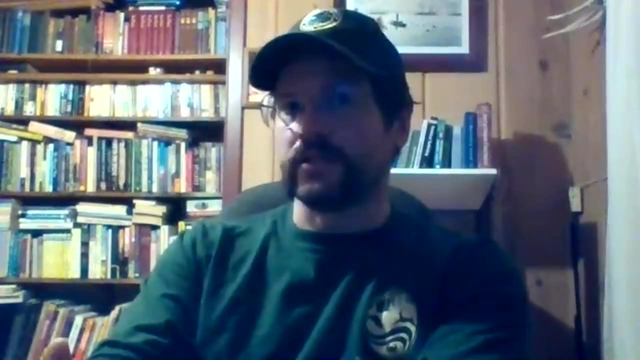 question specifically, but i would say that in broad principles, you know, if, if there isn't very much active forestry and we're seeing um closing of canopies, then we're probably seeing, you know, negative consequences for elk forage. um, you know, again outside of like waiting for a few hundred. 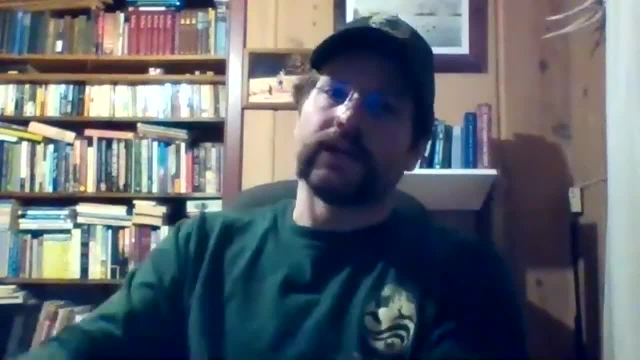 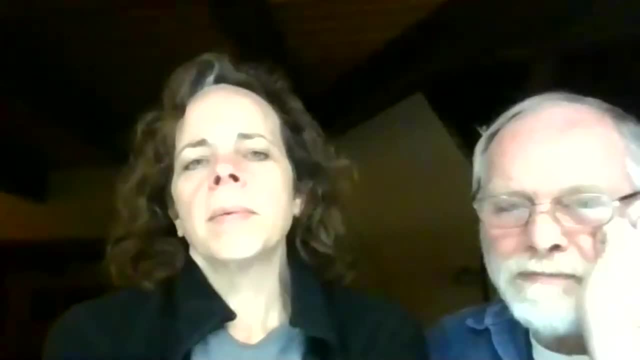 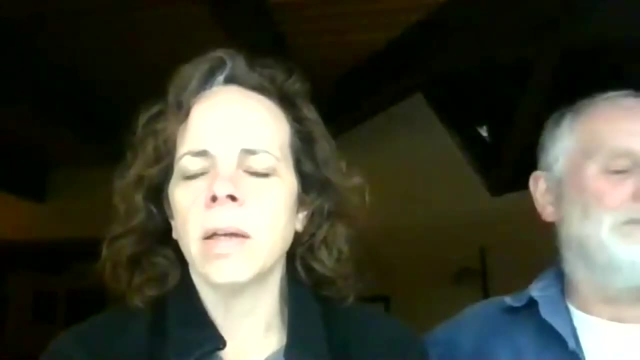 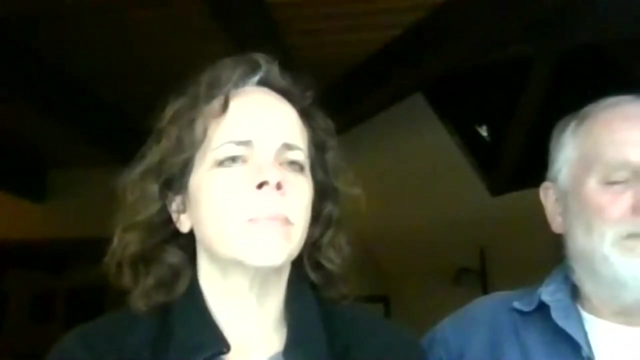 years for old growth to establish, and then that's a different story, but we're, yeah, that's reality anymore. so, okay, um. his second question: um, is there an elk disease that has developed in concentrated herds, like jackson hole? impacted our washington herds? well, uh, no, nothing that you wouldn't consider like a normal disease of of elk, something sort. 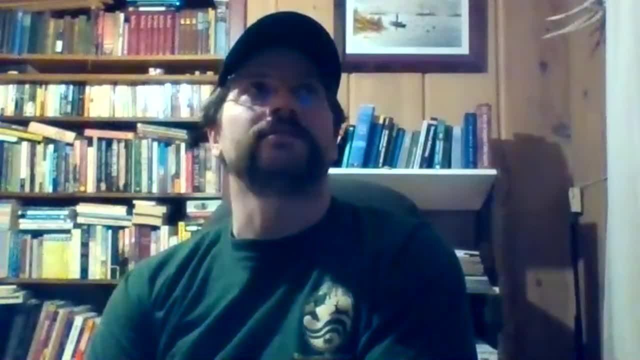 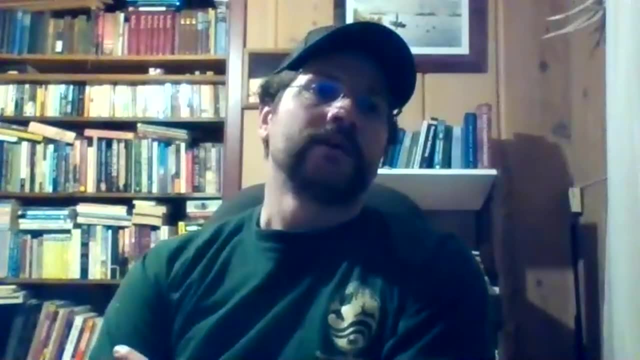 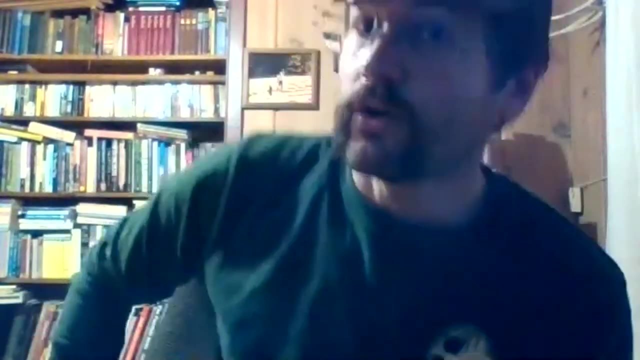 of normally naturally occurring, or something like you know, parasites. um, we are extremely lucky uh, so far to date that we do not have chronic wasting disease. um, we don't have uh brucellosis concerns, um, and those are kind of the the main ones that i would. 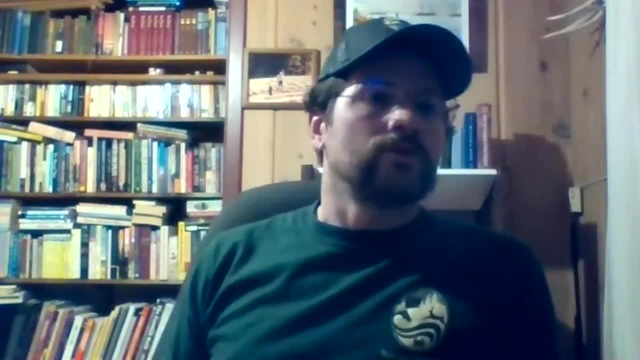 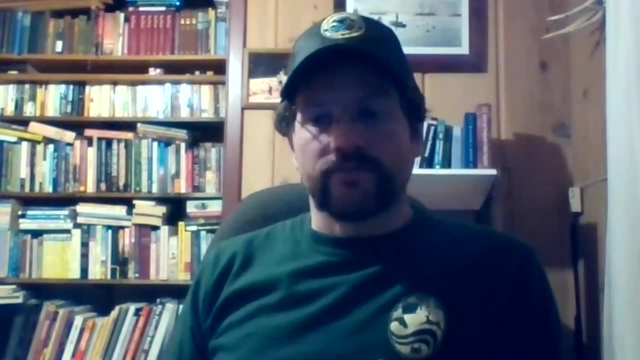 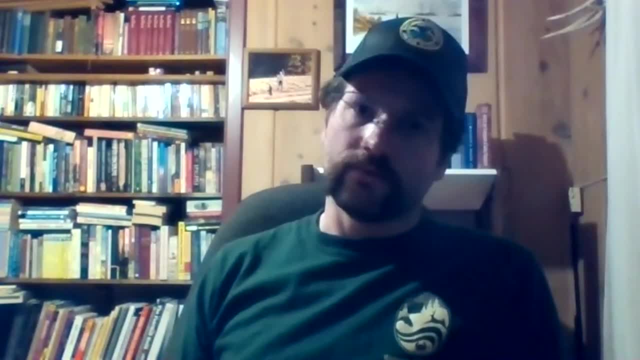 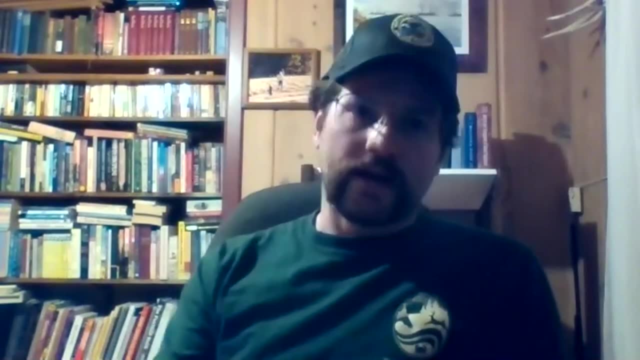 incredibly, extremely difficult to manage and- and we're. it's unfortunate we have elk disease and many other places now do as well, but we are. there's maybe a silver lining and we don't have hoof disease and chronic wasting disease. and i'm going to knock on wood, i'm not a superstitious. 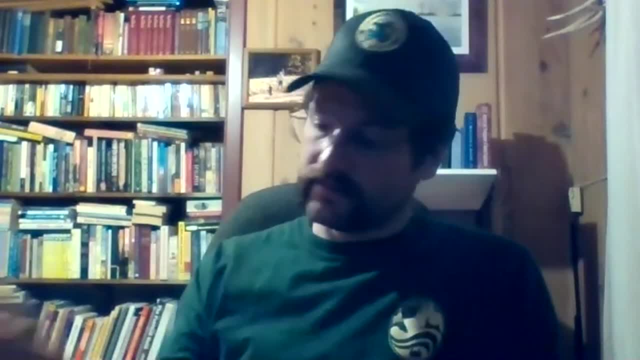 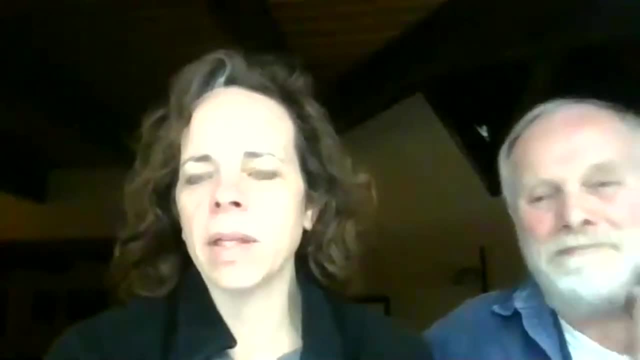 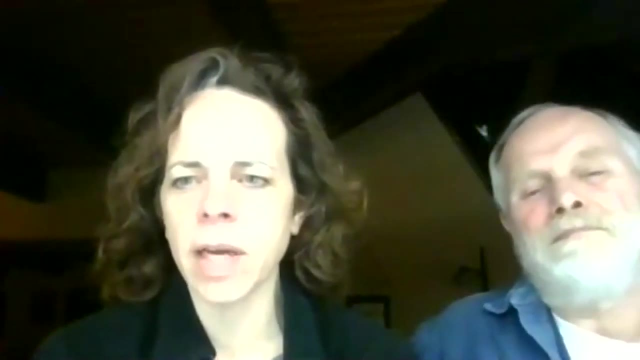 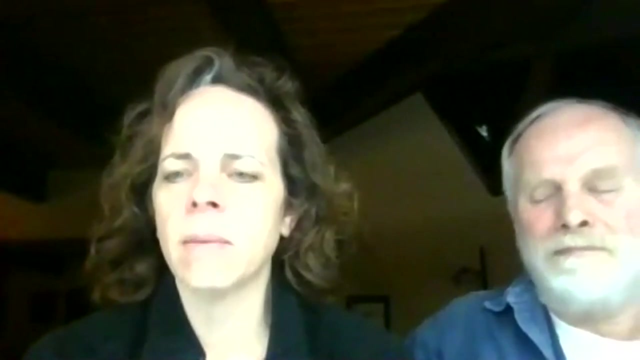 person um from bill uh. he says your summary slide regarding drawbacks, including roads and herbicides. previous slides showed benefit in quality and safety and i'm really looking forward to seeing and abundance after one to two years. this doesn't take into account the benefit to the establishment and growth: benefit to tree establishment and grow. 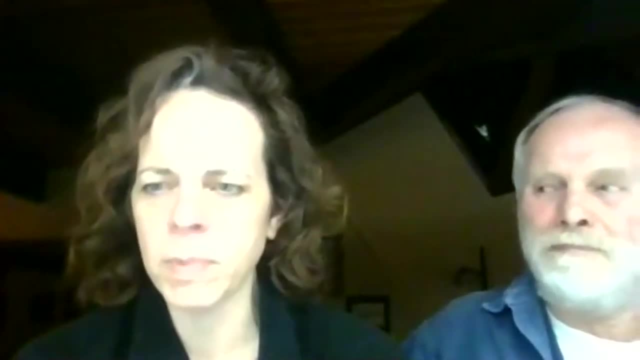 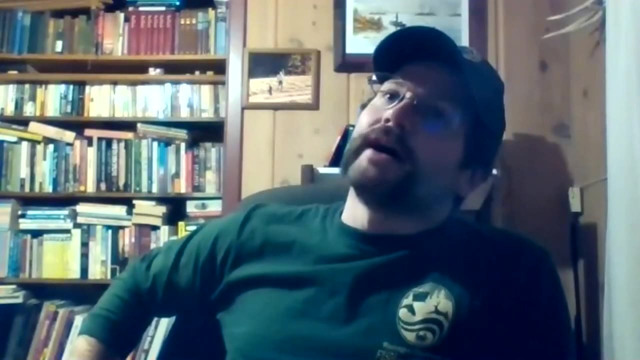 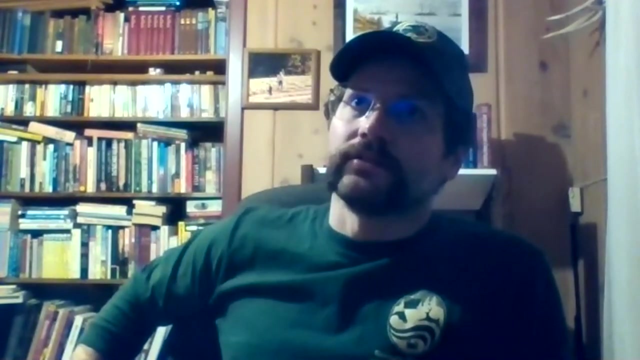 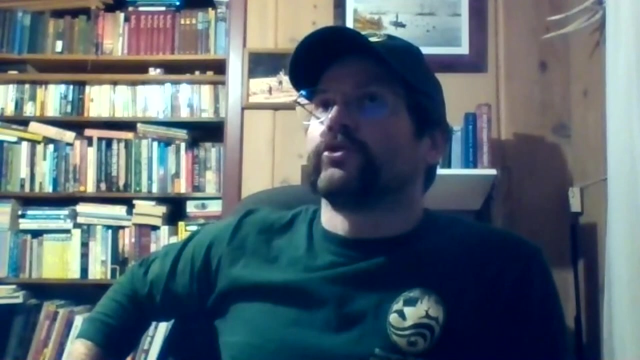 sorry, certainly so, yes, so I'm. my thinking is biased and and anchored by more of what's good for elk and not necessarily, you know, I'm not necessarily thinking of what's better for, you know, growing trees. so it's, it's um, you know the there are drawbacks of herbicides from a elk forage perspective, and but 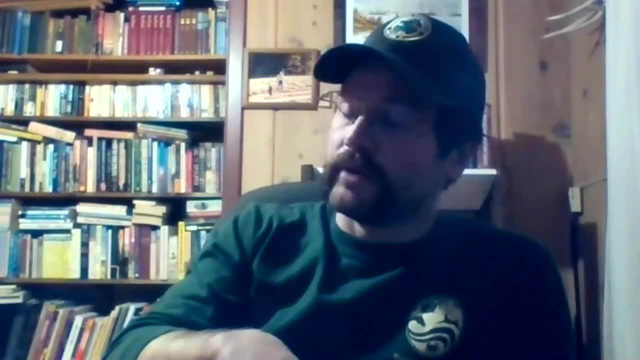 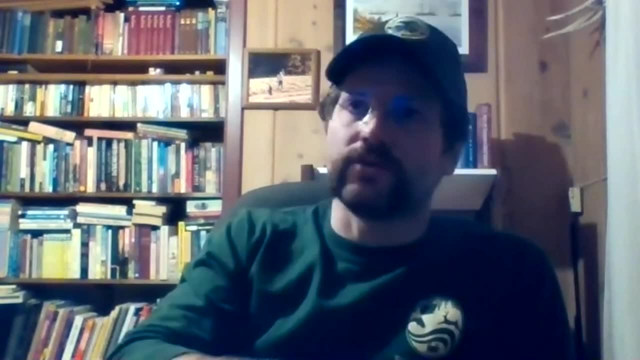 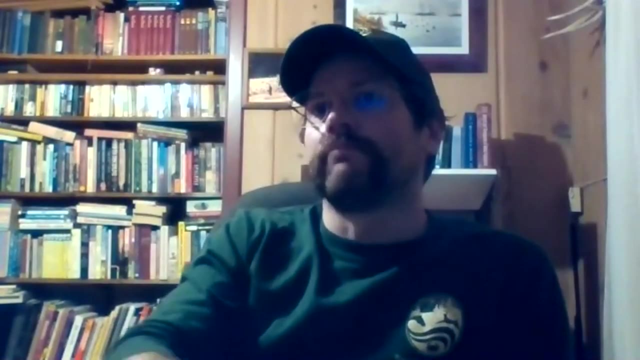 those drawbacks are short-lived, you know, and and there's even complication there because you know herbicides may affect composition of forage species that are out there. that's masked a little bit by uh yeah, and so um discussion of the amount of biomass is out there and again I said that plant species aren't created. 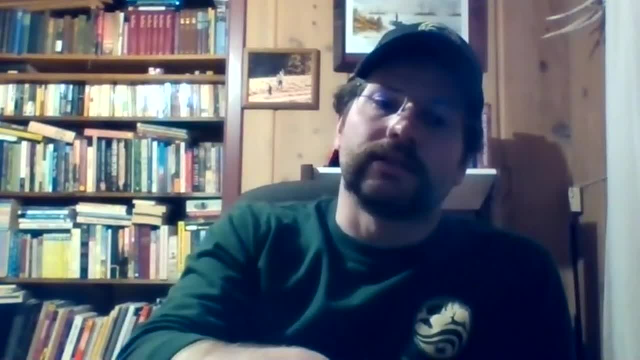 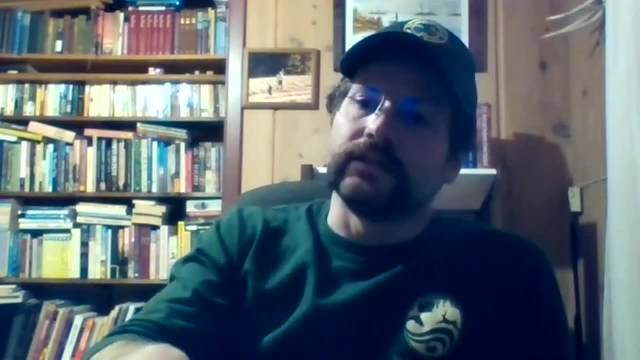 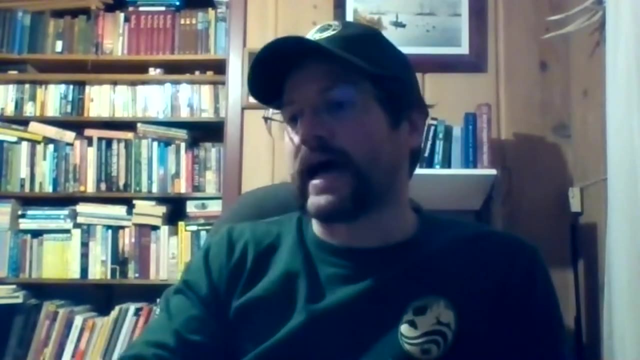 equal in their nutritional value to elk. so it's possible that you might see long-term changes in composition that might not be good for elk and might last for the whole early cereal period. but overall, you know, there's still that benefit of you know stand level disturbance. 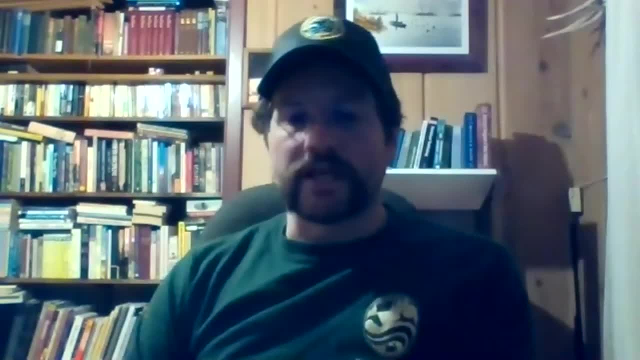 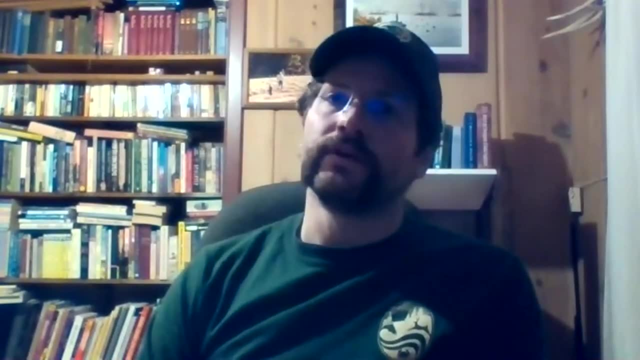 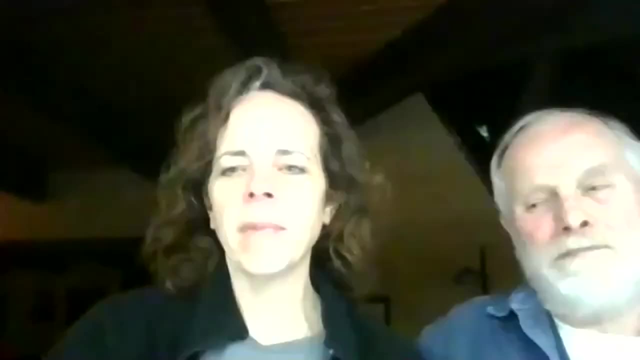 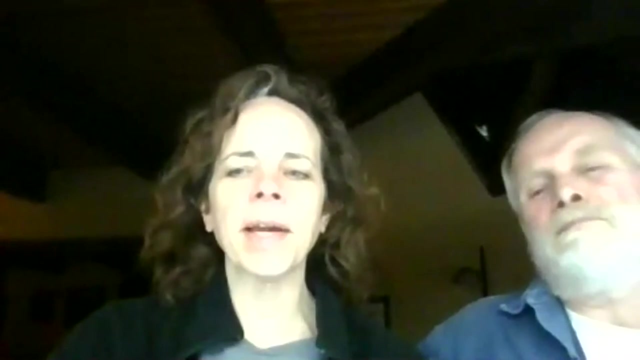 and creating forage for elk, even if herbicides are applied post-harvest. so I hope that makes sense. Okay, and it looks like we might have just one last question here, and it's from Rick. he wants to know whether blackberries are palatable at all for the elk, and he's thanking.